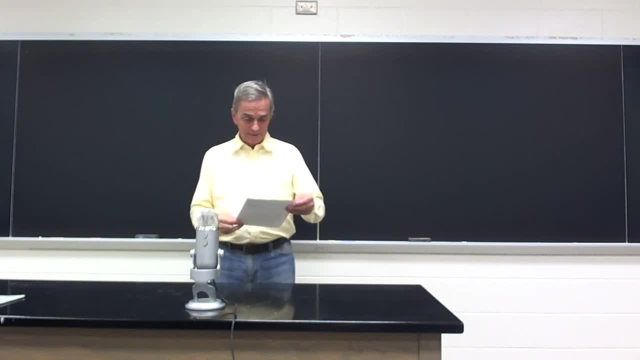 And we wrote our first diagram And today we'll actually try to evaluate the vertex correction to electromagnetic moment. At least we'll get started on doing this. In balance, that's called G minus 2. So G is what magnetic moment actually is. 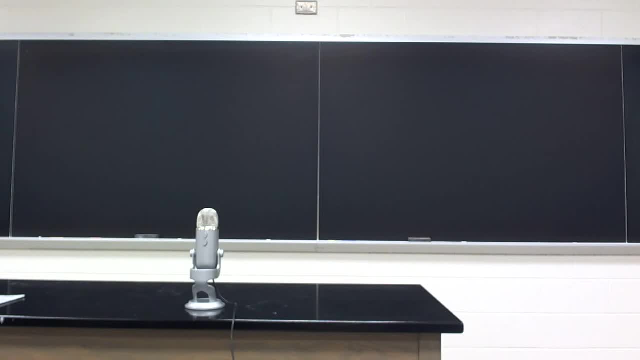 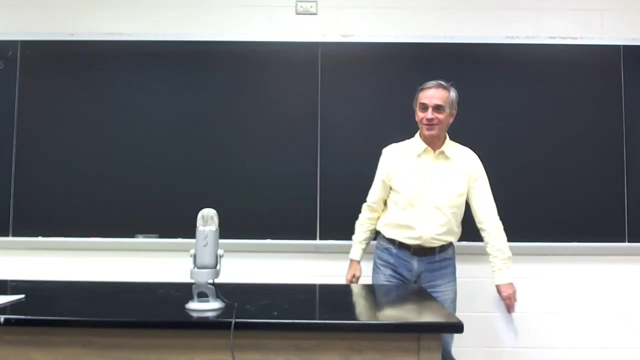 And 2 is what Delac says it should be, So that's anomalous. So this is not anomalous, But it seemed anomalous experimentally when I was first measuring Magnetic moment, Magnetic moment In flash of brilliance. I aimed the camera only at the first middle two sections. 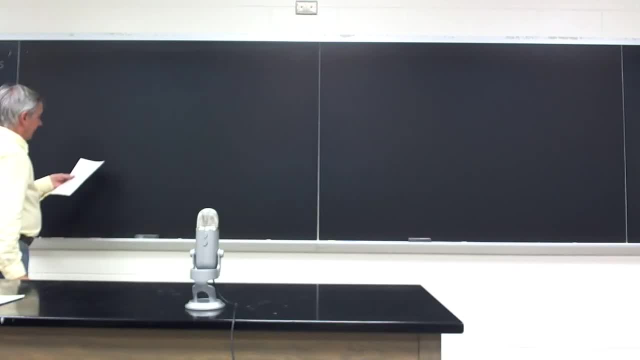 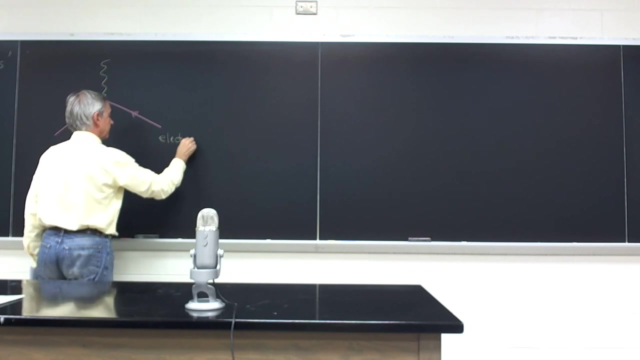 So this is off-camera. So the diagram is: here comes an electron, She has mass and she has spin, and here comes the photon. electron in and out. And the first correction is: electron emits a photon, a virtual photon, which is allowed. 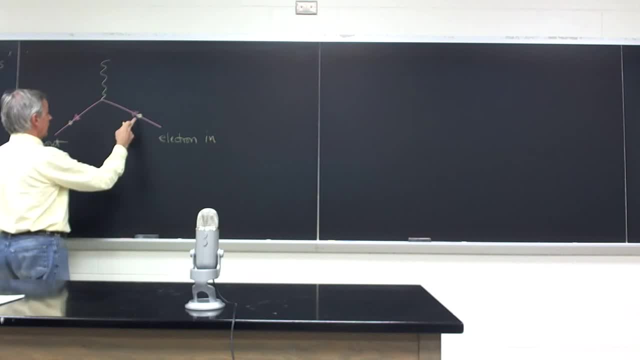 by quantum mechanics not allowed classically, And while the electron and photon coexist, both of them now are of the mass shell. the electron scatters off a weak magnetic field, which we discussed last time, and recombines or reabsorbs the photon. 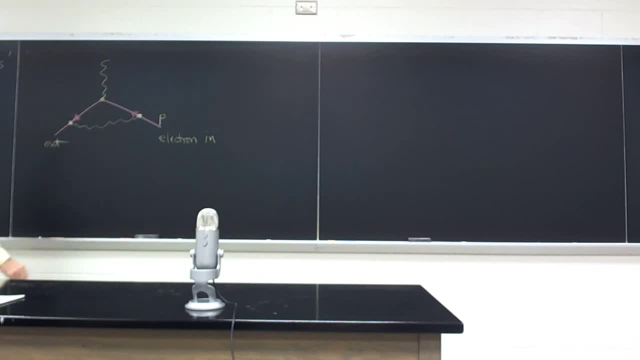 So, coming in, there is a momentum on mass shell momentum. coming out, there is a momentum on mass shell momentum, okay. And then there is photon or external classical magnetic field picks up the difference and we'll be interested in the limit when this difference goes to zero. that's a physical 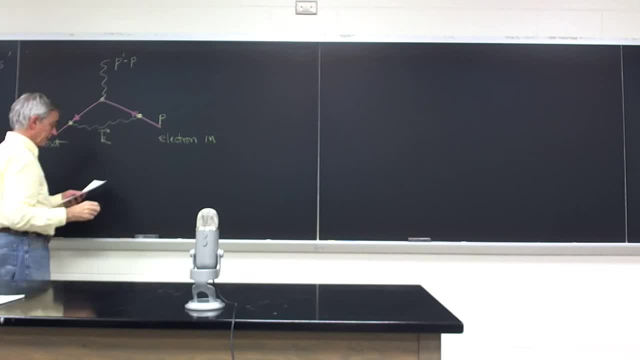 measurement of anomalous moment of electron, And that is a T minus K momentum going this way. Okay, And then there is a, And then there is a Going this way. So is this a scattering? Yeah, this is a scattering in the. this is the scattering in the. But the matter is, it is not seen as a sort of one, but it's seen, as you know, a kind of visible, you know, machine, very sensitive, invisible, and it's a very, very subtle, very subtle. 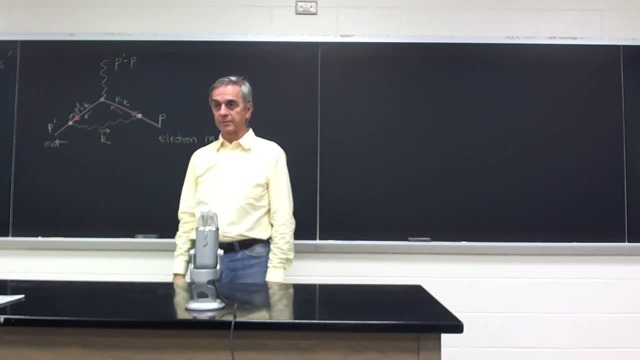 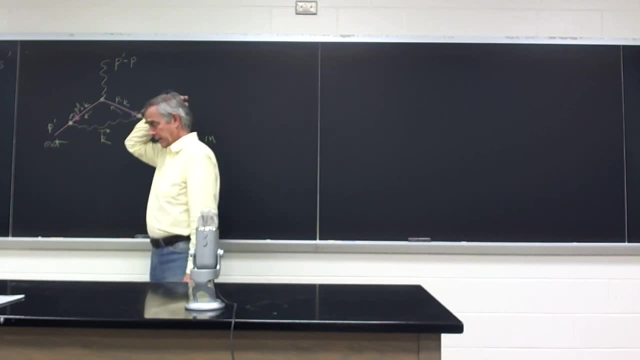 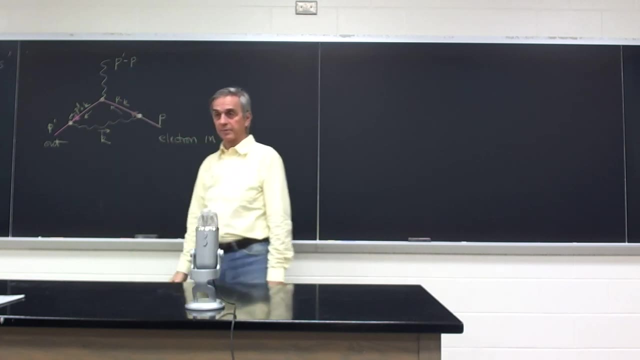 Yeah, with a small magnetic field, classical magnetic field. I mean this is true for any scattering process of electrons. Usually, you know, when you think of scattering, you think that there's another particle, for example a nucleus, and you compute some scattering cross-section. 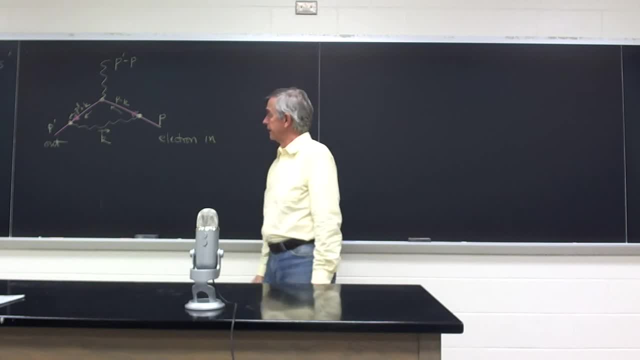 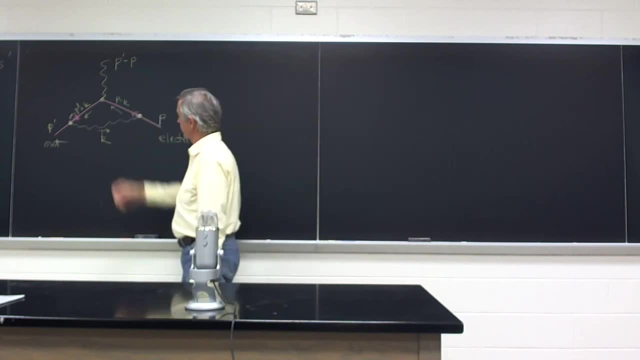 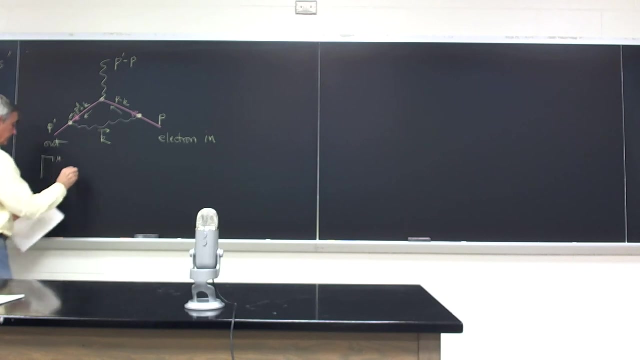 This is just a correction to spinning electron moving in a weak magnetic moment. So you know, last time we discussed the form of classical magnetic field and vector potential that encodes it And we wrote the diagram in the Feynman gate. So there was E squared for the two, two couplings here. 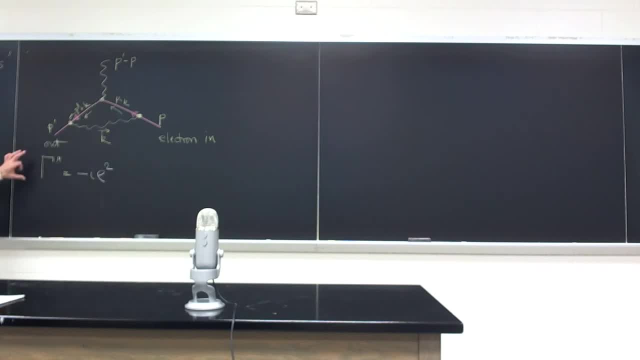 And this E is absorbed into the definition of the vertex. You know, I can multiply this E on the side, and then I will have three powers, or these very important ones that have to do with the virtual photon, And this is most conveniently computed in the momentum space. 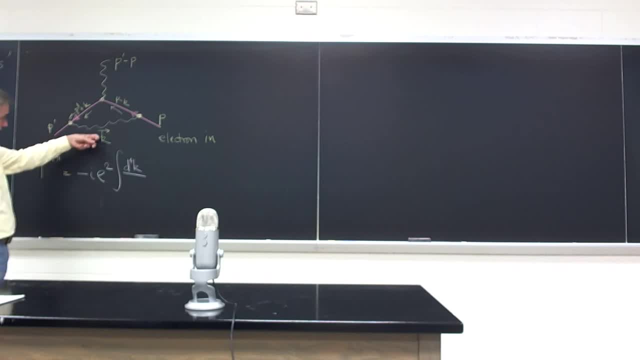 And the only thing that varies is the momentum of the photon. There is one internal degree of freedom that has to be summed over And I'll break it up. So here I have this following Z. You know I looked at actually my first three papers. 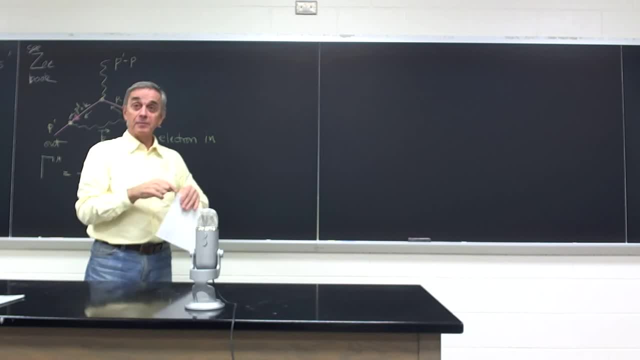 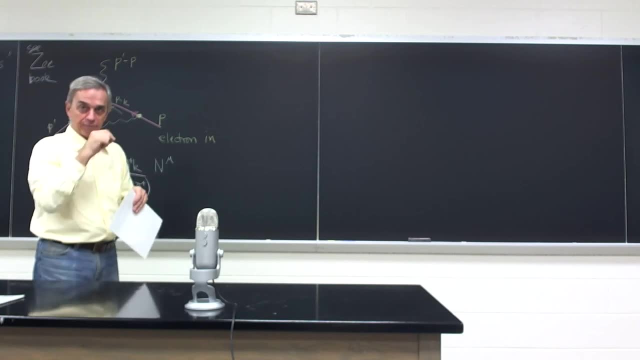 which were on the subject and it's extremely sophisticated. So I it's so sophisticated. it's very hard to explain One loop correction, because I computed three loop corrections, But it's not worth your time to do it in an amazingly elegant way. 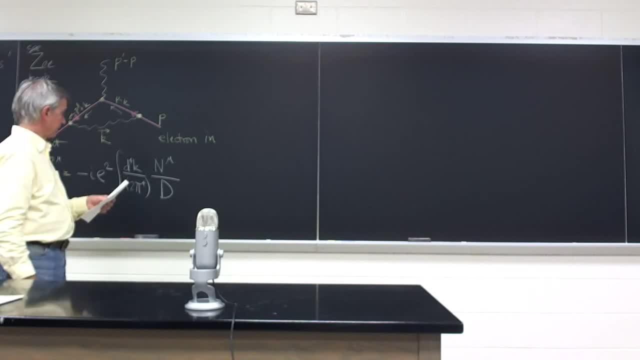 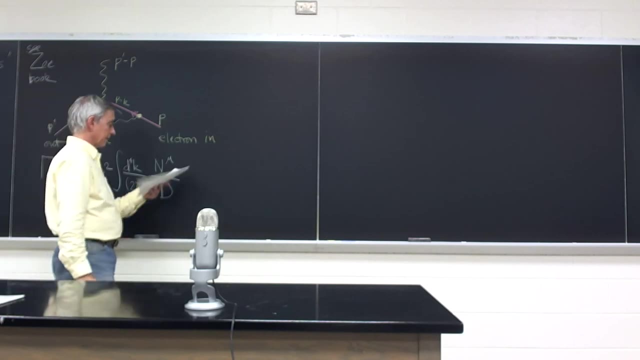 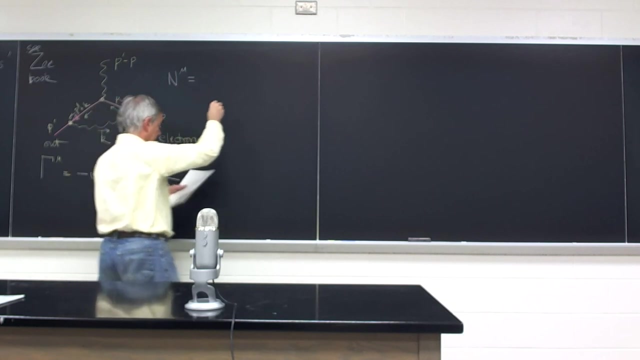 that I did it as a graduate student, so we'll do it in a pedestrian way. So there's a numerator and denominator. Numerator is a four vector because the vertex here is a photon carriage, Minkowski index. So the numerator has got a mu from here. 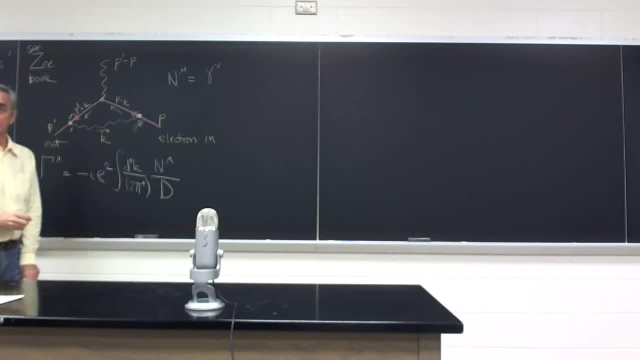 Is. is the fourth color? the outside? Inside or outside? Thanks, Uh Yeah, The. the internal photon up here is contributing uh plus k to the um electron on the right right. Yeah, And it's minus here. 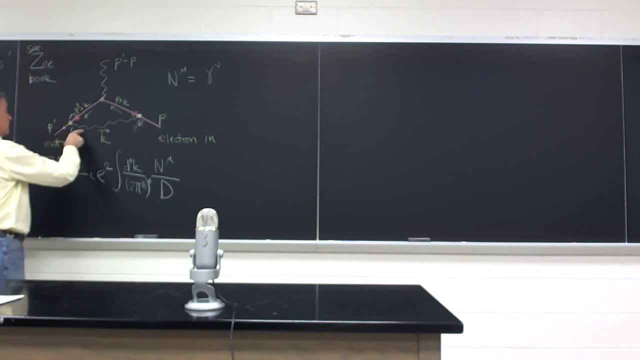 Because it's metric, These two guys. Yeah, this is correct. right, It matters that the output, Then it should be On the left and it's antiquated over. so, oh, it's No, it is okay. 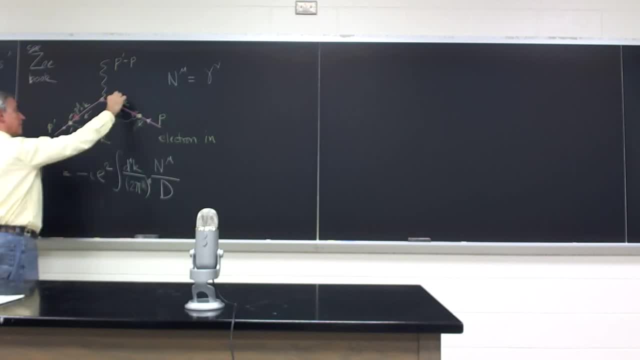 I mean they, they add up. So this two guys are up to that And these are coming out, So they add up to that. So I think it's correct. So there is this photon vertex. you know, the electron couple is: 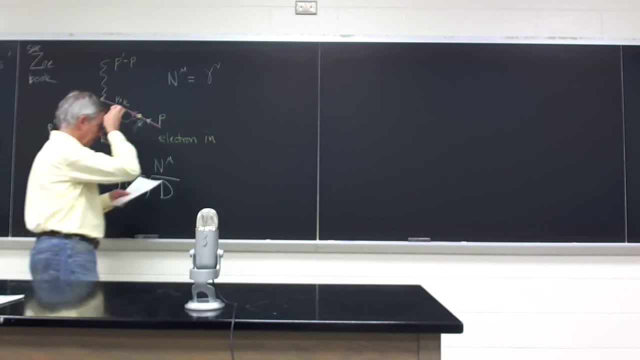 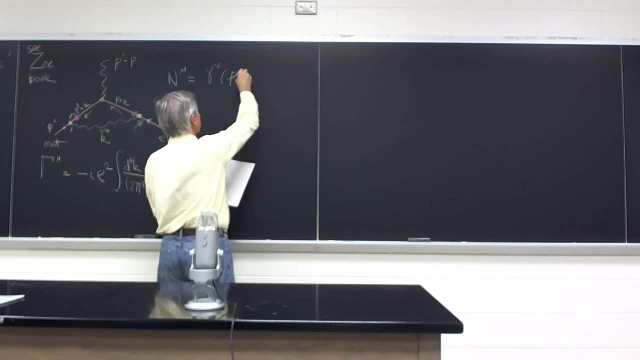 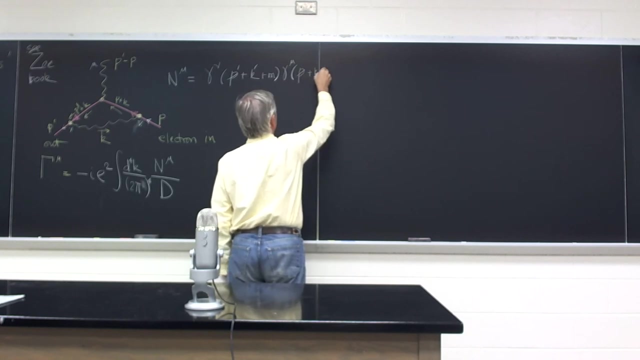 these are here. Then there is a propagator, to the part of the electron propagator, which is plus three. Then there's external vertex, which we'll say is blue- This is the Dirac field- and then there's p plus three. 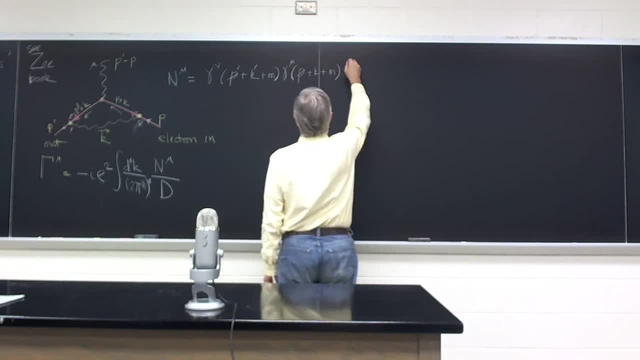 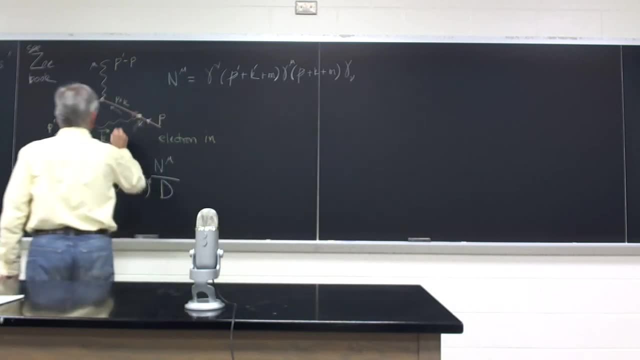 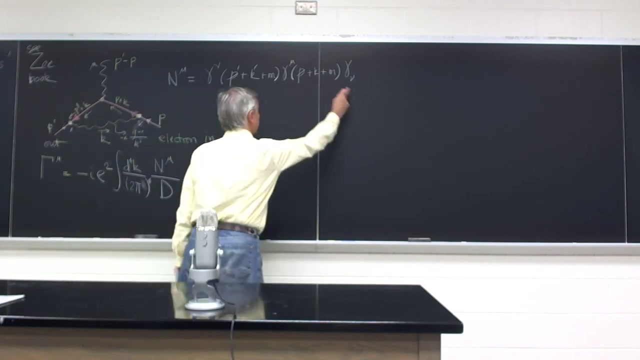 plus n. and then there is g mu, because in the Feynman gauge we had a g mu mu over k square Minus. So this numerator only has a Minkowski metric, which we have used here. So this is a numerator. 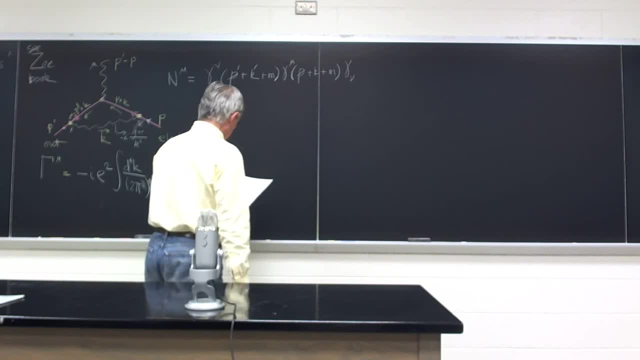 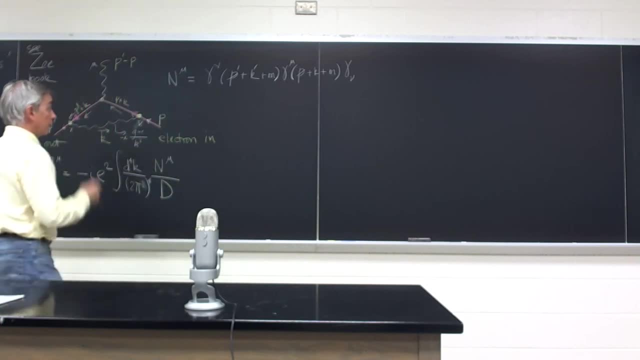 And if there is a mu over the denominator, then we've got something called the momentum of a doublet. And then there's a p minus three plus t, which is p times n plus three. That's a negativeっ minus two. Then this is a denominator. 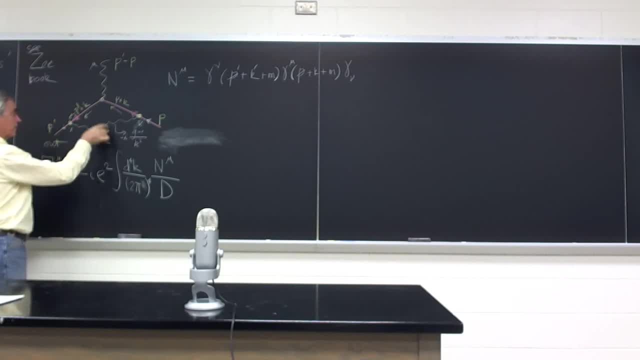 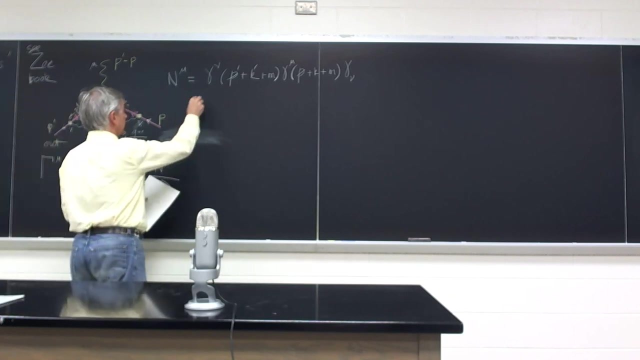 and then there's a global groups, barely Okay. There's a power n here, Yes Okay. of photon propagator. there will be sort of Klein-Gordon propagator part, the Dirac and Klein-Gordon part. So you'll have form of having three factors. And now what you have. 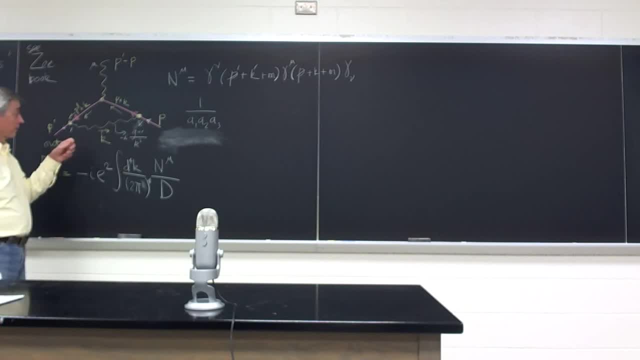 to notice. these factors are quadratic in k because they're all k squared etc. And they're integrating our k squared. Now if we could convert this into a Gaussian, we would be in heaven, because we know how to evaluate Gaussians. that's about the only. 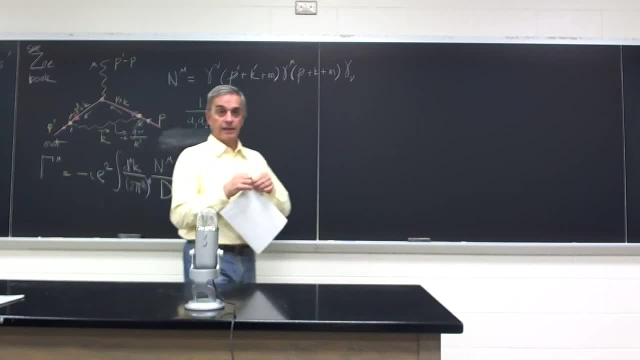 thing, And if you look at the links in the course, I've given you a link to a popular lecture by Witten- which was actually quite technical but you know totally on the level of this class- in which he explains what Feynman diagrams are, And he has a nice 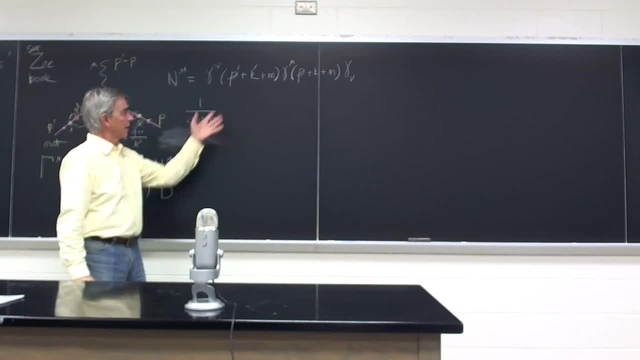 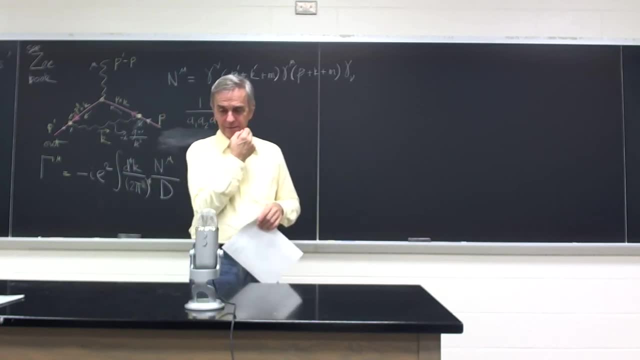 introduction to it and he has a nice introduction to it and he has a nice introduction to this interpretation. So promoting this into a Gaussian is called Schwinger trick or something. But Witten has a nice interpretation of that trick once you get up in the Gaussian. 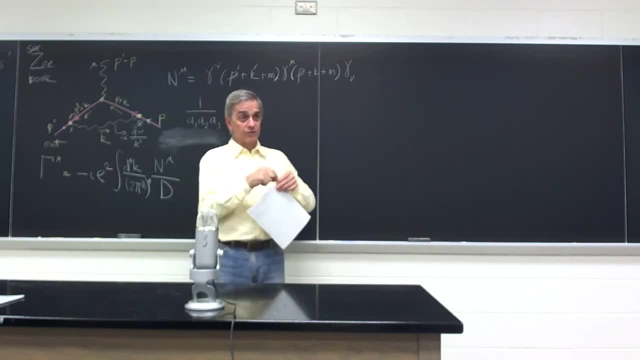 and he really starts explaining that this very much looks like the integration, you know, the path integrals that we've done before and that there is a proper time. in this You interpret the Laplace transformation you did to make it Gaussian at the proper time and 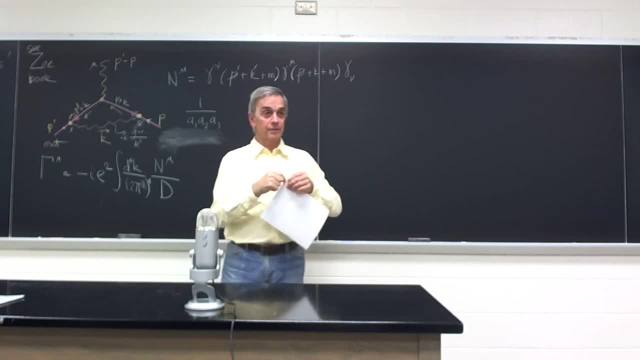 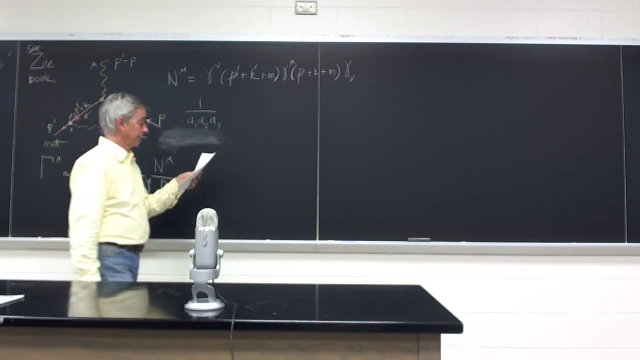 it's very good. And that's his trick to get you into the string theory, because then you say: well, if it's not a particle but it's a loop, blah, blah, blah, But it's very nice, I like the interpretation. At this point I'll just state it as an identity which 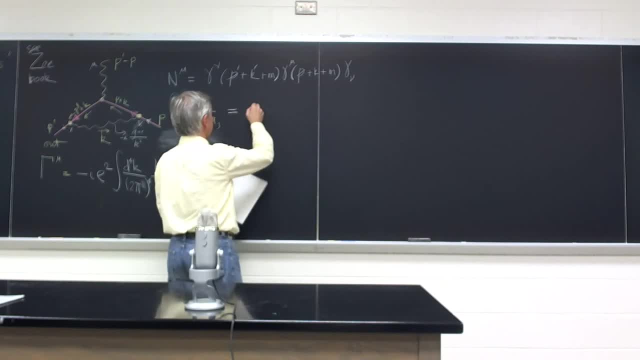 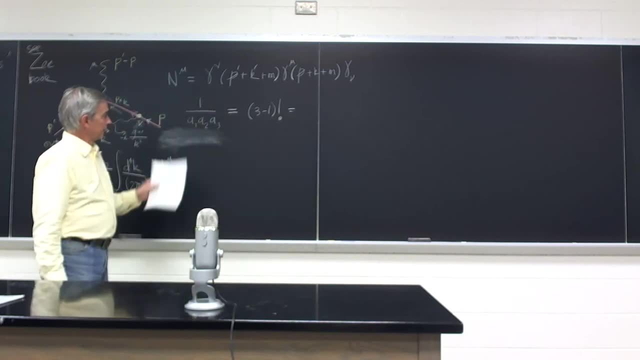 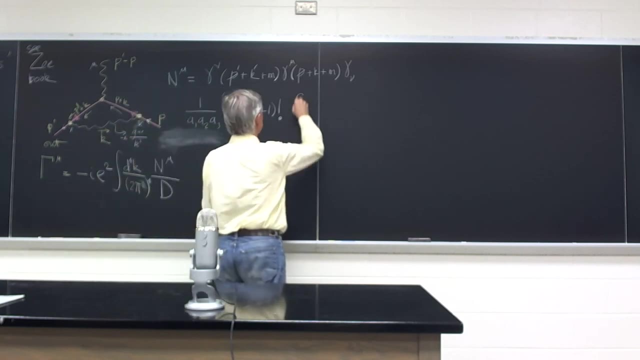 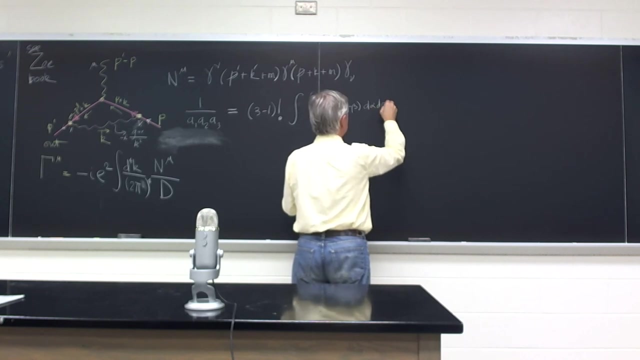 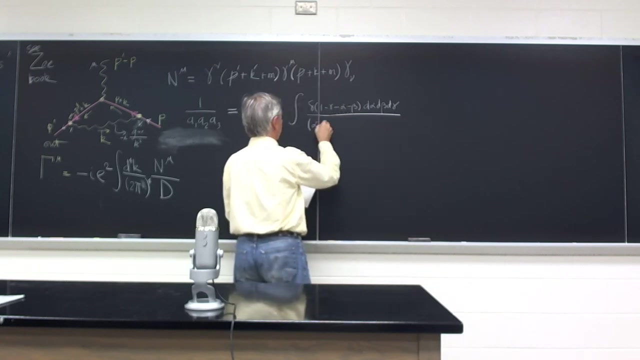 I guess I'll give spirit to as a problem. So whenever you have a product of this kind, you can write it as an integral. It works like this. So that's just an identity and it's very good. Thank you. 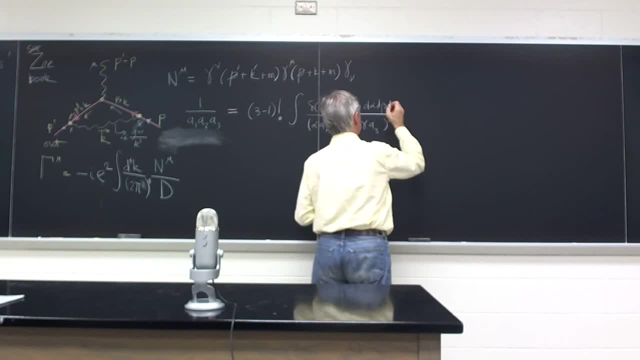 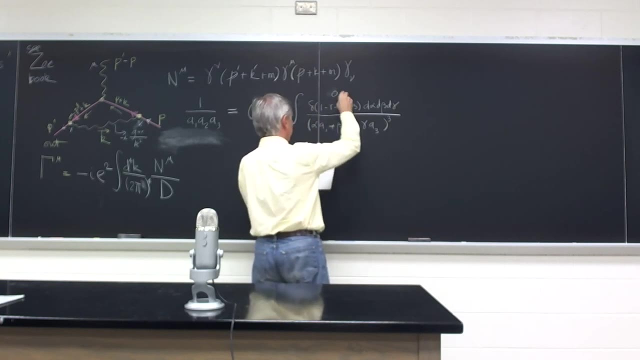 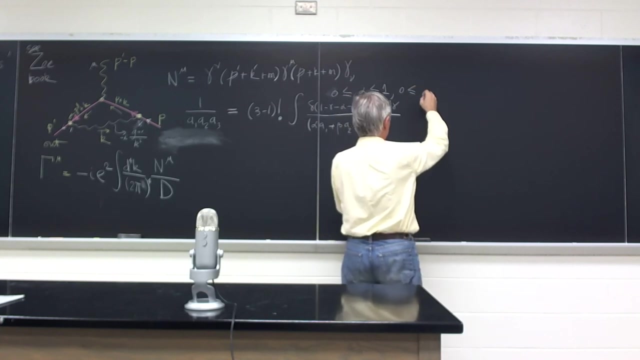 Thank you very much. Well, these things actually have to be ordered. so the zero runs from alpha and beta runs from one minus alpha, And then you have to do the same thing over and over and over again, And then you have to do the same thing over and over and over again, And then you have. 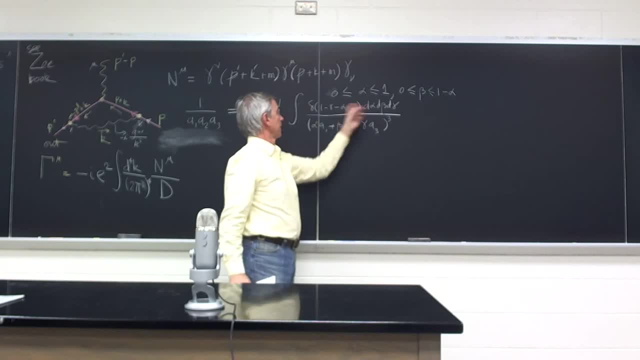 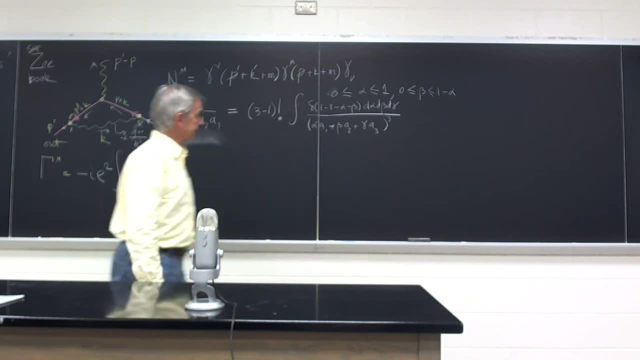 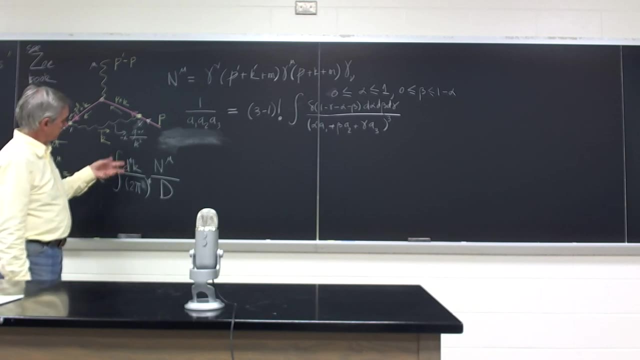 to do the same thing over and over again. And gamma you can get rid of by just doing one integration, because you have one delta function to integrate and so that's an uninteresting identity. But it's extremely helpful because you started with something that was momentum or space, etcetera, and you are able to bring it to. 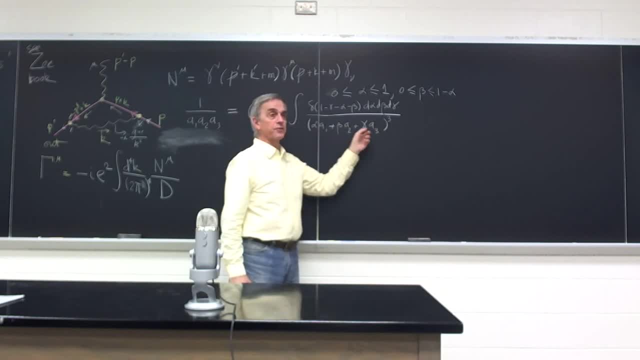 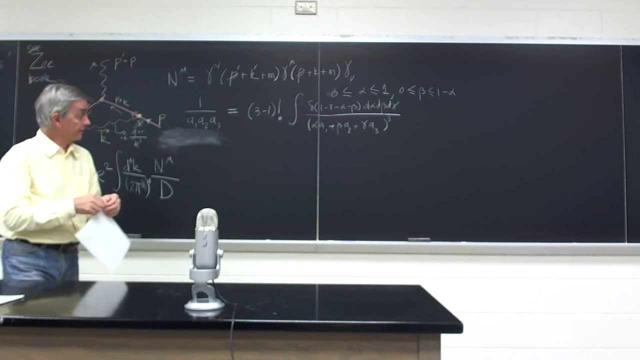 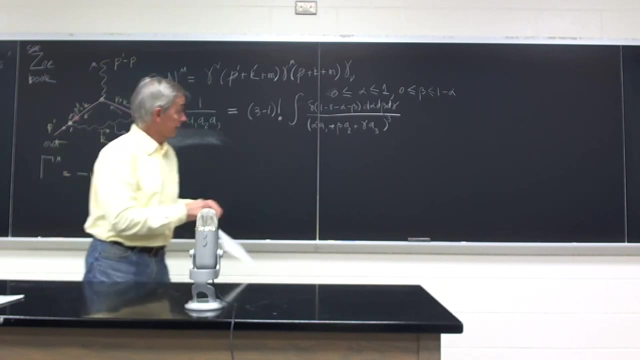 a form where you have something over a momentous square, some quadratic form, so it just lasts. Yeah, exactly, Thank you for our questions. And these kind of things we can integrate And in the way that's done by Schwinger and that's done in the, for example, article that. 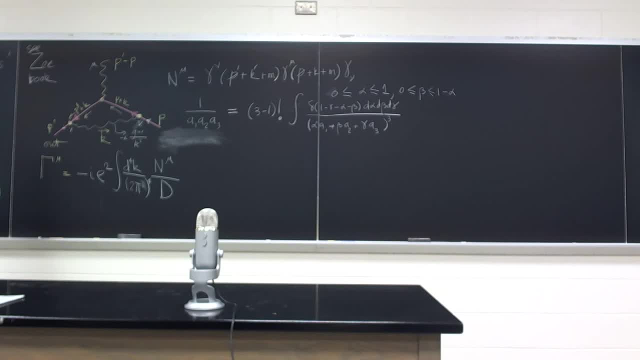 I've written with my advisor. I guess I should tell you about my advisor. So Toichiro Kinoshita survived the firebombing of Tokyo, so this was one of the great achievements of the Second World War. It was a carpet bomb run by Curtis LeMay, the famous general from the Vietnam War, and 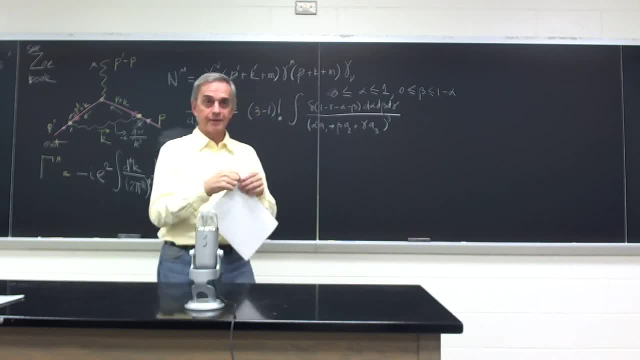 it burned the Tokyo down. It was much more deadly than Hiroshima and Nagasaki, but Tom survived it and came to the United States and he became a legend as a member of the National Academy of Sciences. because the man doesn't know, He doesn't know how to make errors. 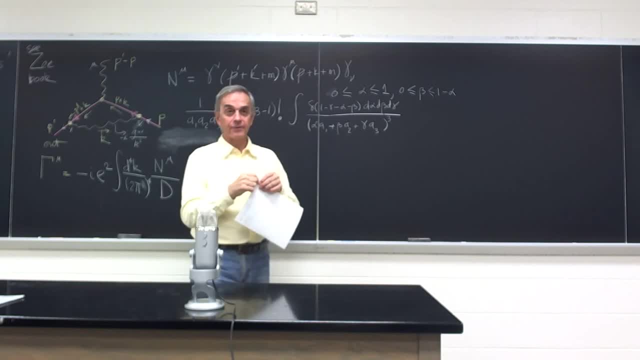 So it's totally scary. You know, I worked with him for a number of years and I've made some errors in our calculations- Not Tom, He never makes them And this kind of calculations get very hard. I mean, there are thousands of diagrams and you have to work for years to do it. 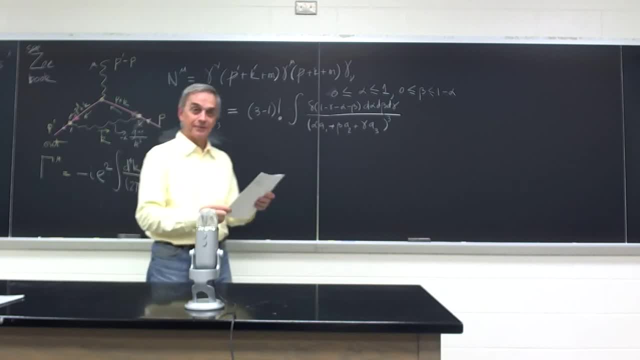 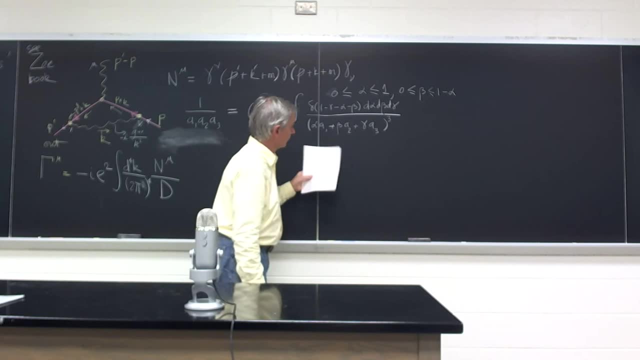 So you know, Tom Kinoshita is made out of different stuff than the rest of us. a very impressive man, And you know he's a great man. Thank you, You know, we have a much more elegant way of computing this in general, which is related. 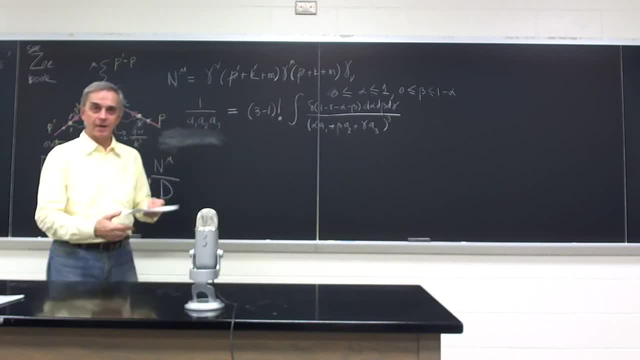 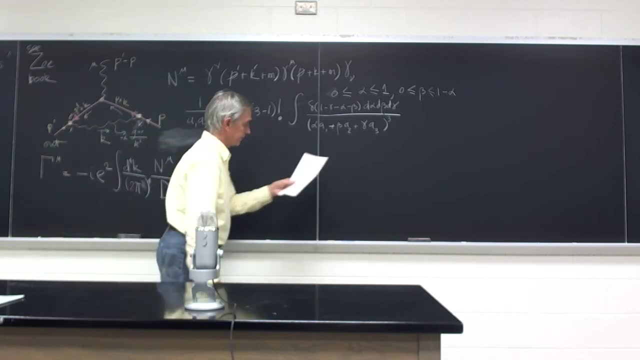 to graph theory and Kirchhoff currents and graphs et cetera. but that would take weeks to explain, so it's not that time, So we'll just do a pedestrian version here. And so: denominator: blue, blue, green, just the thing that's there, and then you have. 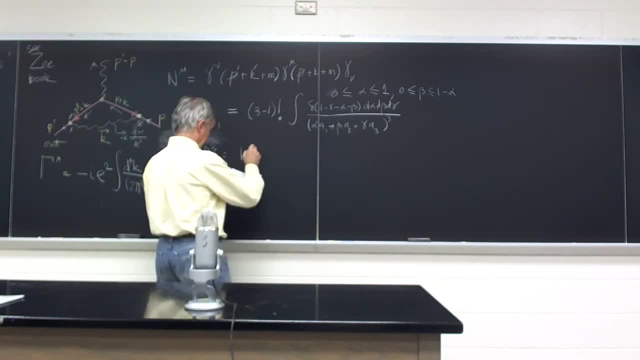 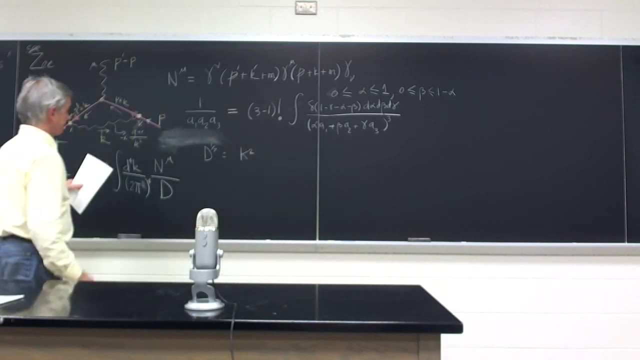 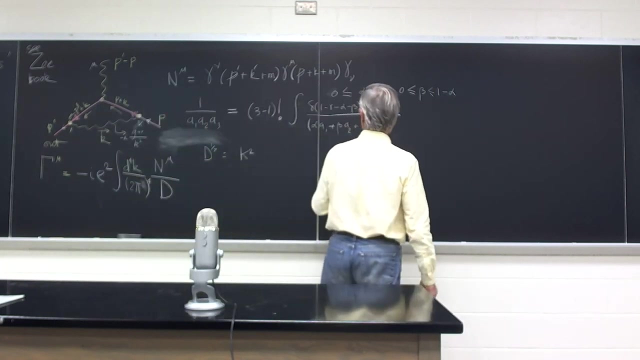 to remember. I need to do this one. I need to remember where You know. once I get rid of the linear, I need to remember you know the linear, you know in the linear. you need to remember where. 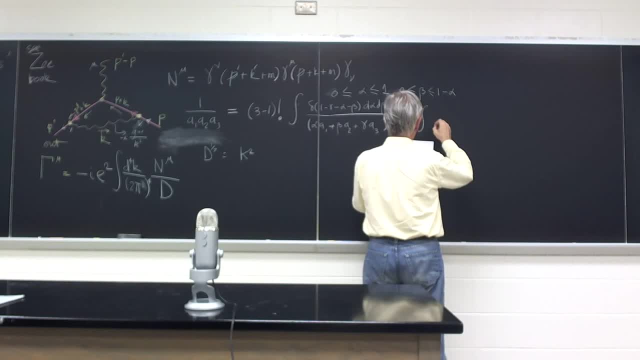 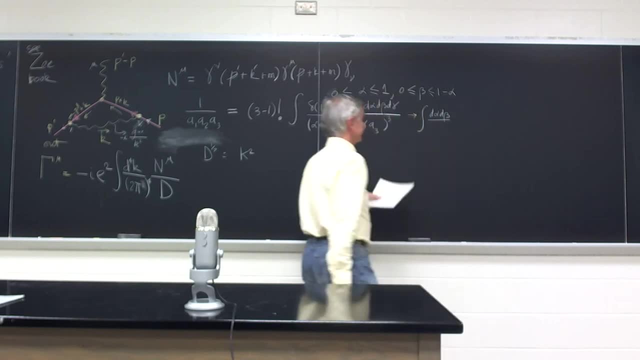 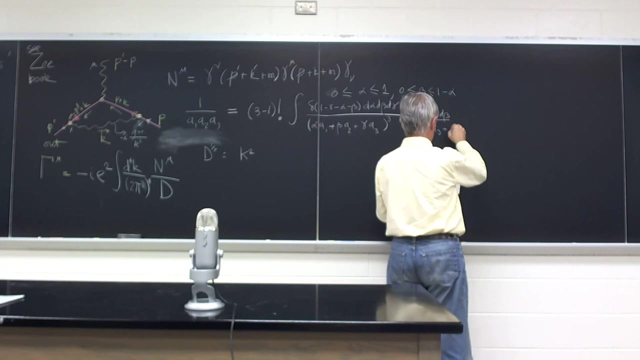 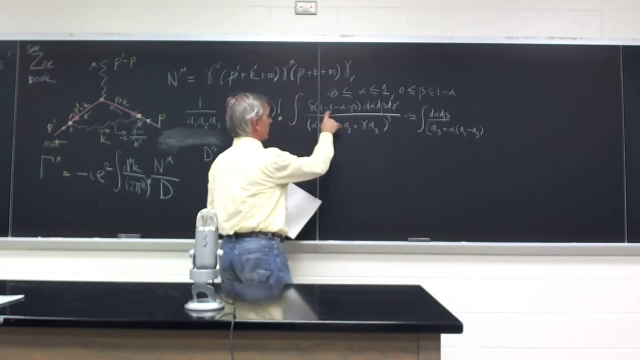 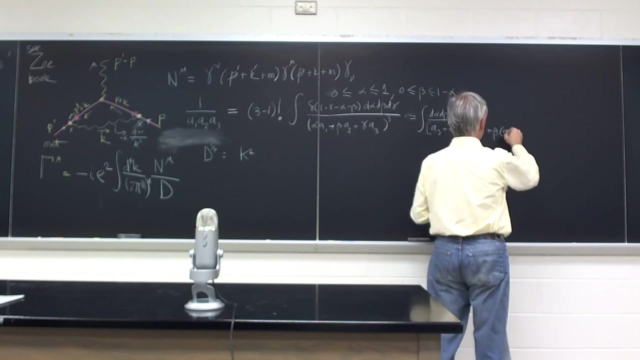 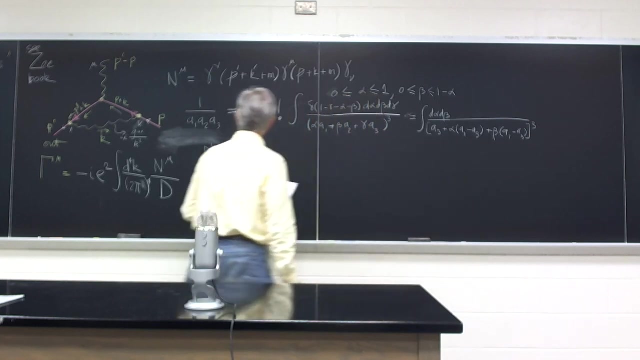 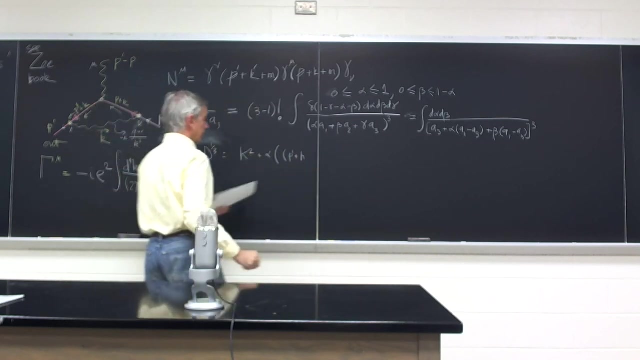 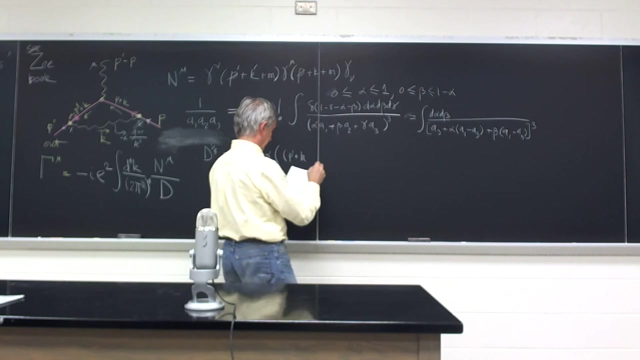 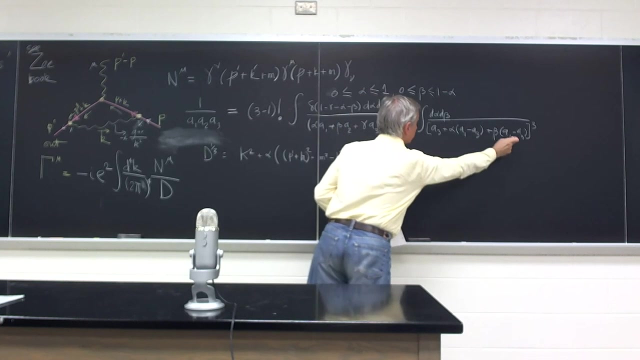 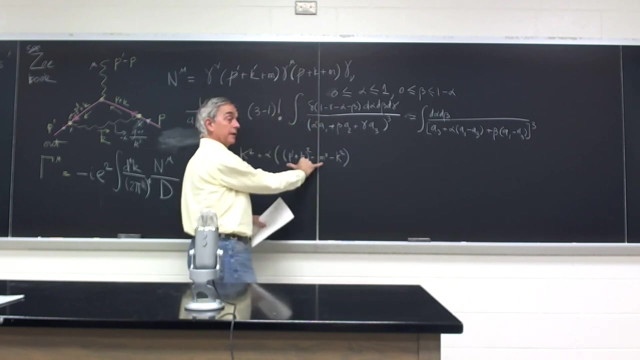 Right, Sorry, gamma calculation into going to play one the place gone by. so what's in here written in terms of k's and p's is the numerator, the denominator of this propagator here. so this case square comes from this replacement here, and this is just the Klein-Gordon kind of. 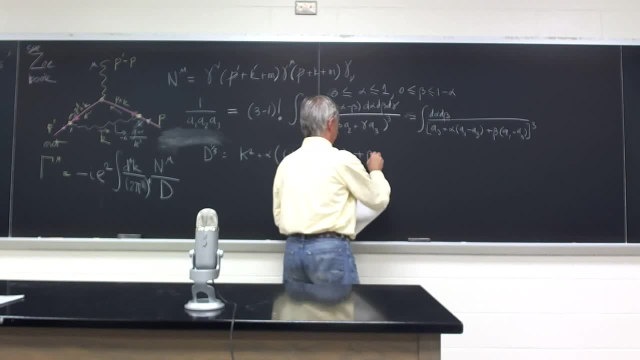 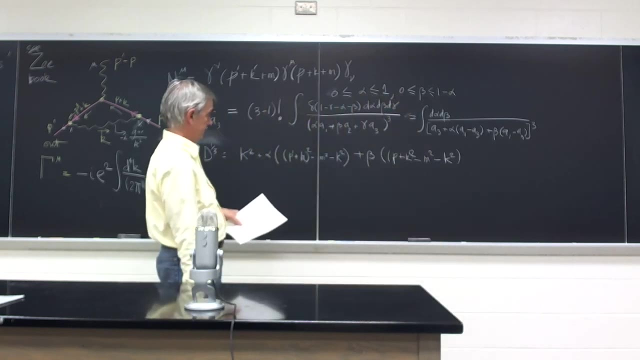 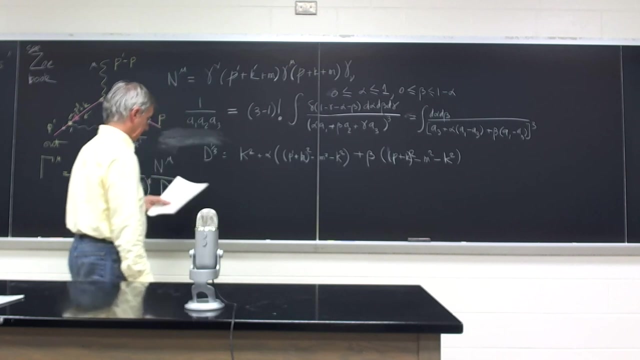 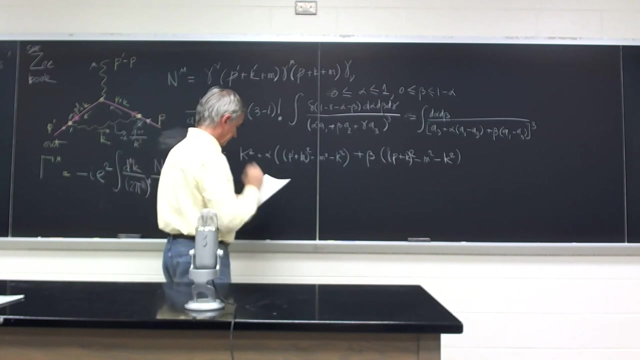 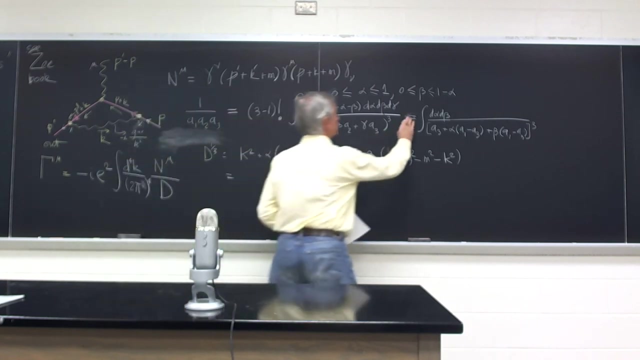 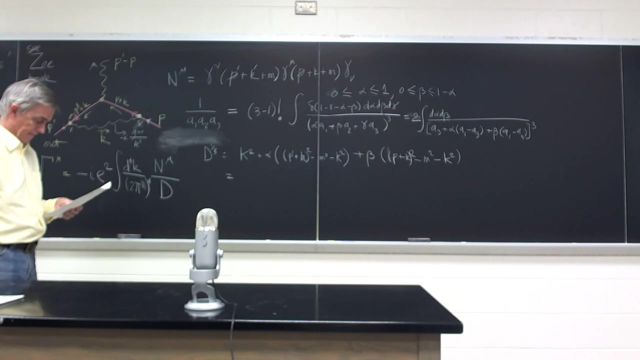 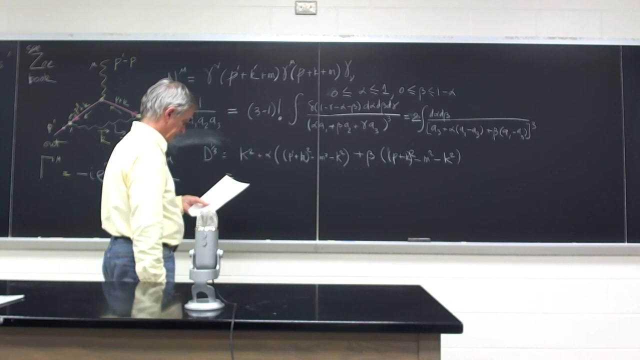 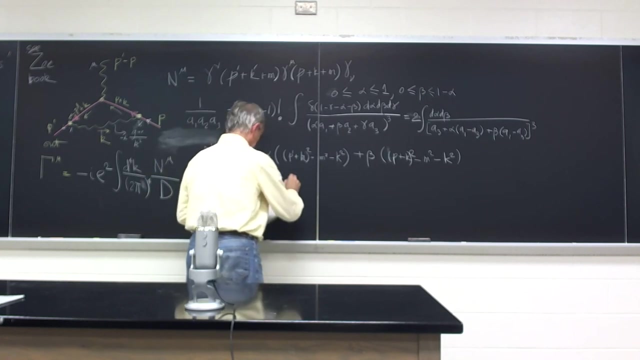 denominator of this propagator. so same thing as case square. and, by the way, what is tools divided by uh two? I need a tool. thank you, pal. it becomes k square plus 2k, and these are four vectors. so this is a four vector dot. 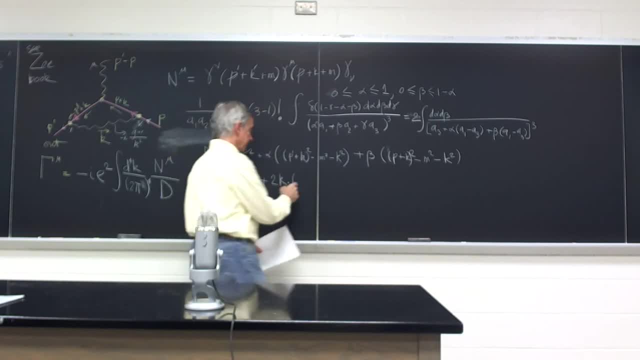 so I don't have to write in this. that's what it means. so let's see. so when you square this, you get a cross term 2k dot p prime, alpha and k square cancels same story here. so that's why alpha and beta don't have k squares. 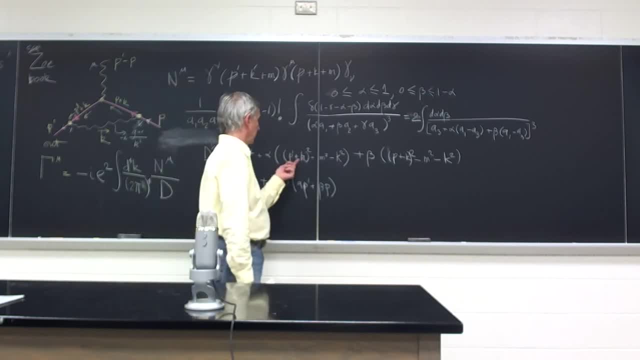 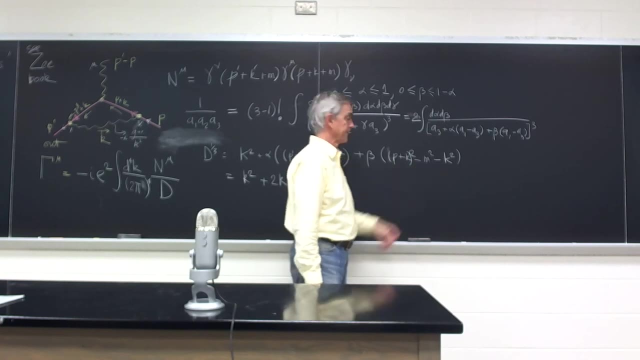 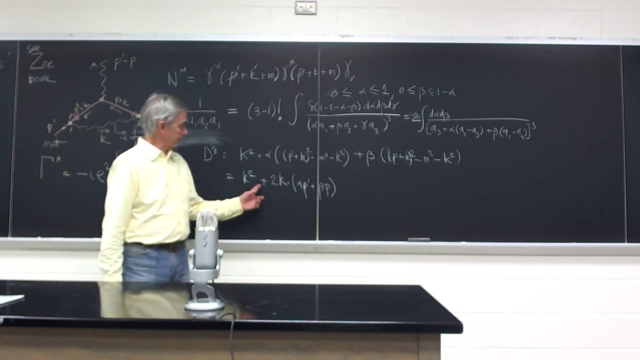 then p, prime square. this is a mass shell momentum, so that cancels this m square. and p square is a mass shell momentum, so that cancels this m square. so you get a very simple expression which you can obviously complete a square of, because it's quadratic in k. 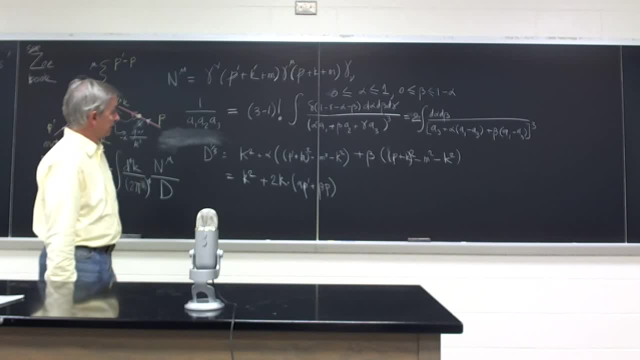 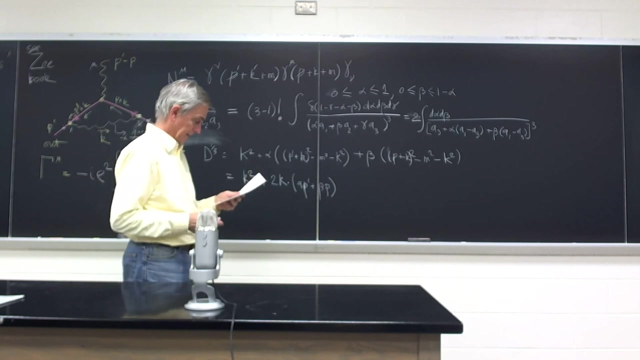 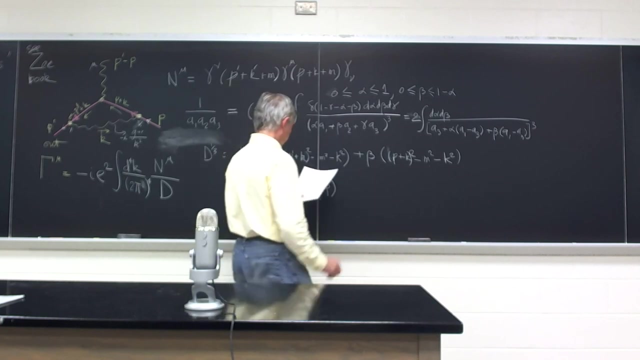 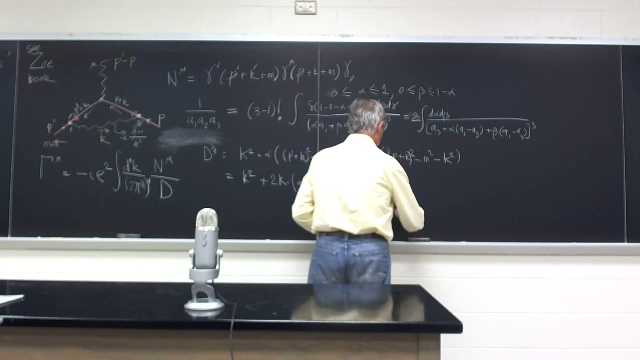 and you will in this integral. uh, uh. you know I still have to do my uh integral over k this integral. I'm just working on the denominator right now, so now I complete the square, that'll be right. l mu will be a mu. is this: is this. 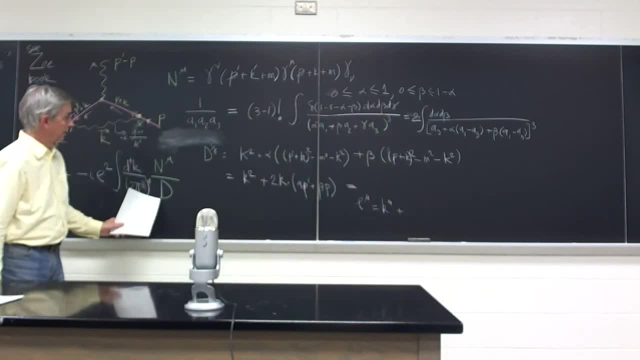 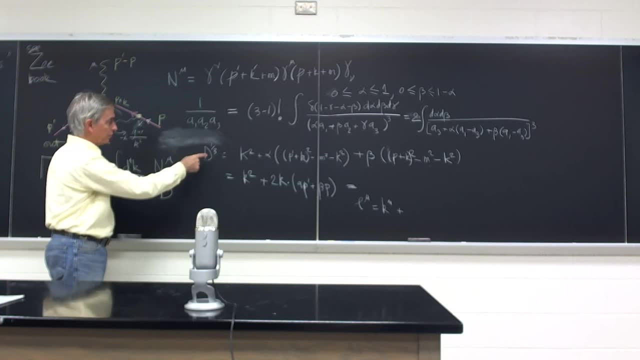 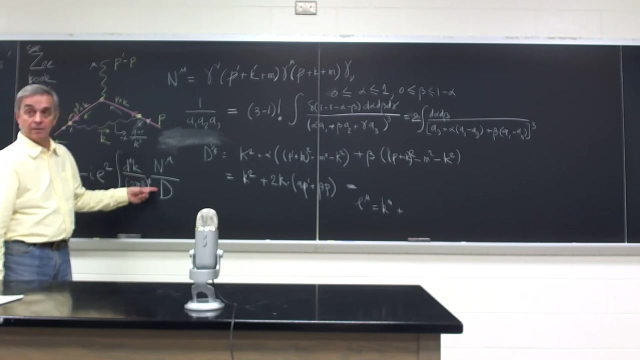 denominator is what we have in the vertex. no, we're not, we're just: this is denominator. now we're just evaluating denominator because it's cube. I'm writing a cube of denominator, so denominator of identity. denominator of identity because not exactly what we. no, I'm, I'm. 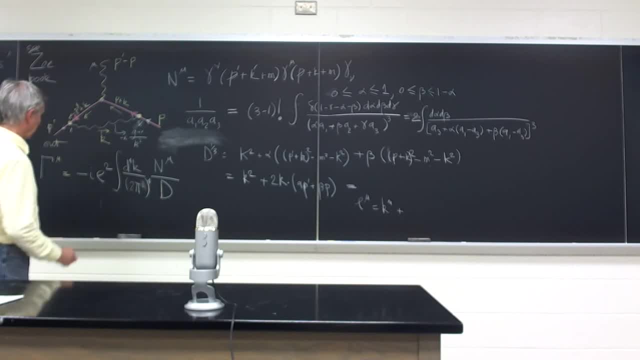 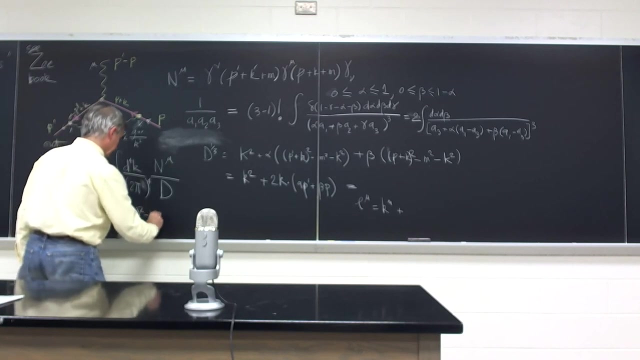 we'll have b you know where. okay, let me write d in in detail, but d is uh, k square from here. okay. well, these uh the three yeah denominators. first, on this: p slash uh plus p k, not slash square. uh minus m, square. the second one. 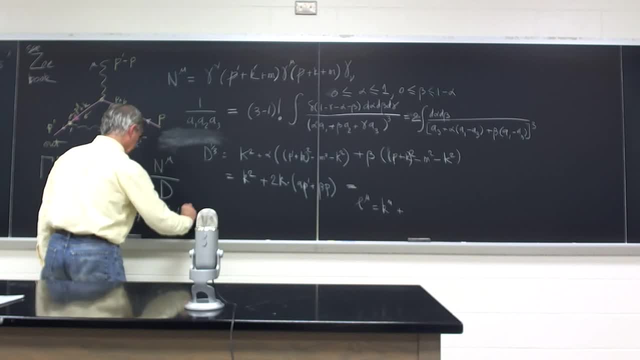 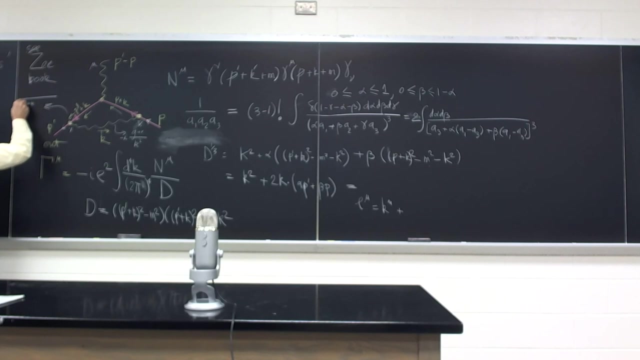 is p plus k square, minus m square, and the photon just gets k square. and here I've used that the denominator, the propagator, has a form, uh, you know, p plus k square, minus m square, plus i, epsilon, and it turns out we won't have to worry. 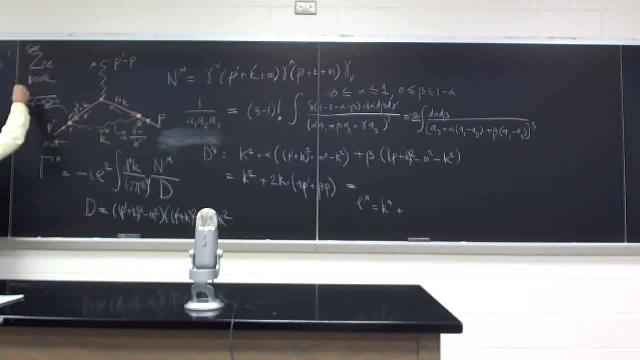 about i epsilon in this calculation, and the way we got it is that we multiply the inverse of the scalar propagator plus. so we get this slashes here. my question is: where are integrations over alpha and beta in this expression you're writing: uh, the identity says: 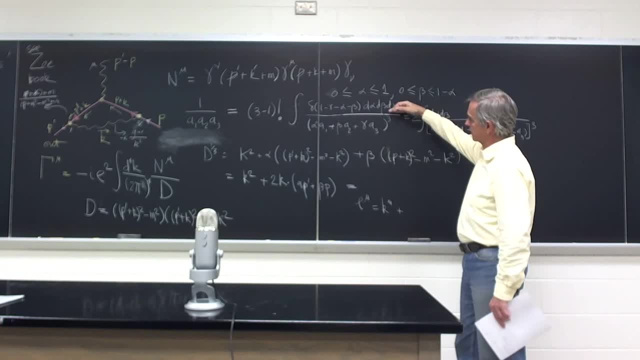 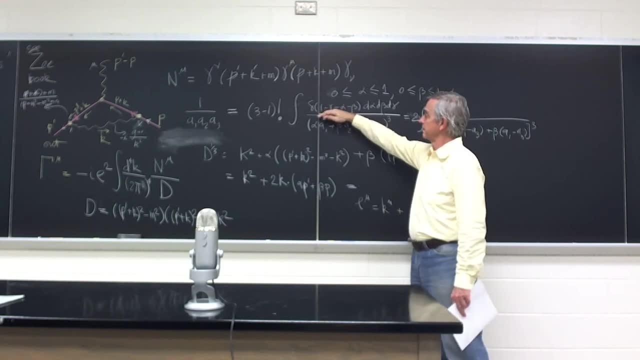 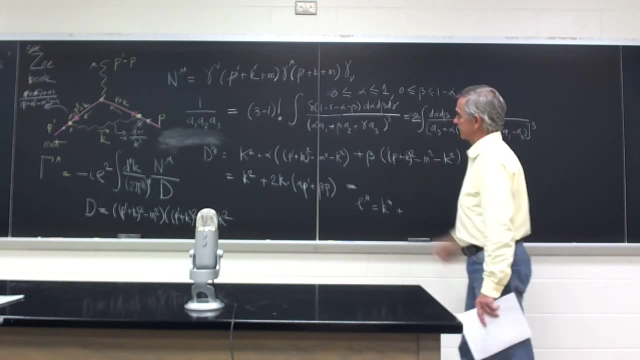 that you can write this as triple integral, totally symmetric, but it satisfies one Dirac delta condition, so I use it to get rid of gamma. so that's how I got there and it has to be in a sort of hyperposoidal area and the one before 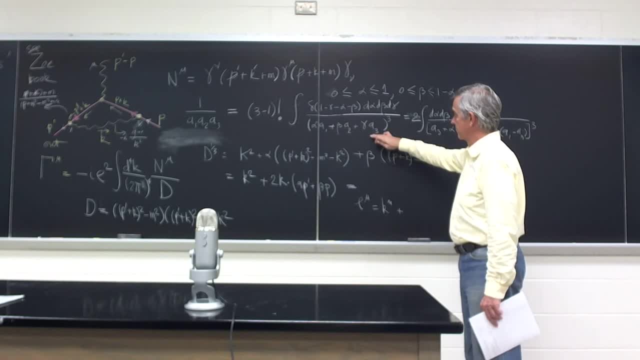 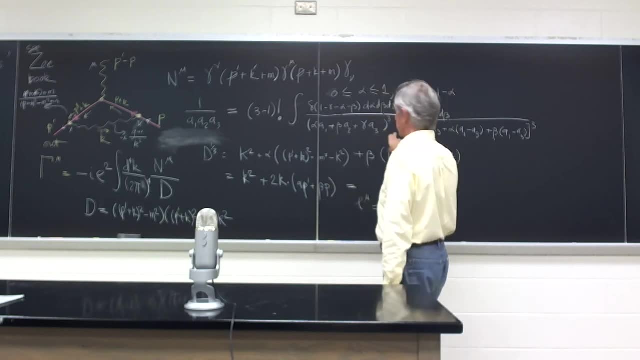 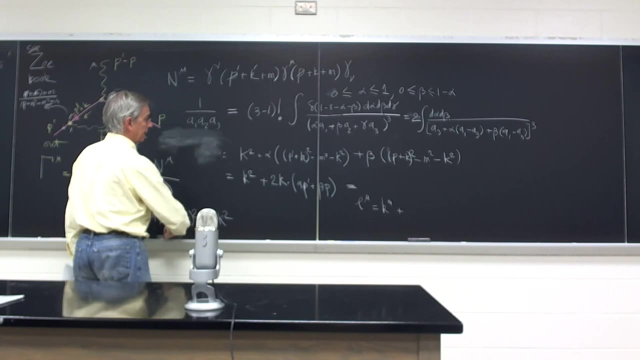 below that d, one d to the one third. yeah, yeah, where are alpha beta integrals? uh, this is just. oh, I see it's just a denominator. no, I'm sorry, it's just a denominator. yeah right, yeah, you're right, the integrals are still there, but 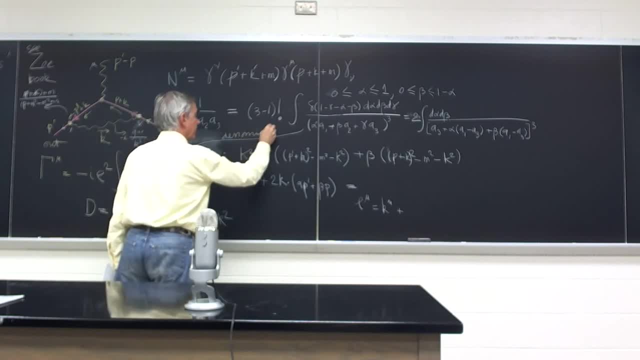 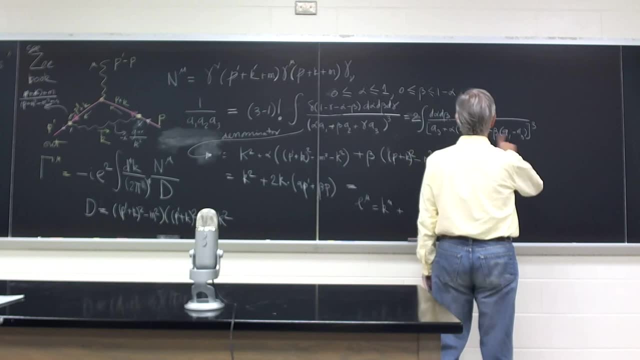 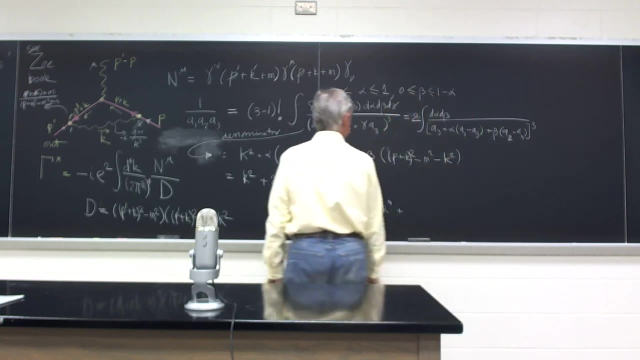 denominator: yeah on beta. uh, what about over there? what about over there? a two minus a three? you haven't heard of a one minus a three, which would be a two over there. absolutely that's enough. so it simplifies. the next thing we do is: we can complete. 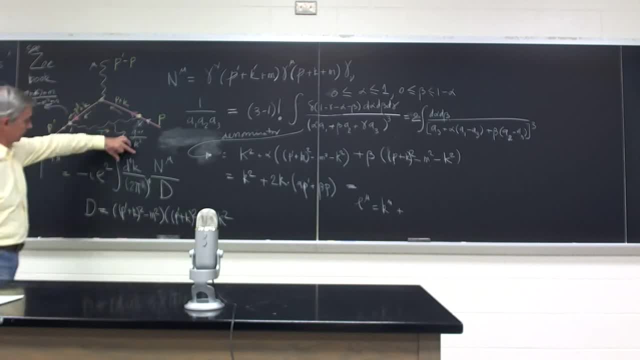 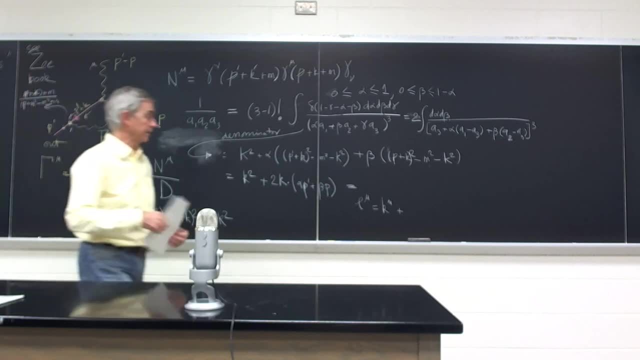 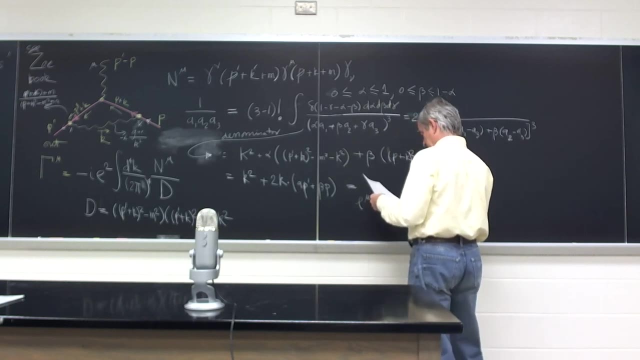 the square, because we'll have the integral here over if order k is from plus to minus infinity. so we're allowed to shift the origin, change the integral. so shifting the origin of the integral by alpha p, prime u plus beta p- u is what we need to complete. 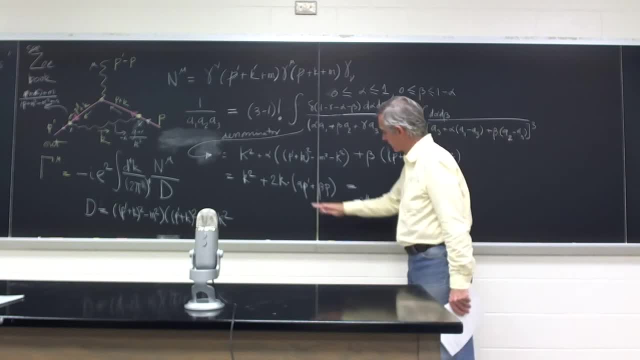 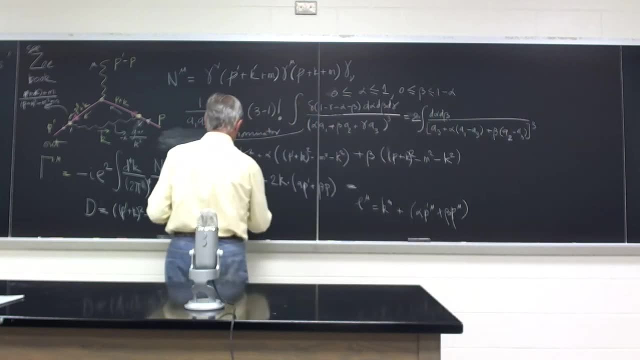 the square. so if we square this quantity in this variable it will be uh uh, four momentum over here. so if it's four momentum, l square plus alpha plus beta square, and every time we square these guys we get m because they're the national m square, so we get. 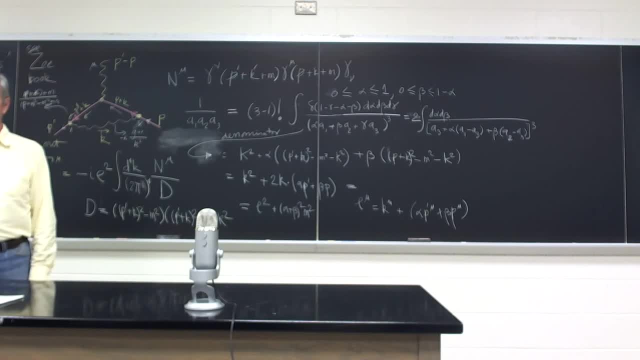 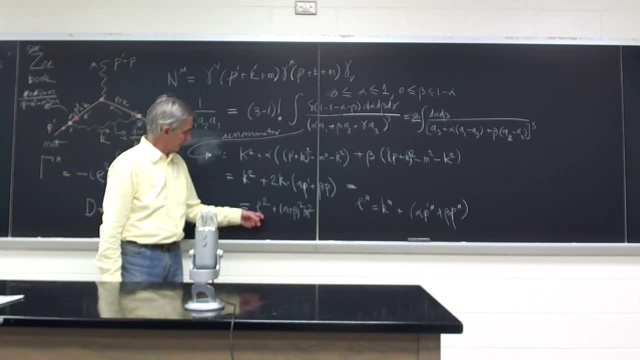 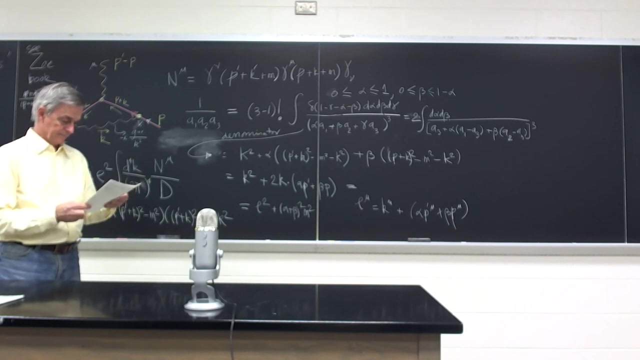 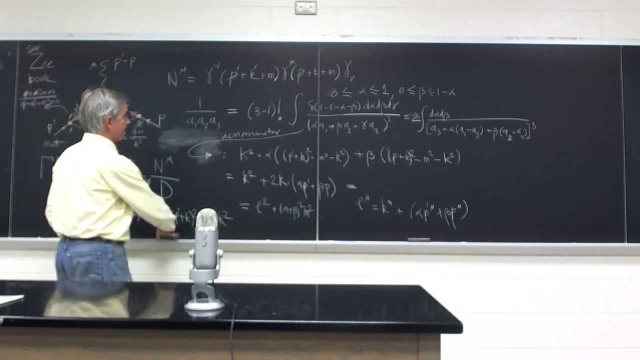 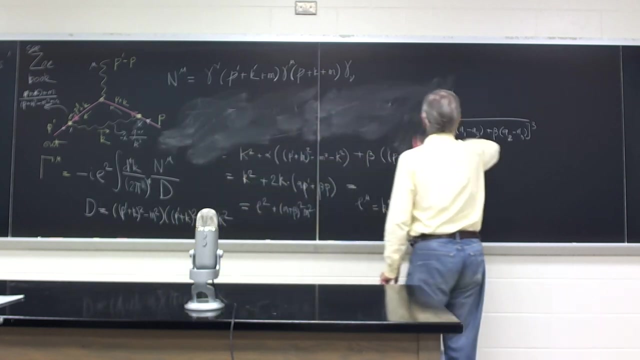 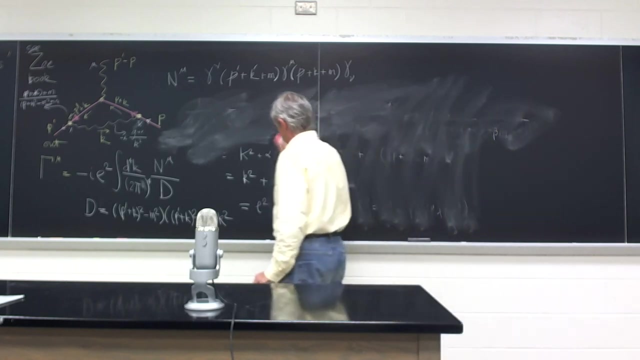 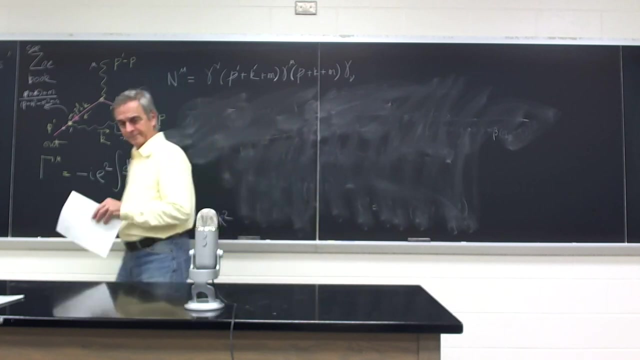 a very simple expression for the numerator of this integral. so what it means is to do the integration over the momentum of the photon in the shifted coordinate. so let's leave this aside and, uh, i will erase this and, uh, focus on denominator, on the numerator, so you. 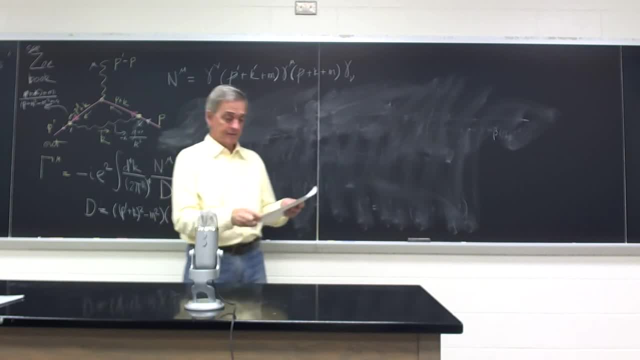 know. after i did this calculation with my advisor i in the career afterwards i had the wonderful opportunity to talk to cn yang, the great uh theorist, quantum field theorist and uh originator of young mill theory and uh. every time i talk to him there'll be. 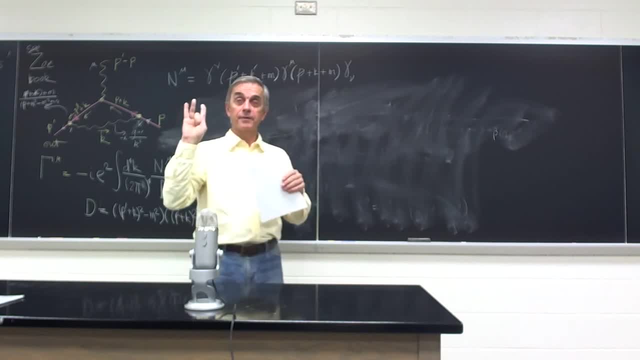 always the same conversation. they have shown young and mills have written two papers, so there's milson, young and youngs and mills and uh. mills and young paper is that they've shown that when you do perturbation theory at the three loop diagram, you know the way. 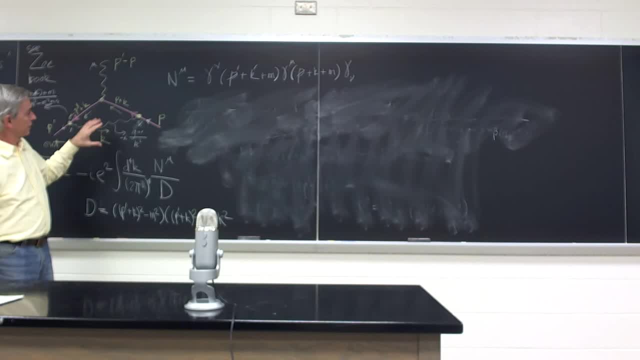 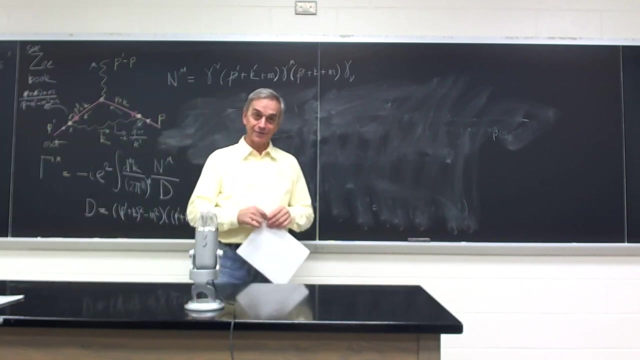 this theory is actually done, if you do calculations is. there is a totally general way of getting rid of momenta and everything is written in terms of this: integrals, alpha, beta, gamma that are run and they only depend on topology of the graph, so it's an ambiguity. 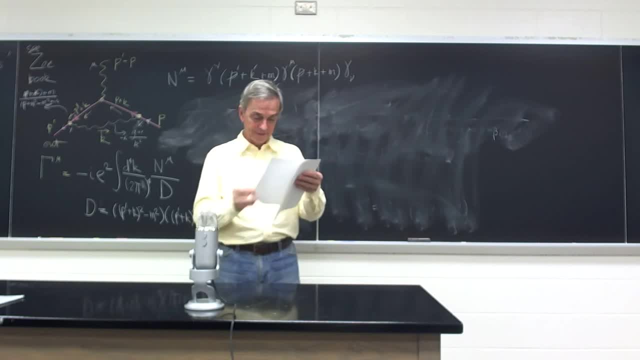 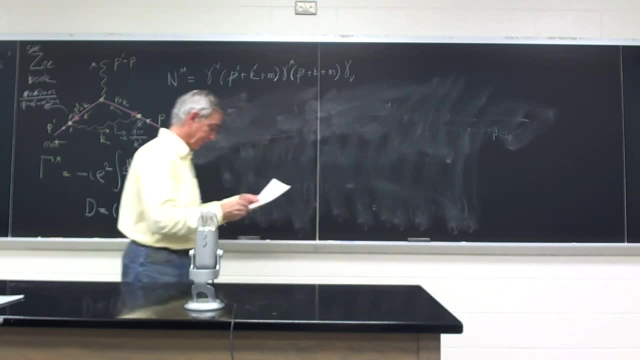 because this diagram we showed in that paper in nineteen, fifty five or something, and there is no ambiguity. the theory is beautiful and it's you know it's a whole new ball game once you start thinking seriously about fireman diagrams, because this serious in france, you know. 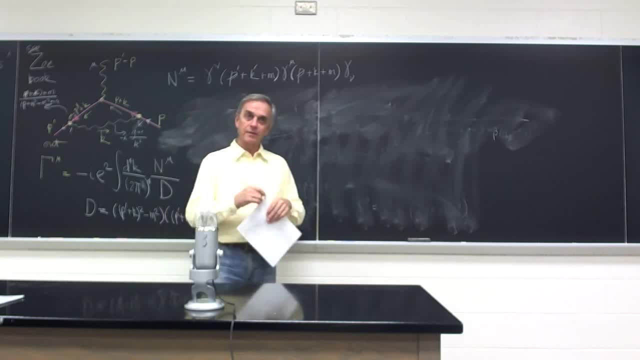 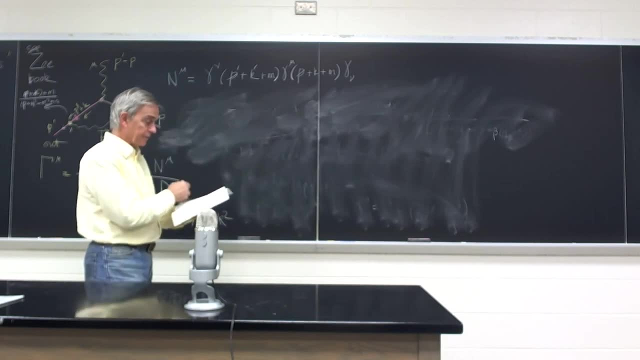 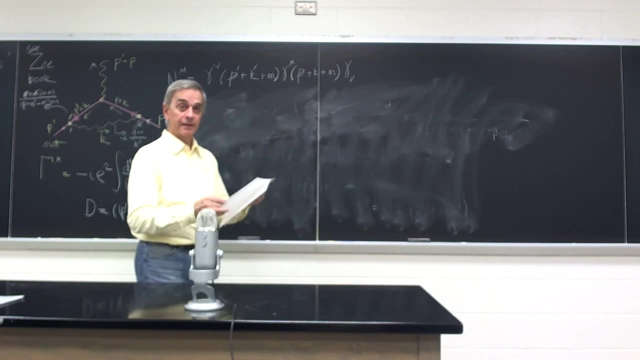 has it for that kind of thing. they're beautiful conjectures, they're related to polylogary terms- you know all kinds of beautiful things it can do- and they become a subject of their own, but for us they're only a clutch, because that's the only. 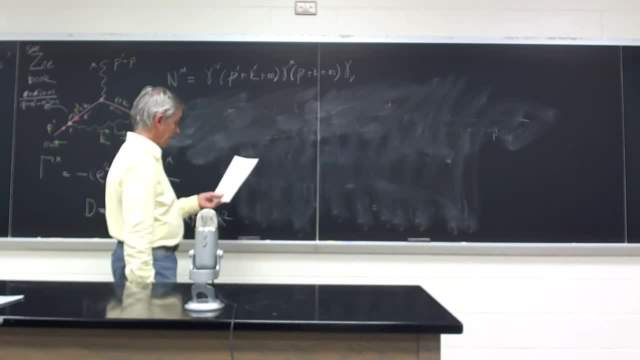 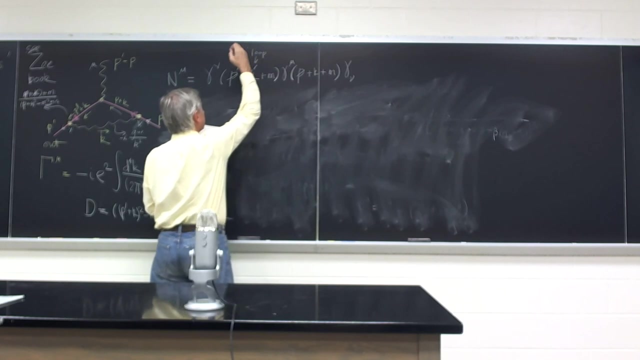 way we know how to compute quantum field theory and i think it's go to this guy rewrite this. you know we have changed. i'm sorry. i've erased transformation of k to this new variable, l shifted variable. so you know this is something that has to do with loop and i'm free to redefine as i wish. 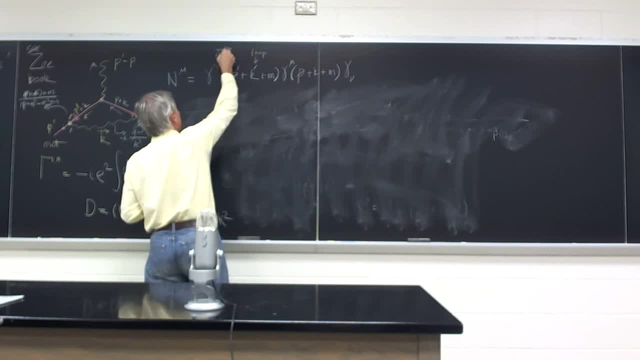 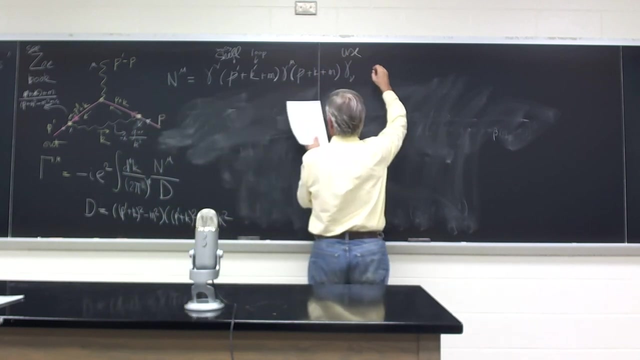 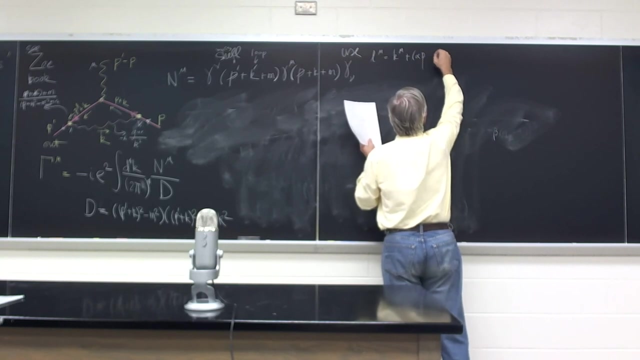 mass shell external. that i cannot mess with. we have just, uh, we can now rewrite p by- i guess i better write again- transformation, i guess the new momentum, internal momentum, the original momentum plus the thing. now that depends on our reparameterization of momentum. so it depends on that. 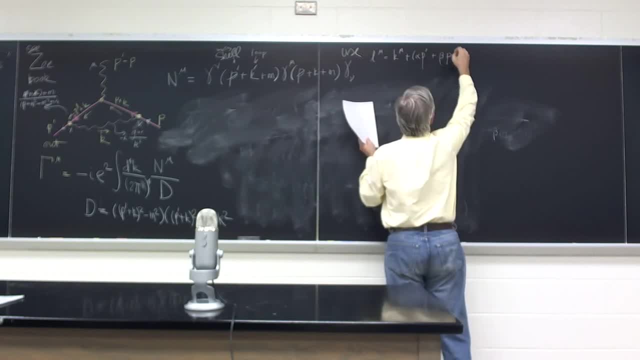 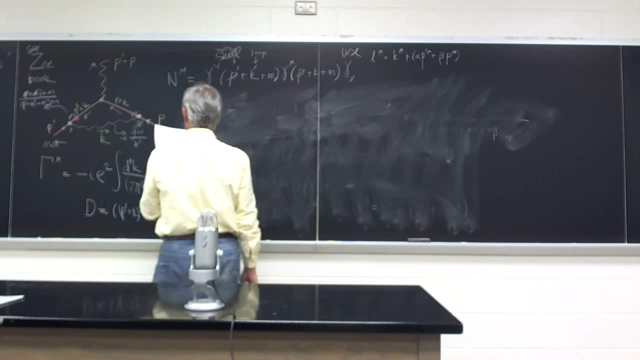 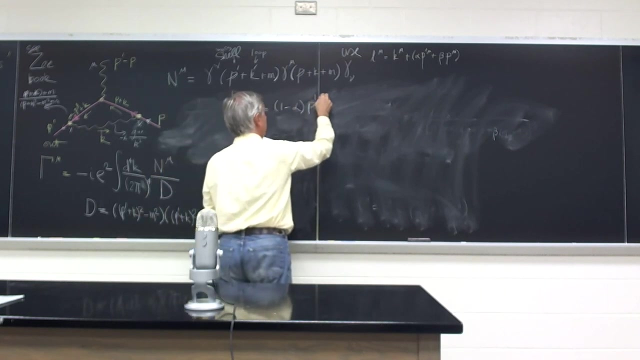 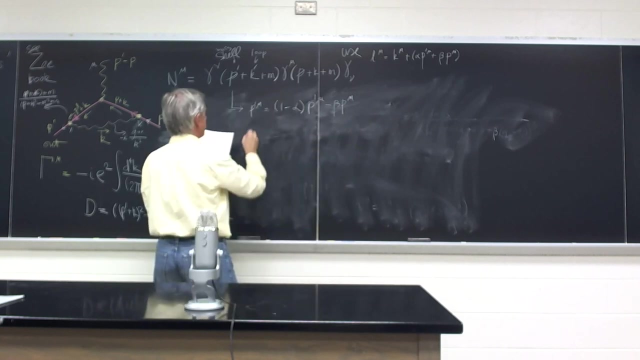 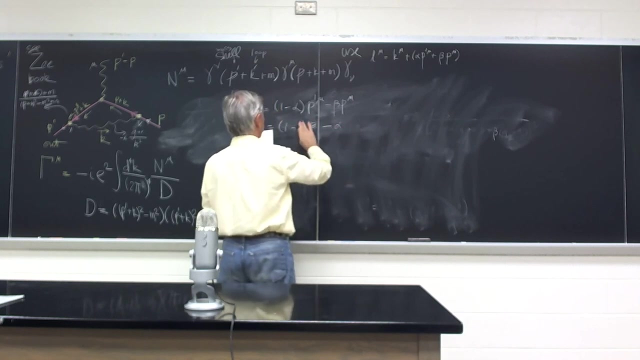 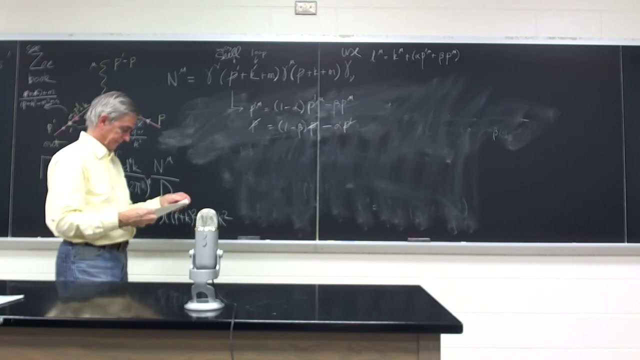 so if i substitute inside, then, uh, my p's will change. so i will get this, will become l, but this will become p. prime u is one minus alpha, and if i use this last equation just for the algorithm, i will just take that and uh. 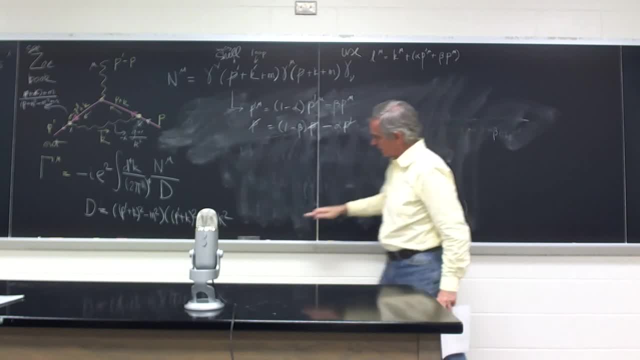 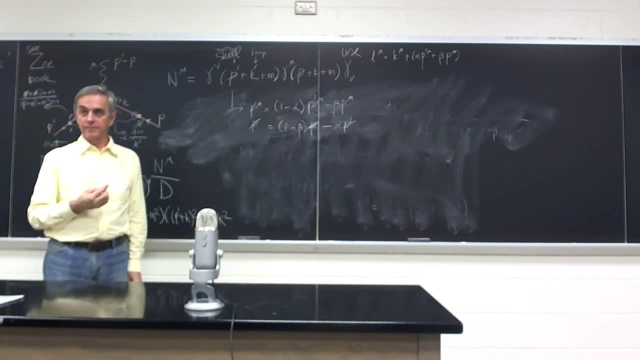 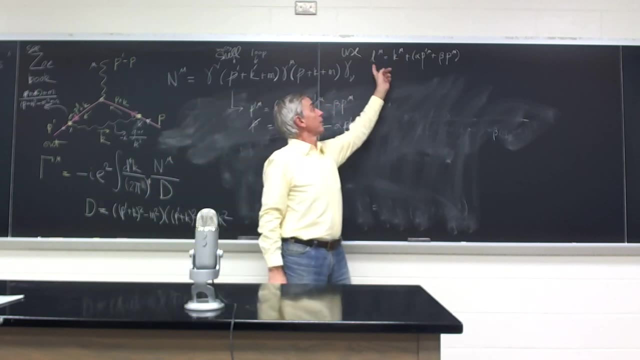 what i did is i in uh bringing the denominator inconvenient form for integration. i shifted my internal integration k. i shifted it to have a new origin, i added some components from the external momentum and then i will do the integral to the x. i will do in this case, the integral to the x went to the x first, who is the exact same as the z. the z is the commu integral to the z is the integral to the x, and if i have to do this, then the z is the integral to the z and then we can to provide the area of the. 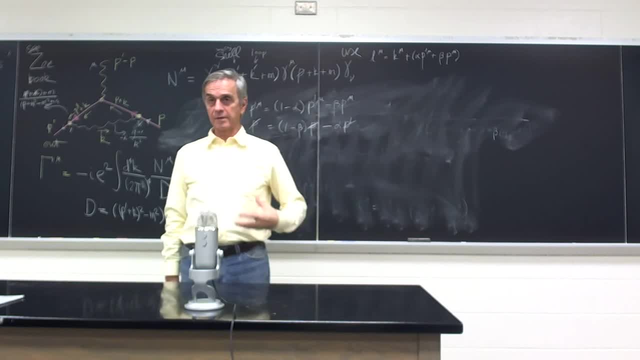 inner revolution from this. and that's totally legal, because I'm allowed to change the origin of integration as I wish. And the Jacobian of the transformation? it's a linear transformation, so Jacobian is one. So that's why we're suddenly having 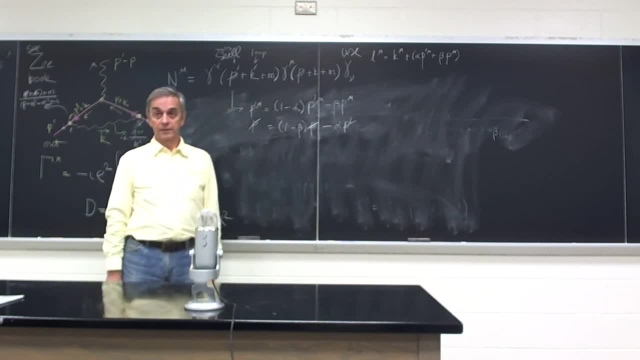 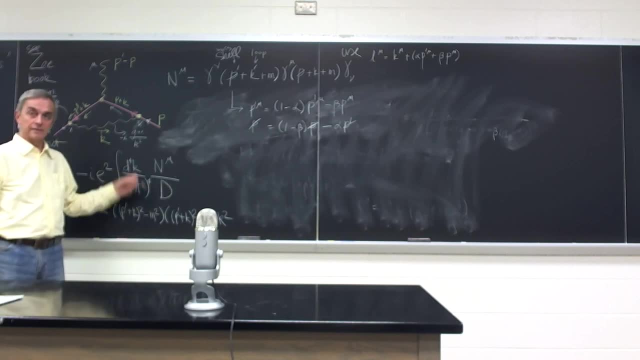 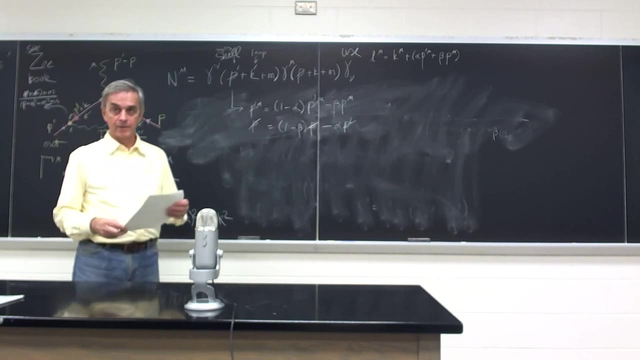 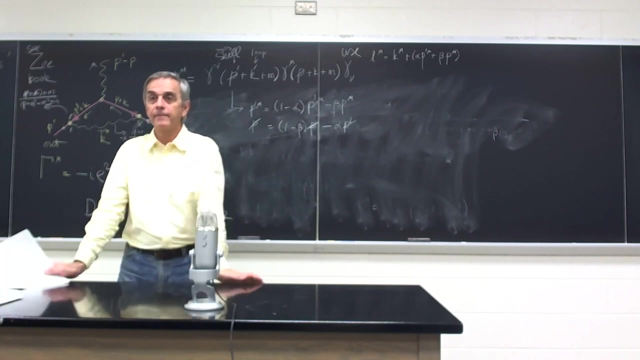 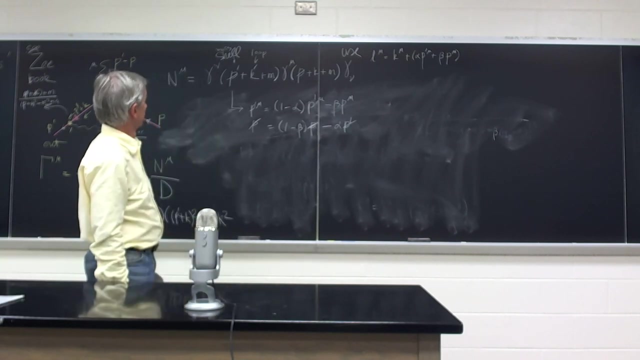 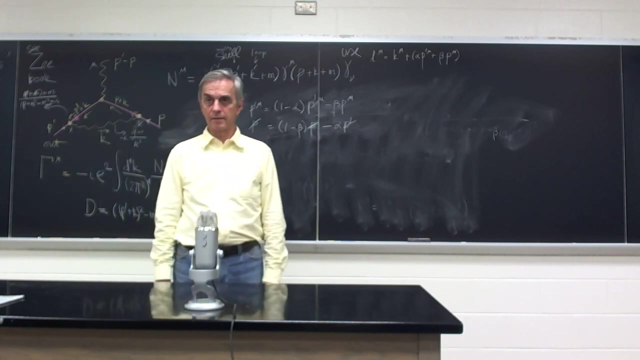 things that depend on alpha and beta also in numerator, because that's what we did in denominator. We redefined this integral to be integral over L Shifted variance. Okay, Okay, It's the same numerator, Anyway. power of objects. whether this thing depends on K. 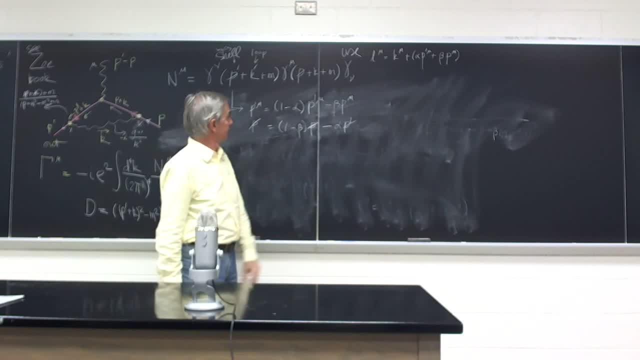 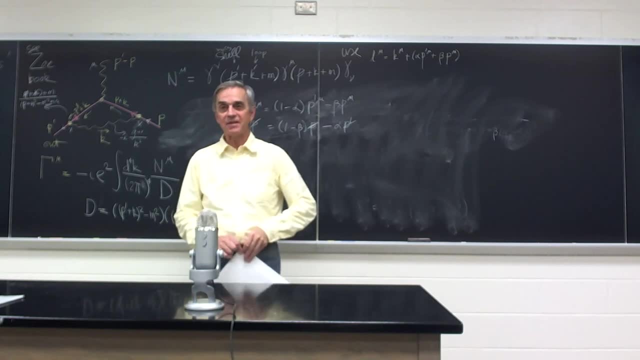 explicitly and it doesn't like that. now it depends on L explicitly, without being called something else. You might be right, As my wife tells me. You might well be right, which means she doesn't really believe it. Very polite way of saying it. 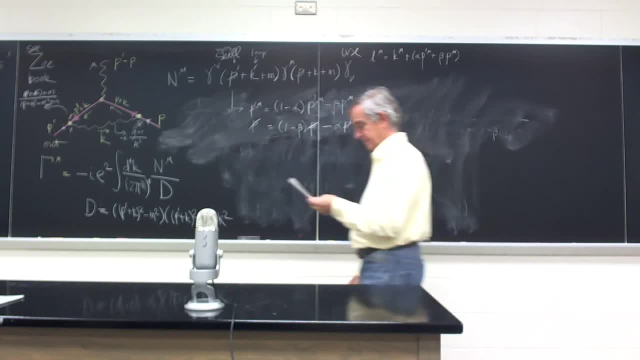 So now We'll do some Wunder, which is essentially what we want to do. This is as written. This is now a general vertex And it's a part of one loop. corrections to electron photon vertex. There are two other terms we ignored because they're not one particle reducible. 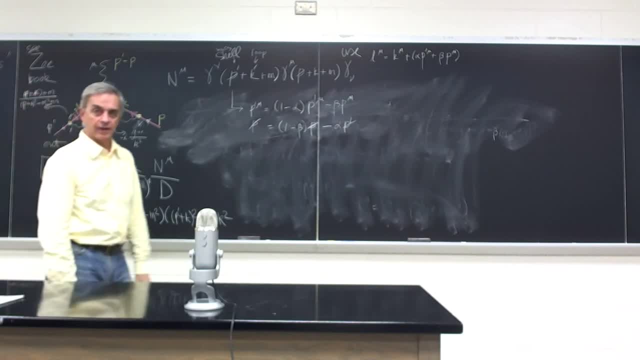 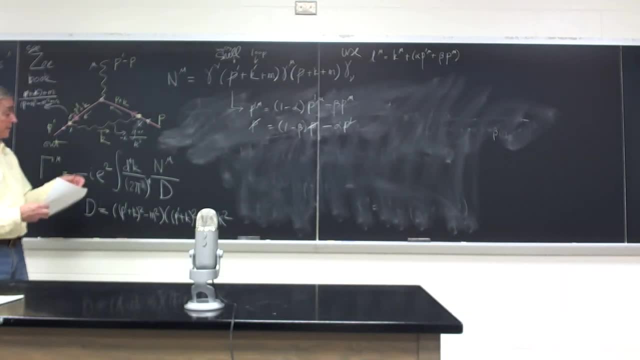 but all of them have to be put together to define a renormalized field theory. It's skirting around, but it looks like you'll have some time to do renormalization in the after Thanksgiving, So it's not always lost. So now, 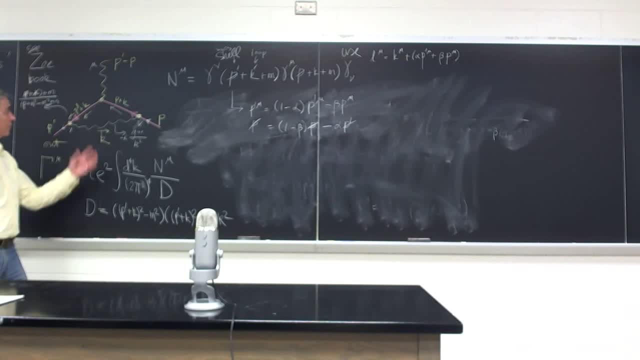 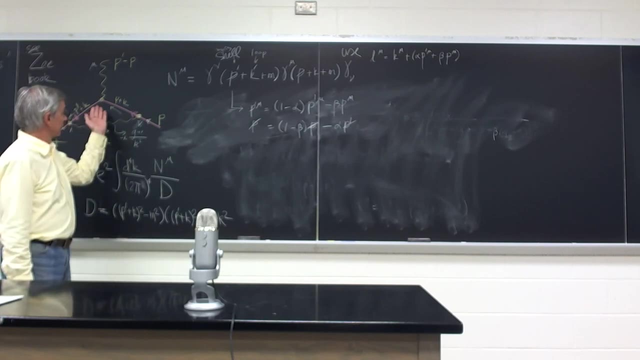 The next step of manipulation will be just to isolate the magnetic moment part of this vertex, because this vertex corresponds to so-called charge renormalization or just, you know, strength of a charge, And it has a contribution which is proportional to this sigma menu to the angular momentum. 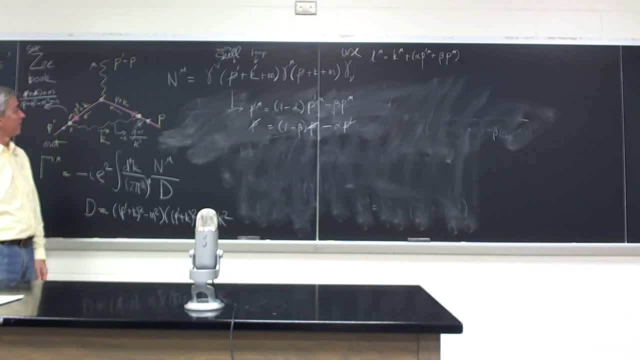 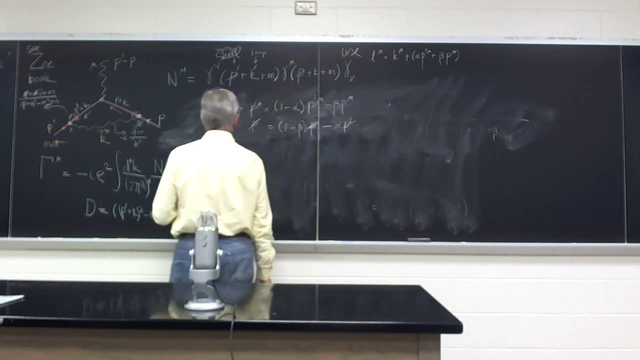 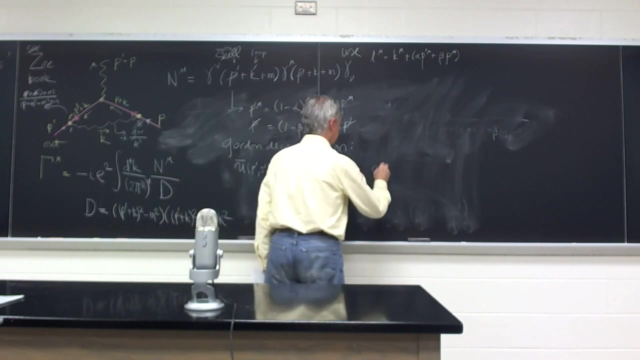 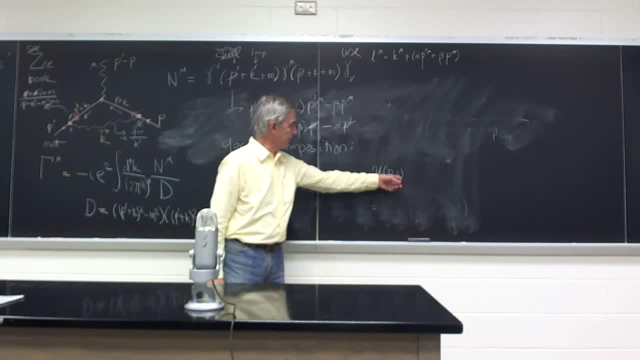 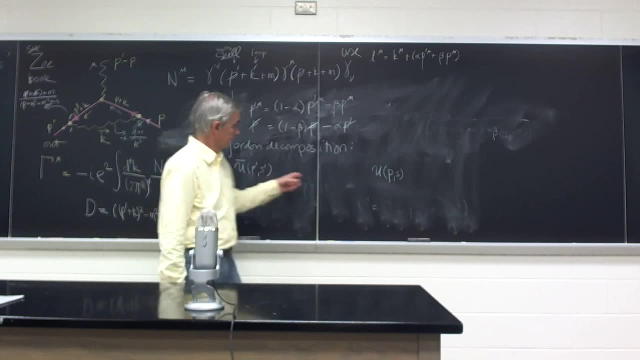 So you know this means is you have the matrix element. If you're thinking in old quantum mechanics, spin can be up and down for meaning. So you have matrix elements that say that external field can actually flip the skin. so that's why S should be written there. 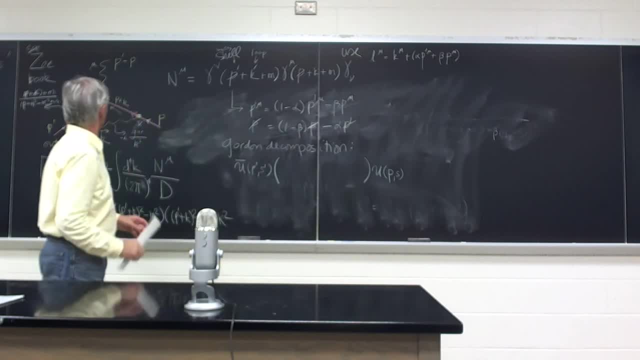 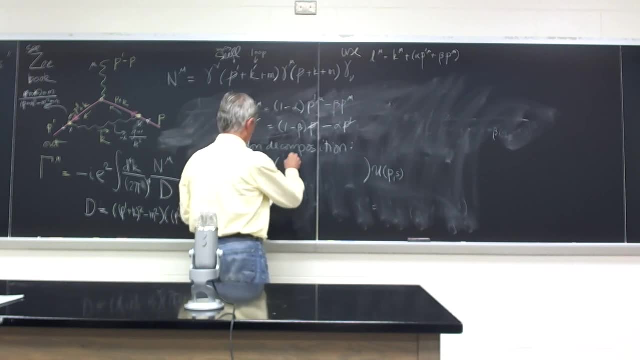 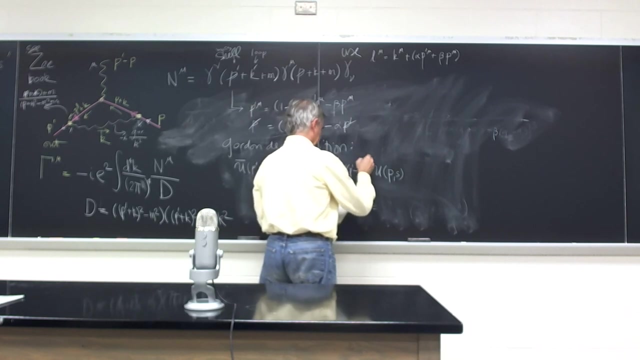 And then the g mu nu. just this vertex by itself could be written in terms of p mu plus mu m. so we derived them last night. And this is the commutator of two-gammon matrices, Which describes the coupling of magnetic moment, of electrons, this external moment. 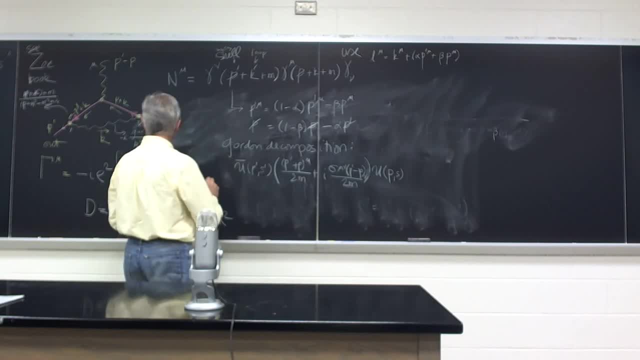 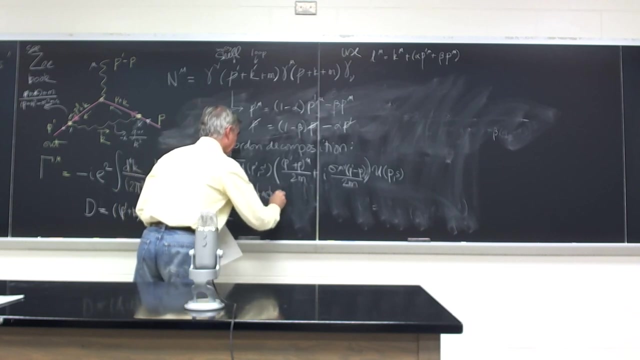 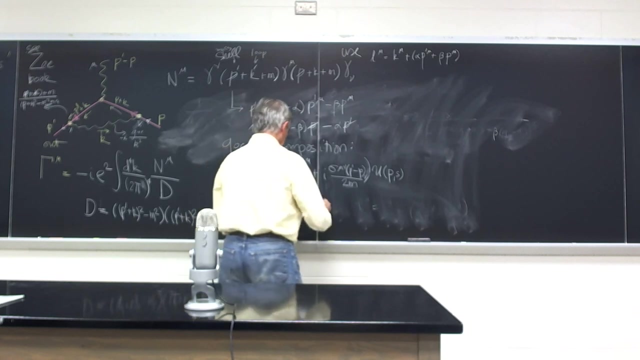 And this we also did last time- that it can write the form factor. So that you can write the form factor, So that you can write the form factor. So this is the general thing of this one-particle reducible guy. If you have corrections to any order, they would contribute. 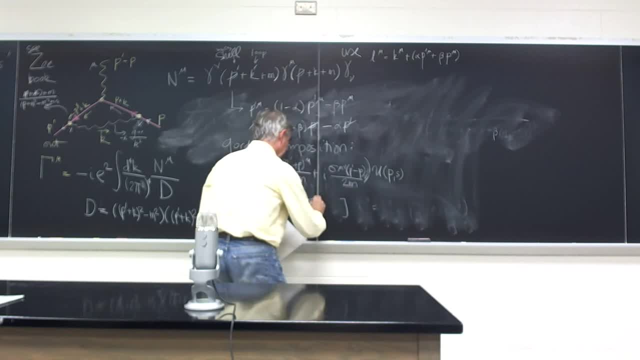 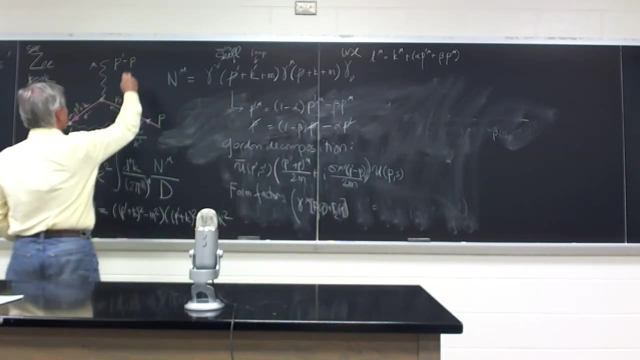 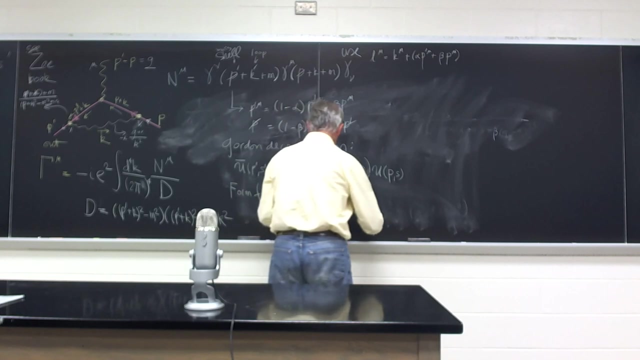 And now p prime minus p is called q in this formula. And now p prime minus p is called q in this formula. I can write it down If I had same OR and same P meets or theулs I have on the FamilyIQosis. 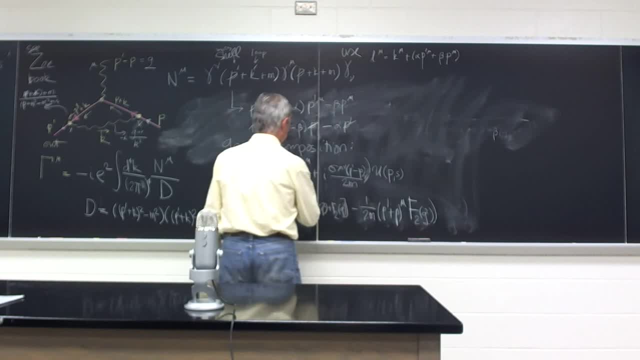 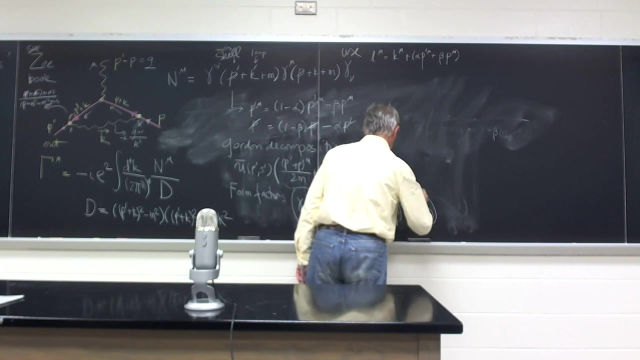 we have the link to the in the written form. I will show you too. See here: n1.. 2. 10. n1.. associate the magnetic moment term with having a momenta in the vertex. This has to do with magnetic moments. 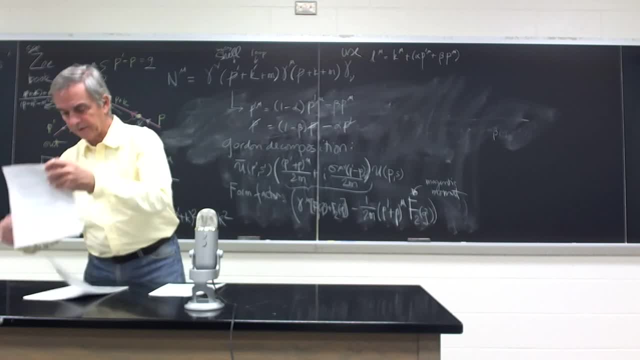 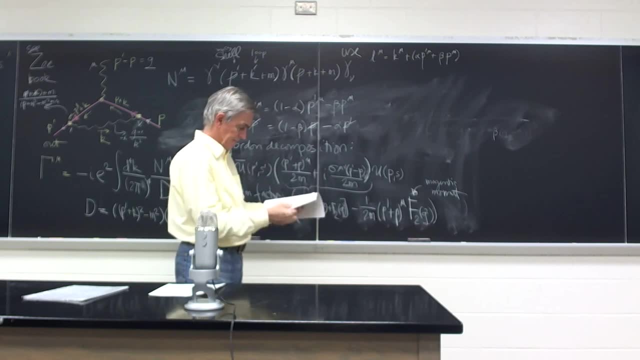 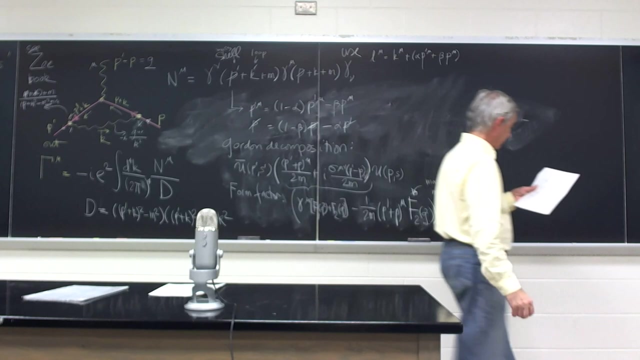 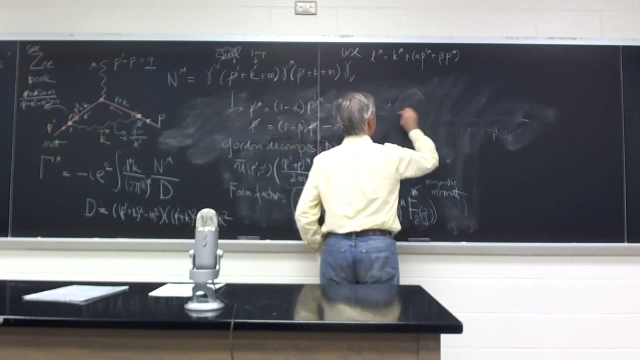 Let's just check my notes from last week. Okay, so what I wrote last week is something that made eminent sense. You have all possible one-particle eviscible corrections. So photoimmune selection in the left canal And evaluate on the left cell. 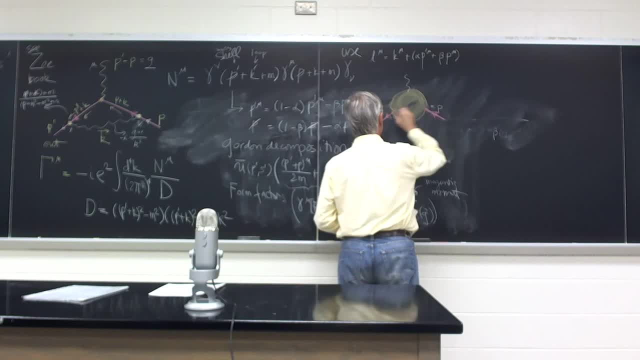 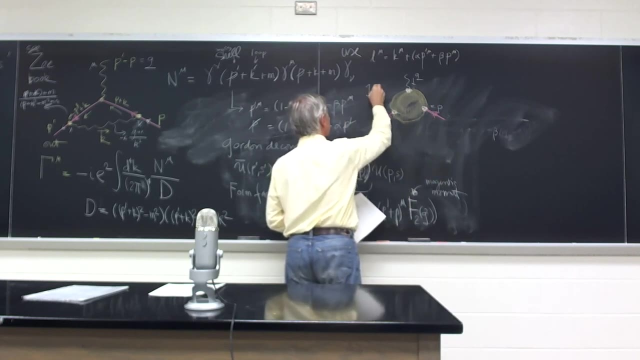 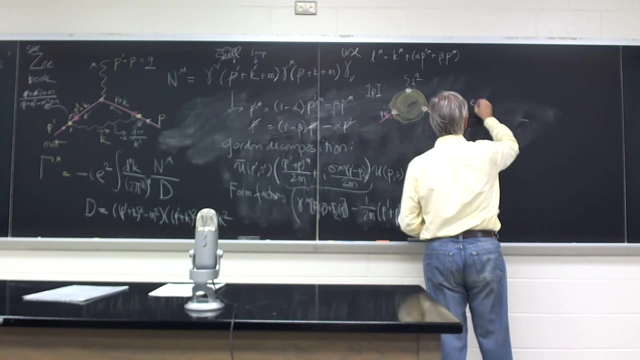 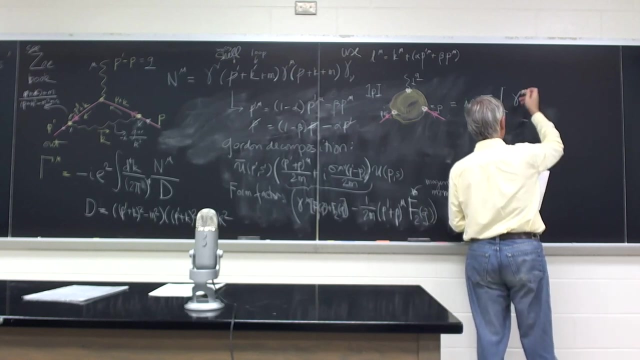 So this is p-momentum in, p-prime out and p-momentum in. So you know one-particle irreducible three-vertex, That's one RE. So that's the bare vertex And then all corrections that contribute to the vertex. 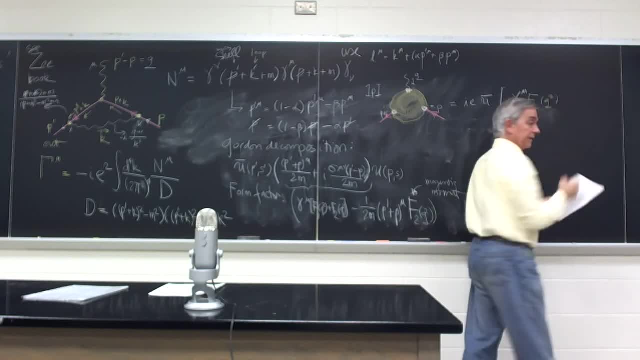 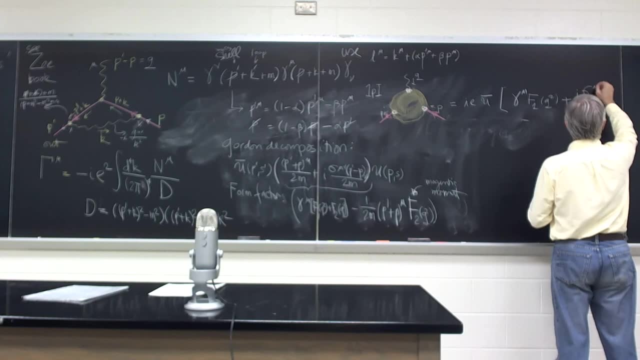 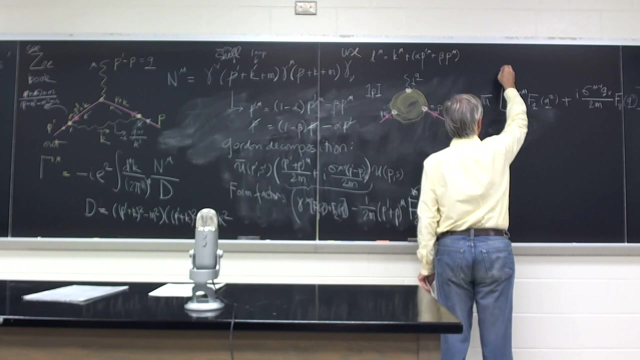 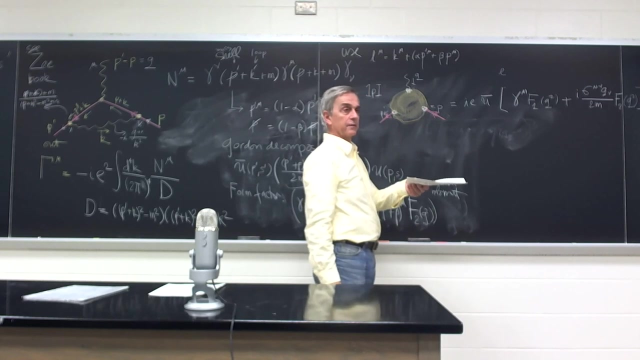 gamma vertex square. They can be interpreted as child brain remuneration, As I sigma mu, mu, mu mu Square. And in experimental measurement of charge, you're interested in charge just in the static electric field, So you don't impart momentum to it. 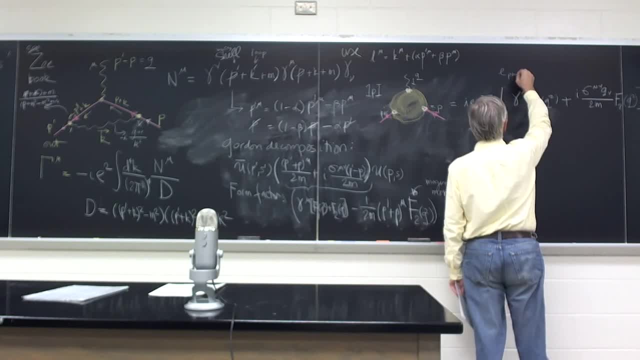 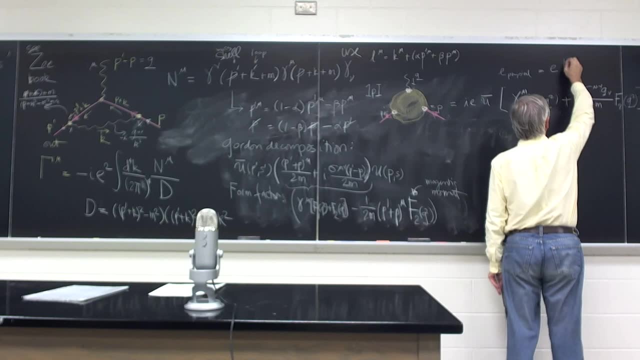 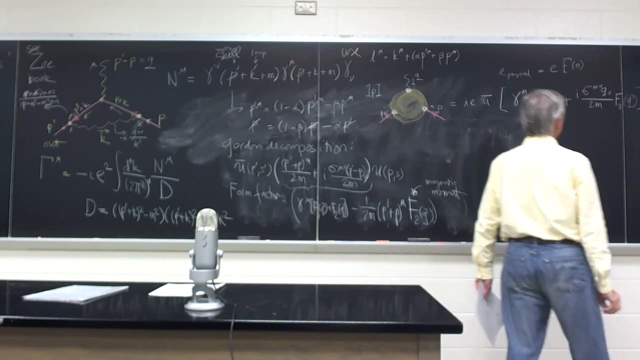 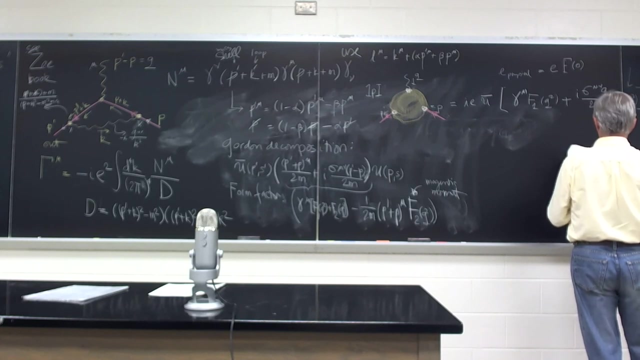 So we normalize our, you know, physical charge. It's the bare one Times everything that quantum mechanics got. Evaluate the zero external momentum. And this guy, F2. F2. Evaluate the zero. You did it last time. 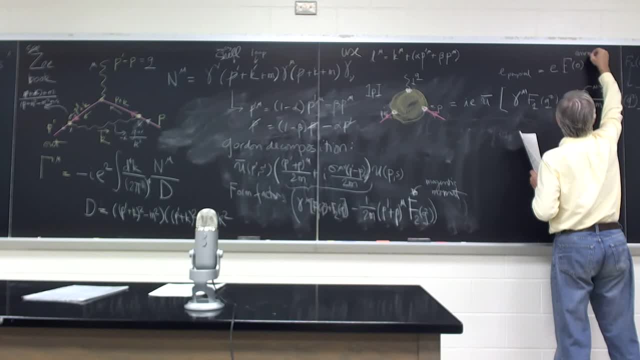 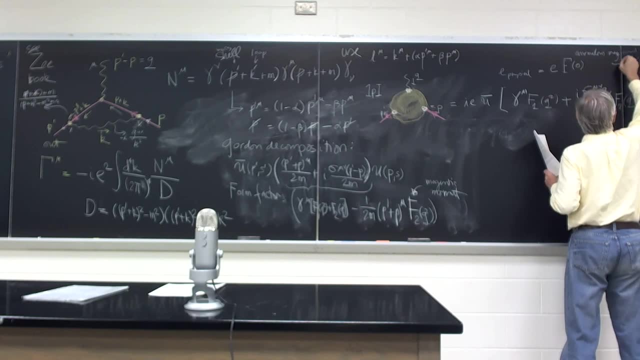 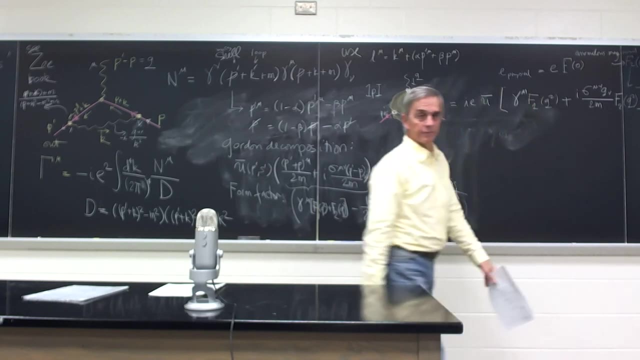 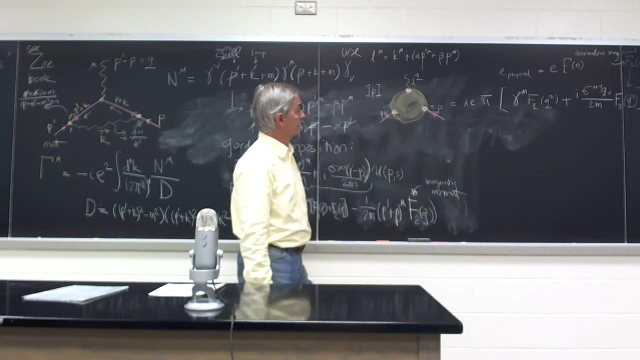 It's interpreted as a normal magnetic moment. So the way this thing works out is that the Dirac prediction from relativistic physics for magnetic moment works. There is no normalization for that guy. Once you have fixed the physical charge, it's absorbed in that. 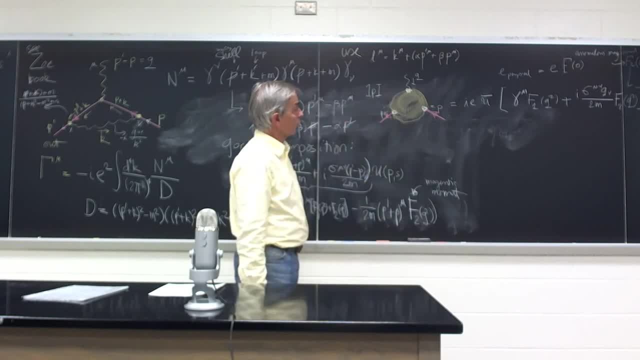 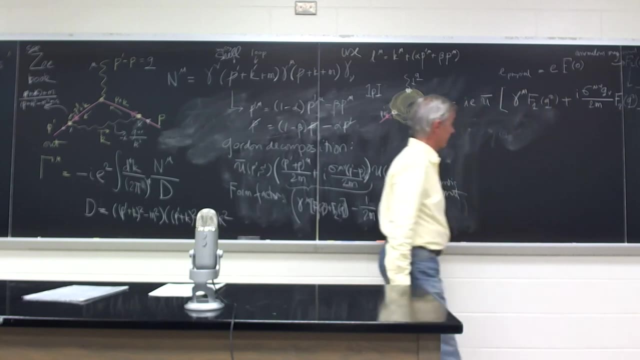 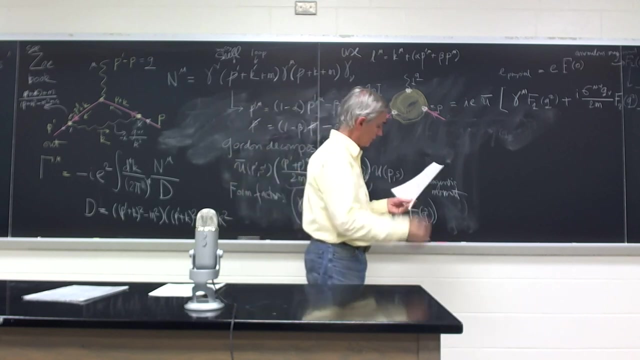 That gives us, you know, one in this, in some formula which I'm writing here, I guess, And Schrodinger anomalies: the difference between quantum mechanics and Dirac relativistic Quantum mechanics. Quantum field theory- Dirac relativistic quantum mechanics. 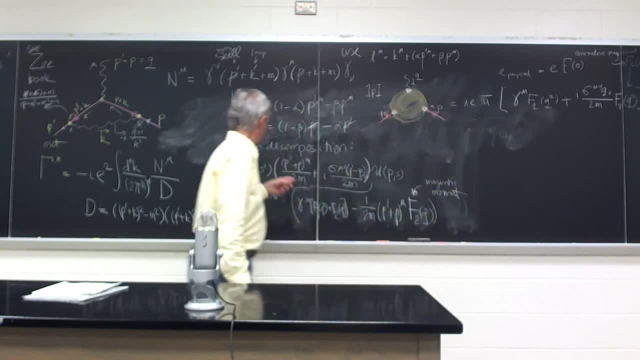 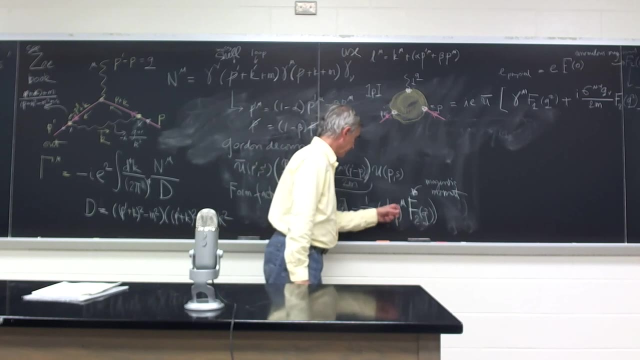 So now I did a little bit of this using the Gordon decomposition to bring it to this form, And that's just convenient for calculation to have anomalous magnetic moment associated with momentum up there. As you will see, this is very handy because 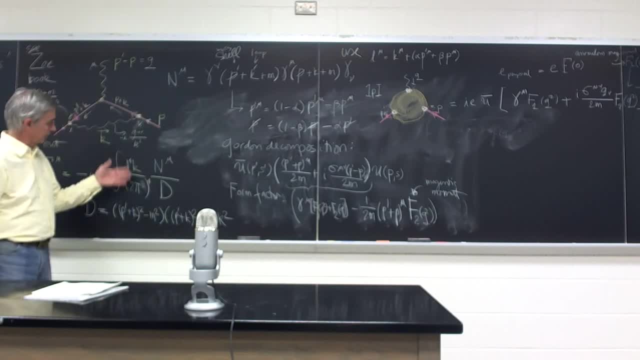 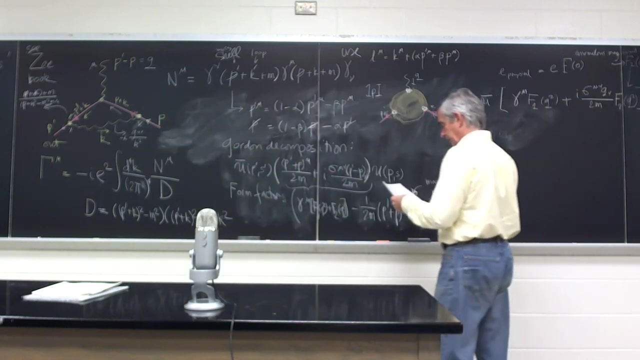 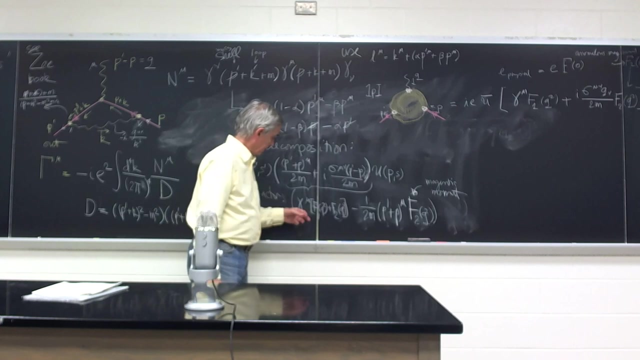 this integral looks like it's logarithmically divergent because it's you know something of order four integrated And the denominator had a power four Looks like power six. Okay, So now we are not interested in the. this is not a very persuasive argument. 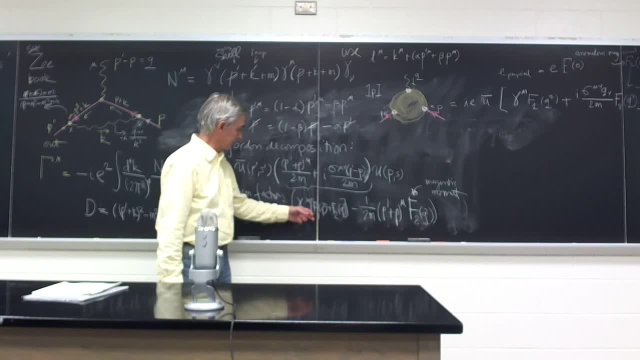 So we're not interested in the stuff that renormalize the charge. That's for somebody else to worry about. So we'll drop anything that has to do with gamma u and we'll only look at this part of denominator. And here is the denominator. 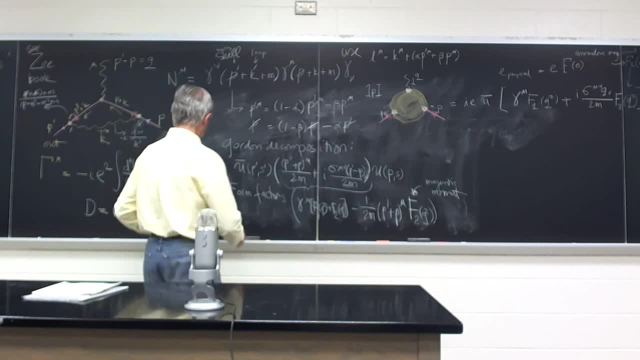 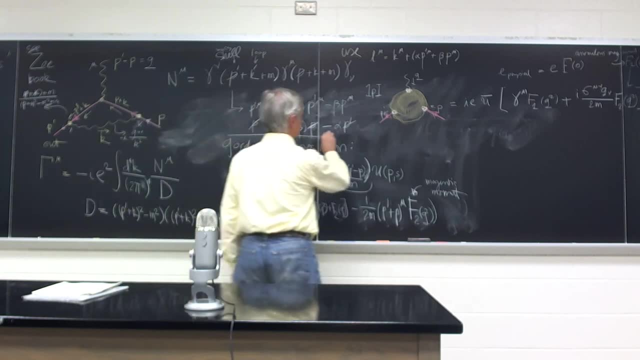 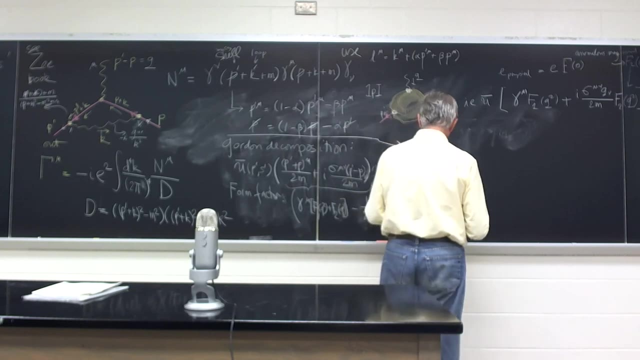 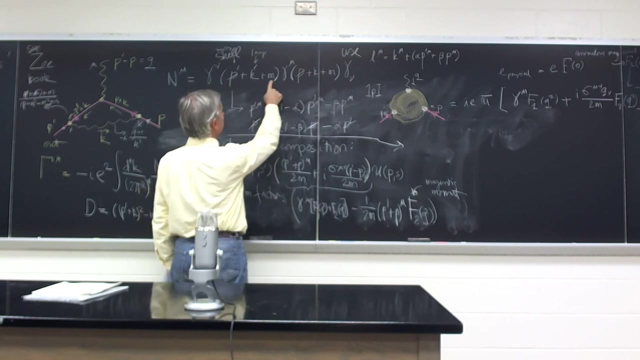 So let's work it out. So first thing we notice is that we have a very simple term and this is a constant and this is a constant right. So there'll be term, there'll be g mu. you know this thing. 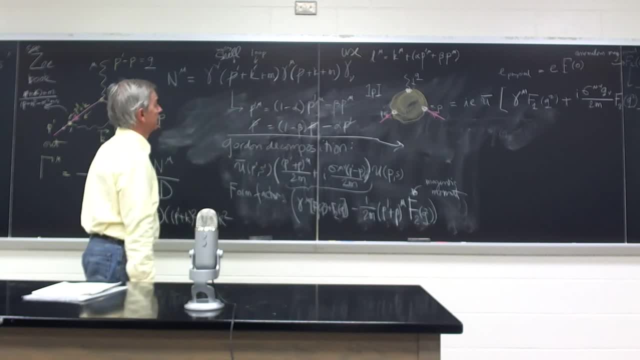 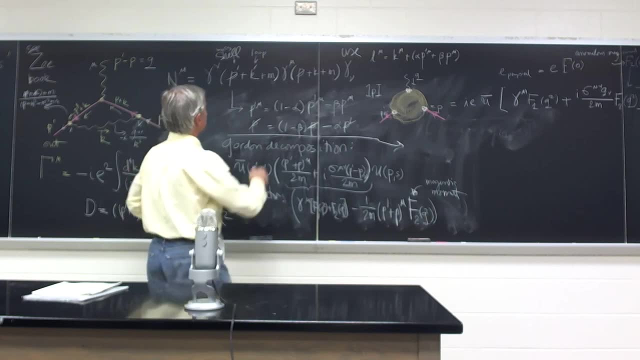 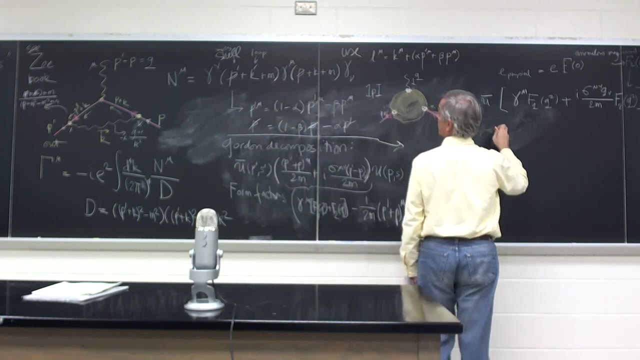 this gamma in the middle sandwiched by another gamma, And this is of order m, And so there'll be a term here. There'll be a term that looks like m squared, Gamma mu, gamma mu, gamma mu, And you know that that thing is. 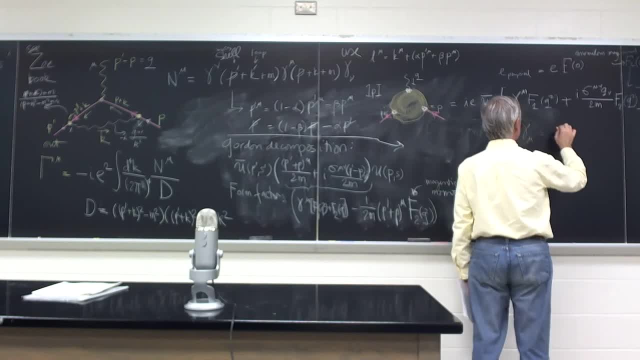 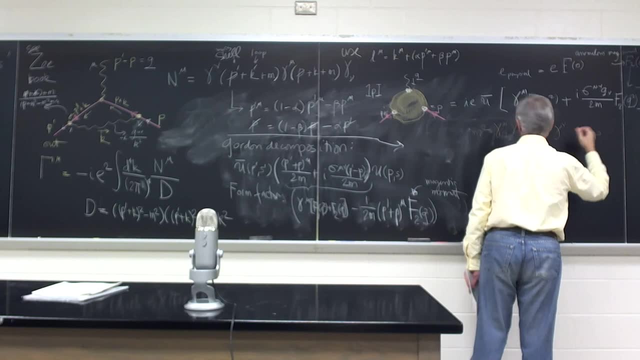 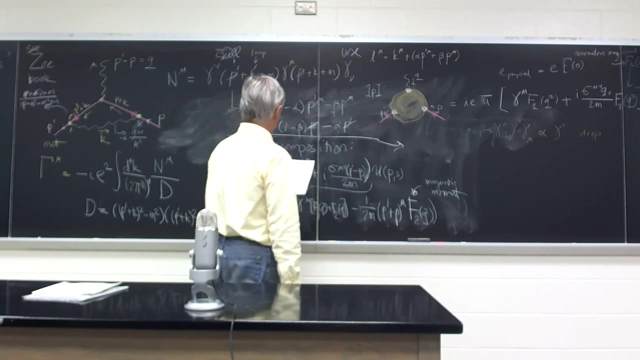 if you work it out, that's proportional And I think we worked it out. It's proportional to gamma mu. So we'll draw that That belongs to this part of the calculation. So that's this part to drop Right: gamma mu. 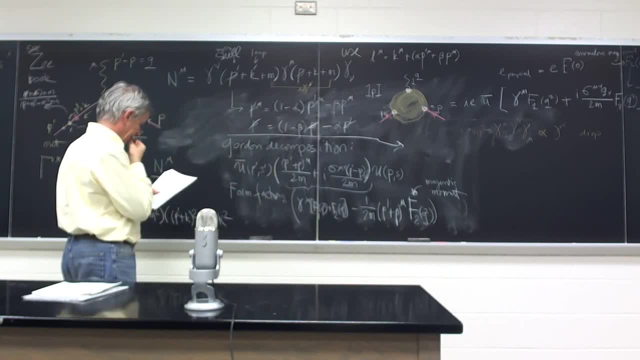 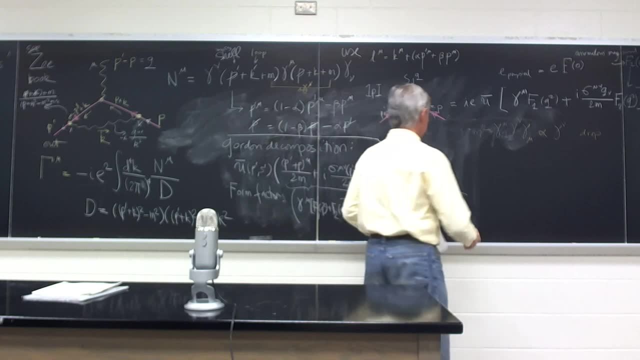 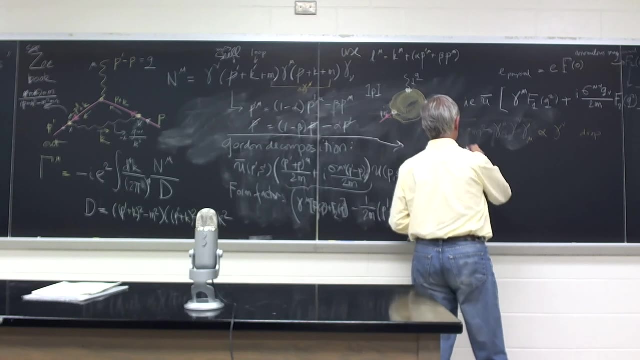 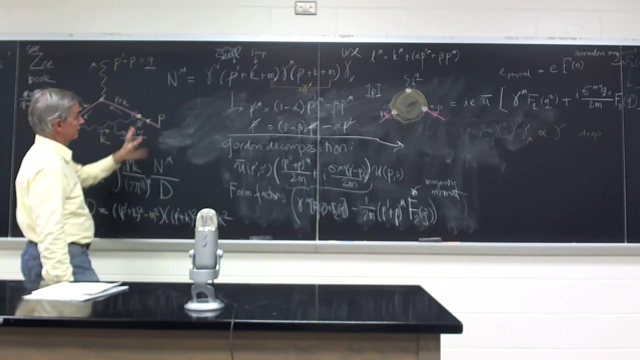 We'll drop it. Then there are terms of the following form: Maybe let me have it in there. I think that might have mu again, but just in terms of l's. Then you know, I'm integrating a d4k. 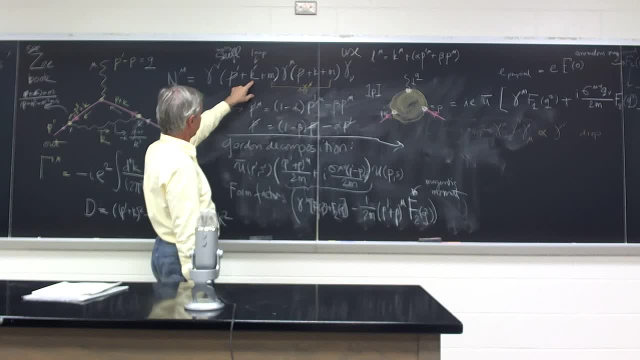 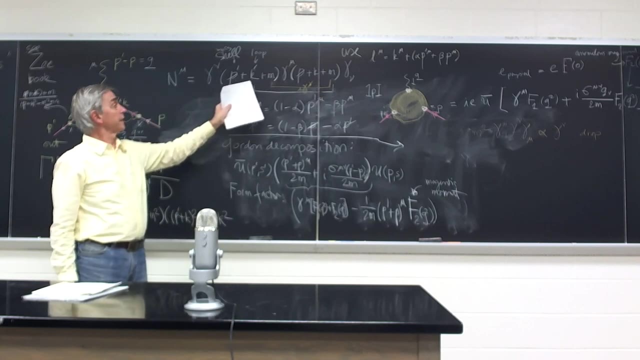 We'll get the change thing for a moment. And if I pick up k from here and m from here- So I look at the cross term of this kind- Then I have an integral which is odd in the powers of k. 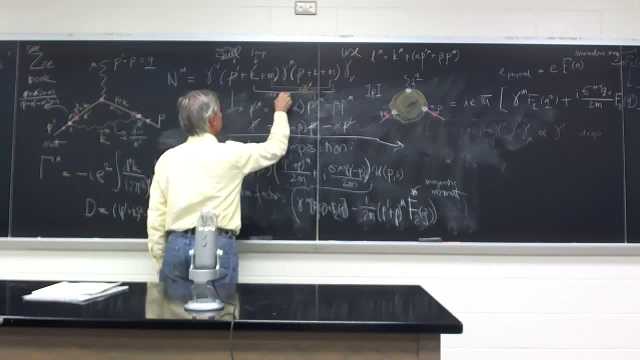 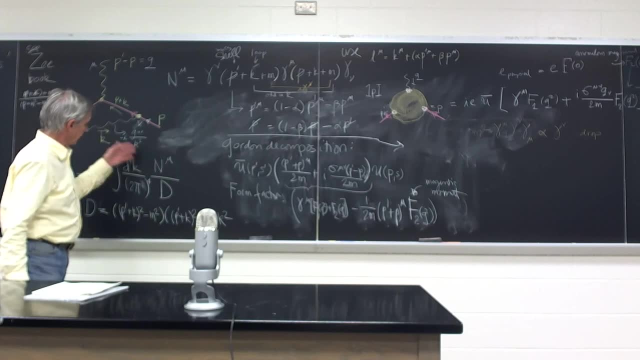 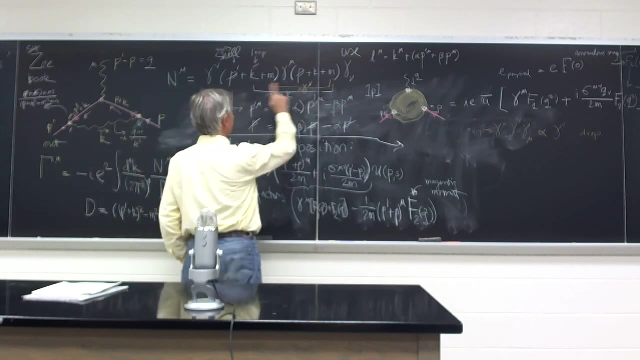 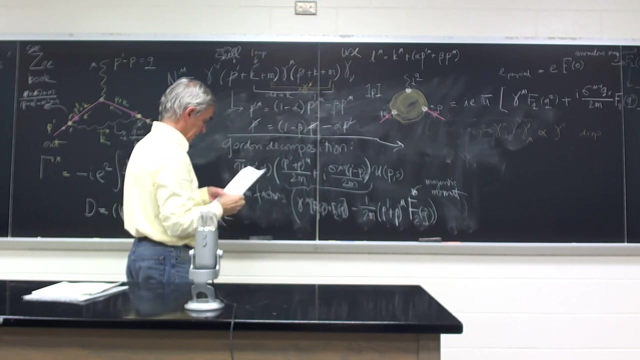 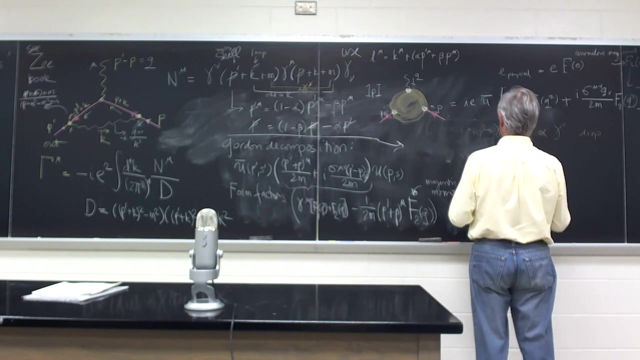 This is odd. If I integrate overall space and odd function, I get zero. So I can get zero of that one. Then of course there's another cross term. I got All right. Then I'll have terms that look like: 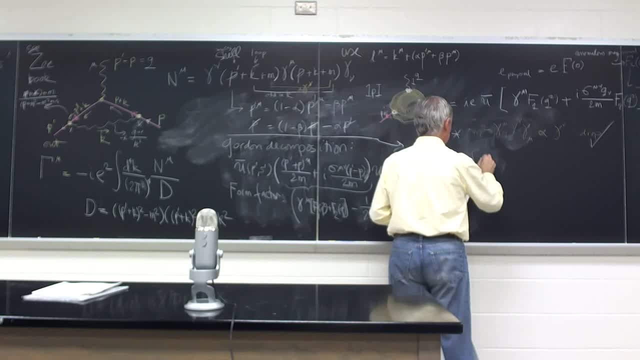 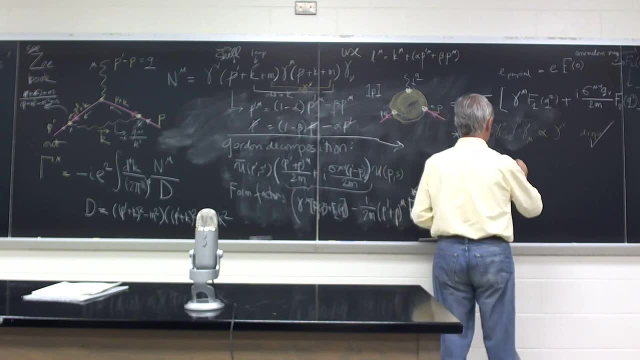 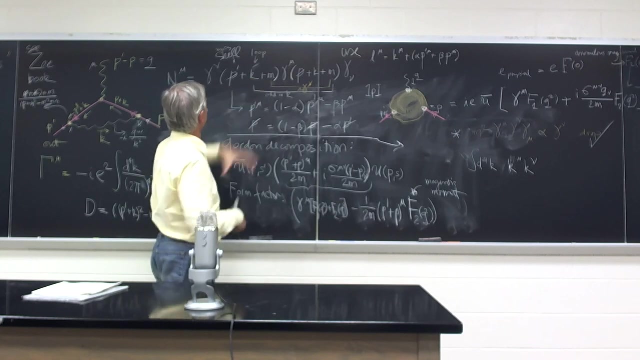 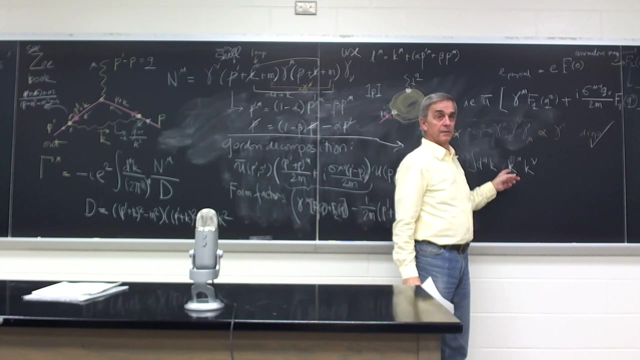 l u no, k, mu, k, mu. So that will be the terms when I test sloshes again. Yeah, Sloshes, So that's this term here. the cross. Now if mu and u are different, 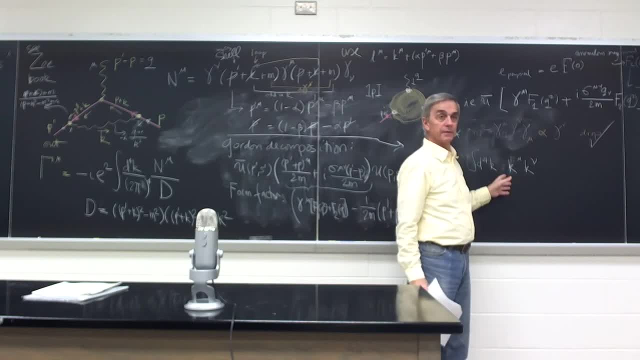 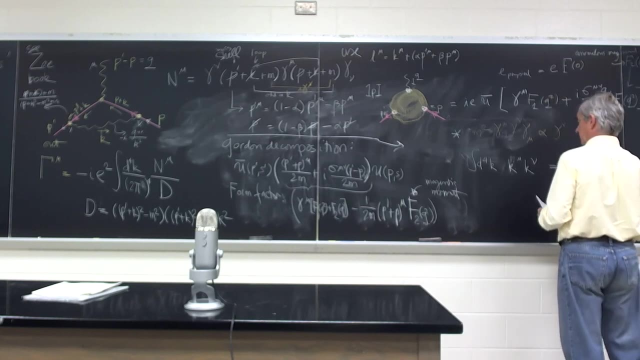 then integrating. this is odd in each one of them, So it vanishes. So I can get only non-vanishing contribution if they're the same And you can easily show that this is one-quarter integral of B4K K, K-square G, U, U as. 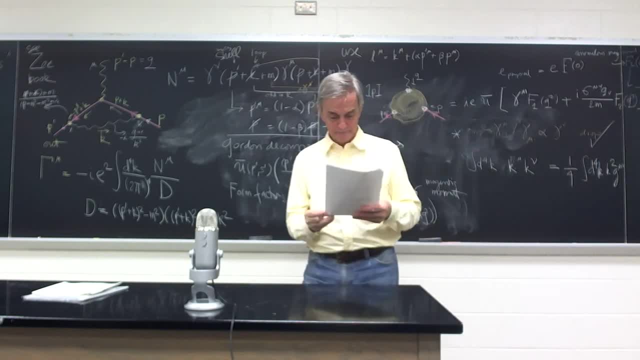 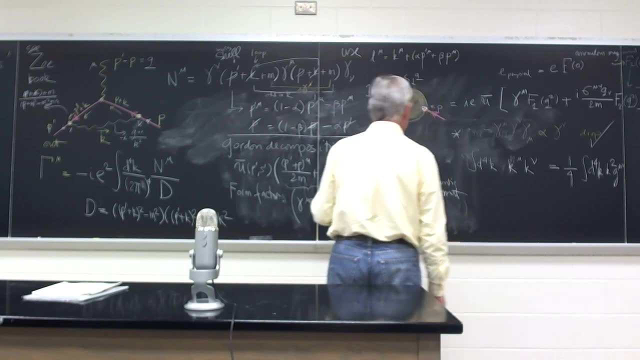 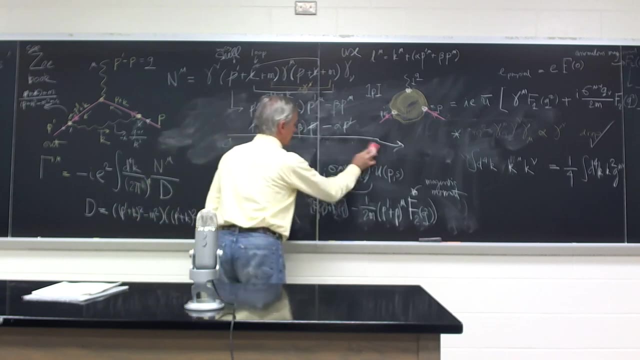 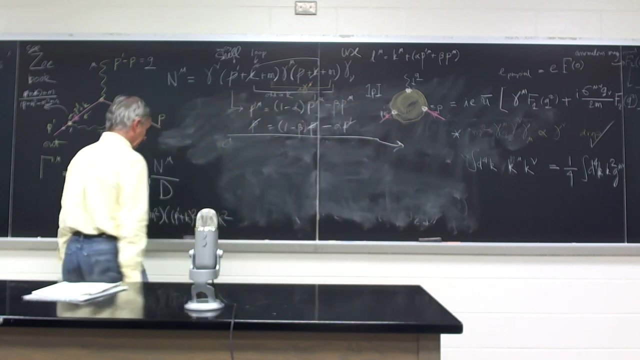 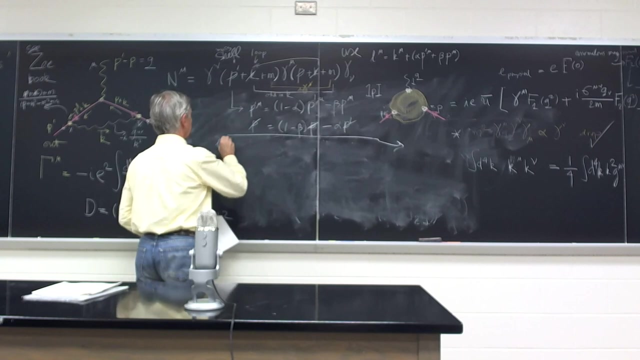 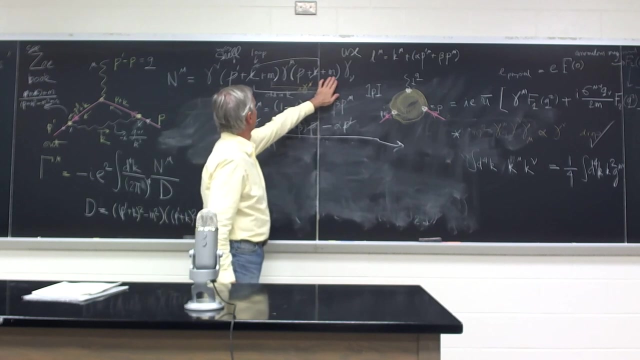 the only symmetric dependence that we have available. Then there are terms which are linear in M. That means I pick up M factor and then I pick up K And then I pick up K And then I pick up factor of this on the other side. 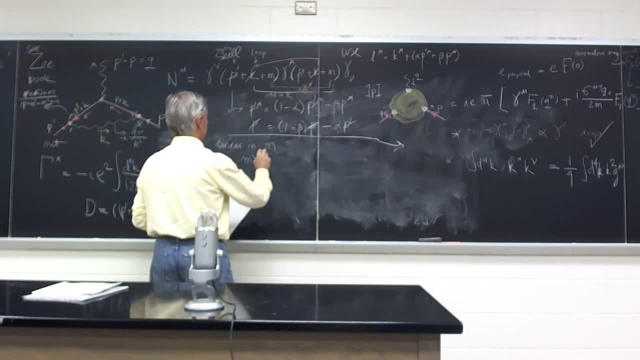 So they look like M, gamma, U, P slash as an example. So not momentum, but an external momentum: P slash from here And gamma And U from here And here I got an M from here, So that is. 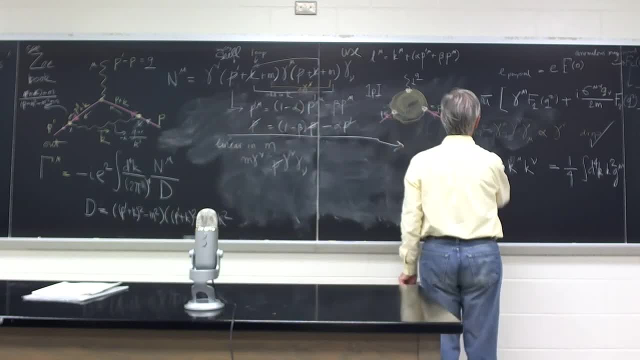 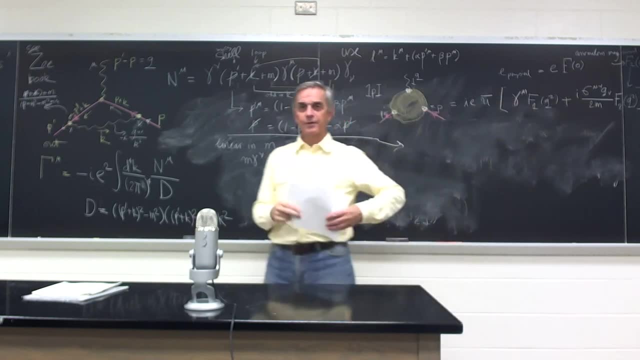 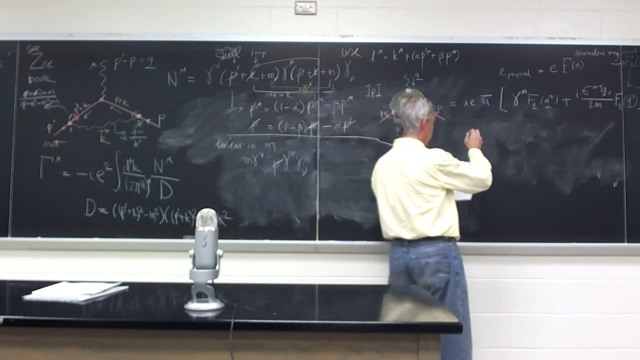 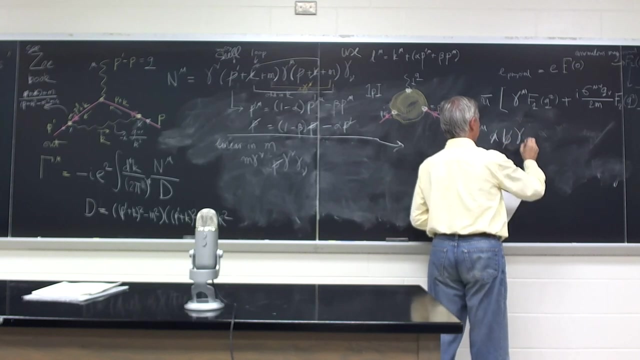 And to evaluate those terms. I really don't remember you know what gamma gymnastics I asked you to do in the exercises, But But Did I ask you to evaluate gamma mu? slash A, slash B, gamma mu- Was that part of the problem? 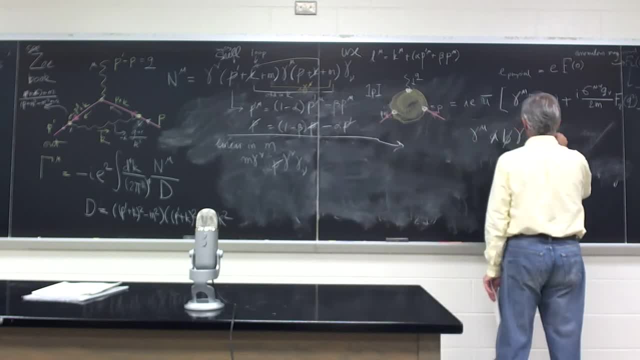 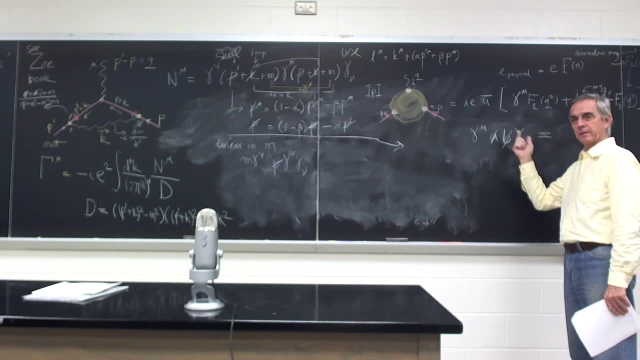 You know, does this stand with? these are gamma matrices. you use the anti-communicator relation of the rock, you pick up G and U and work a little bit And you realize this has to be a scalar number. And you know what scalar can you make from A4 vector and B4 vector. 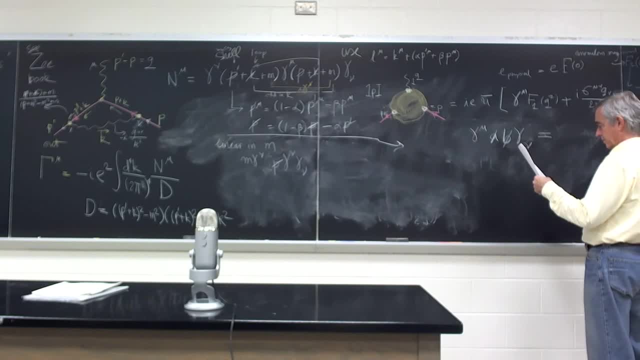 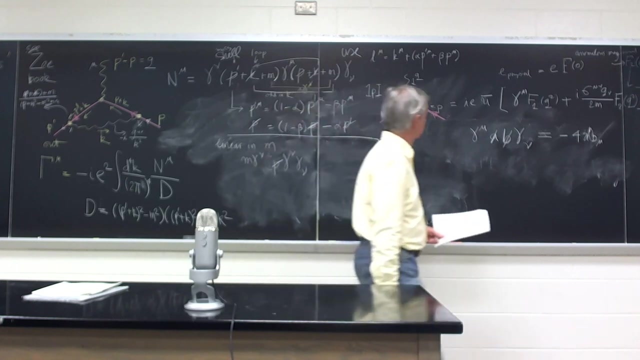 And after a little calculation, which I don't want to do now, we get minus 4 dot A, dot B. I can write it in covariance station. You should have both in the same, Yeah, of course. Thank you. Some of the external. 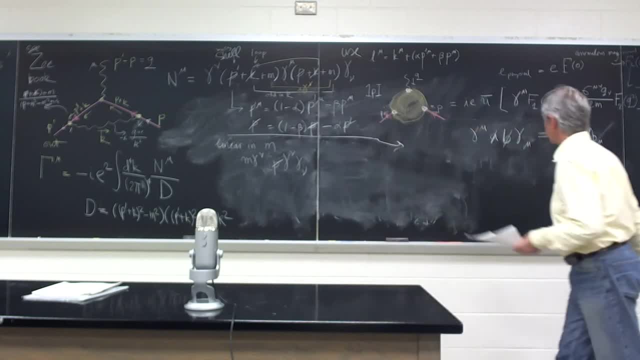 So, yeah, it looks credible Because if you have two vectors, you know what scalar quantity can you call from. Let me set the dot product. Thank you, Nothing else to do. And you know you have to compute the factor as minus 4.. 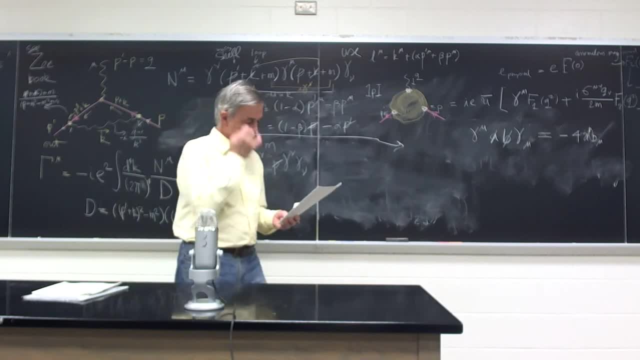 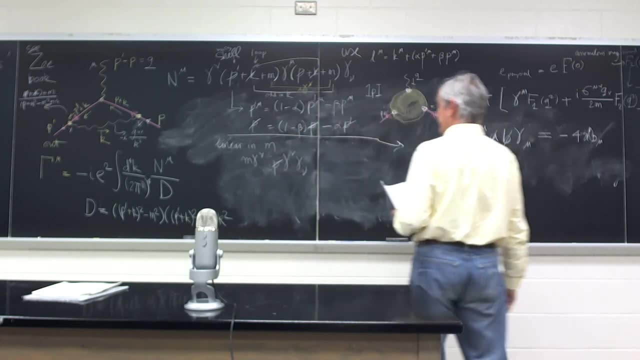 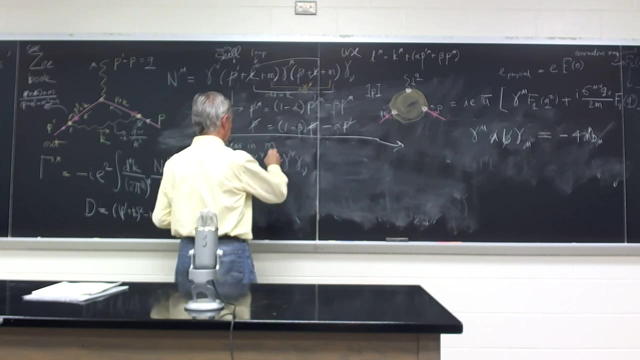 So that's standard Gerard-Gammon gymnastics. So if I put that in here, let's see. So I have two cross terms like that, Because it's also term. So this is probably E slash gamma, This is a gamma mu. 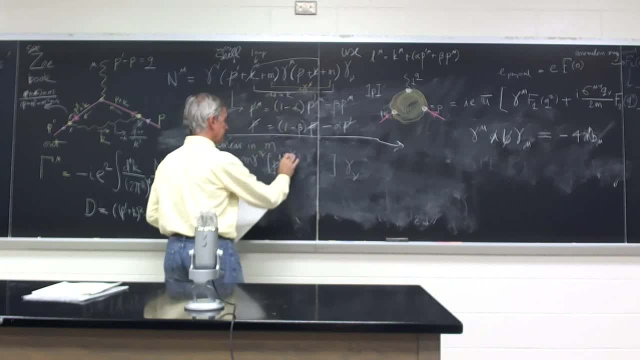 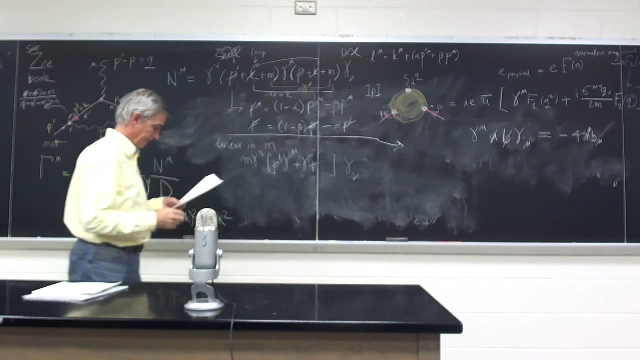 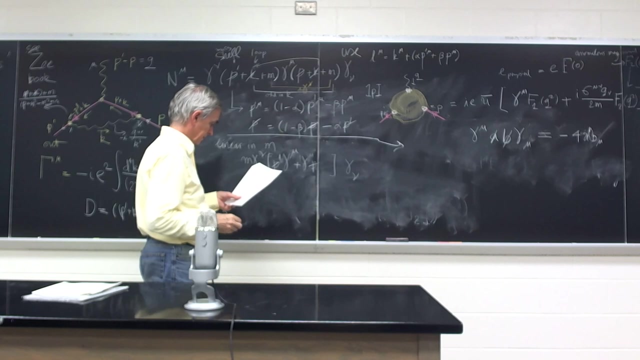 This is a gamma mu summed over two indices. And this is mu upstairs. And then there is also term that looks like gamma E slash. That's this guy picking up mass from here. The eighth angle will be this: coordinate Whoo. Another gang of eigens are also going to be. 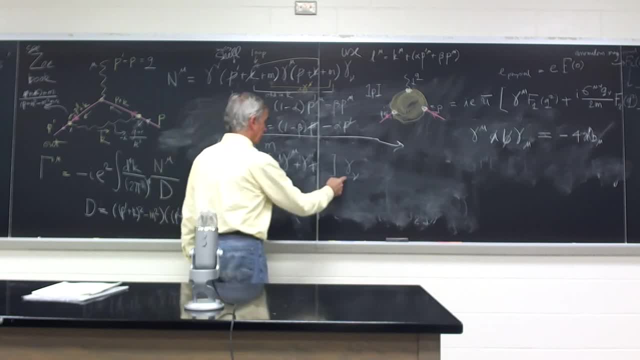 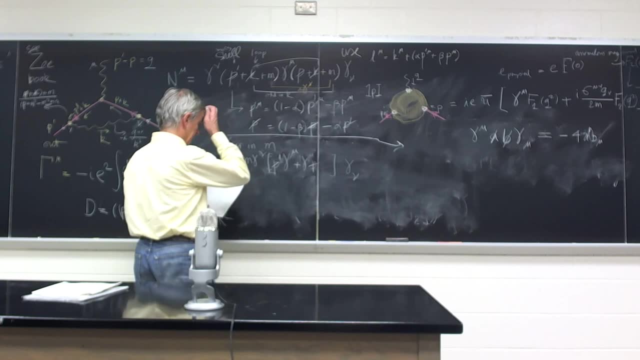 In the numbers And they know one, two, three, four. They have four gamma matrices in this form, So they by-grants. Azure is Two pi minus three, そして comes a value. Okay, Very good, Thank you, Thank you. 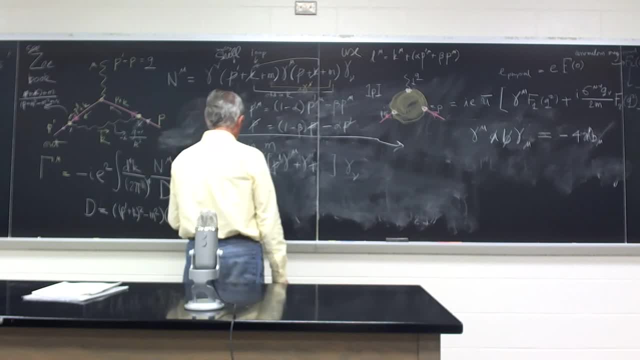 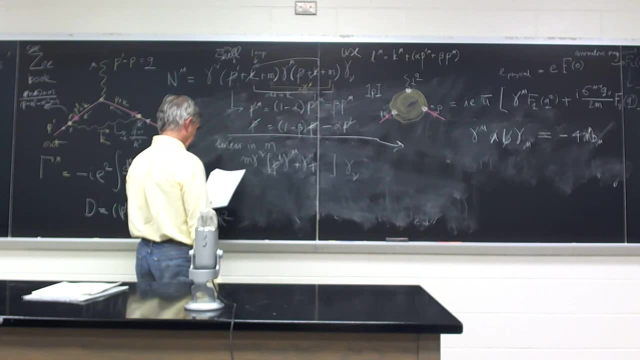 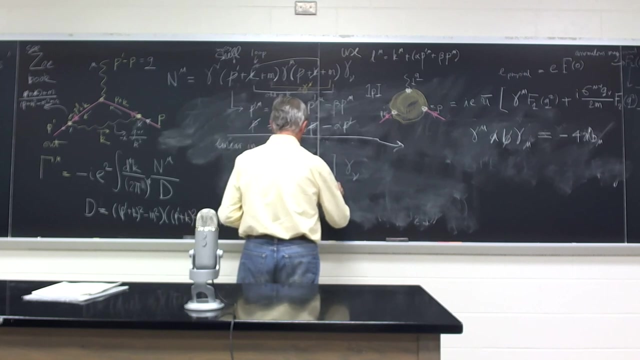 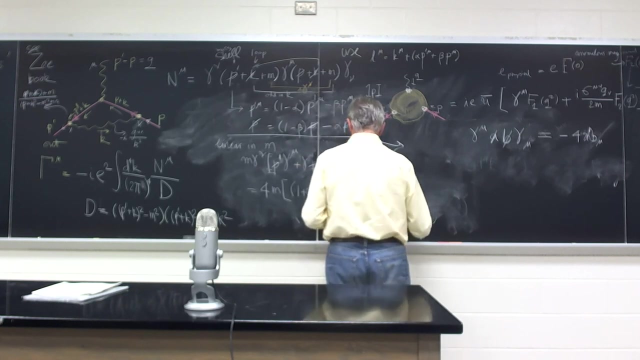 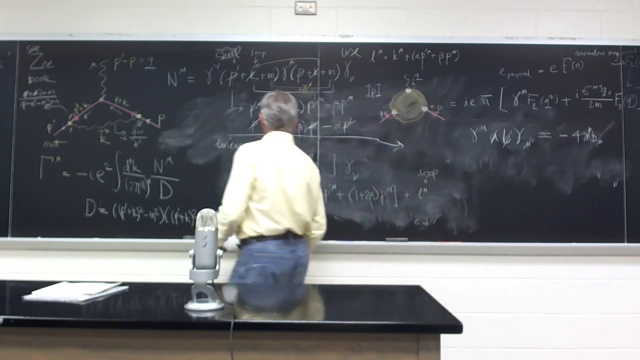 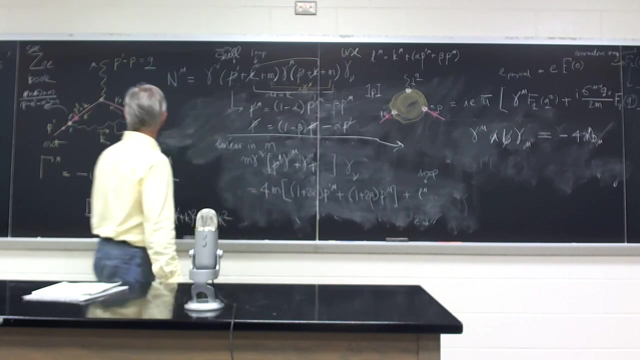 What you want to do is you want to anti-commute one of these guys because you want to make, you want to bring this form where you're looking at. So I use- I hope I didn't drop it- I use this identity here because I'll be integrating over L and not K. 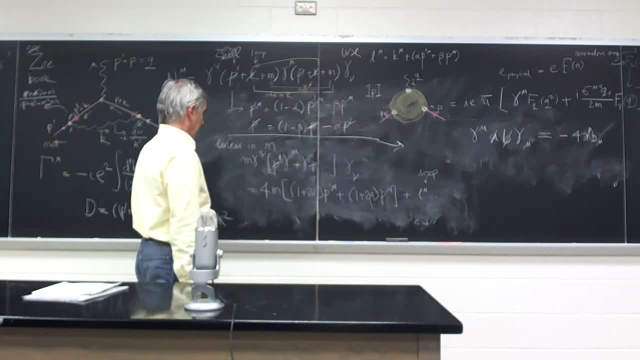 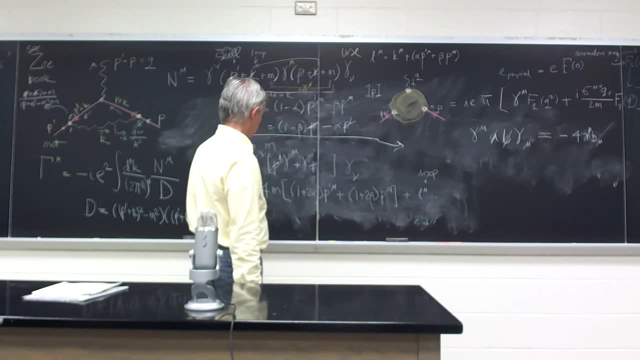 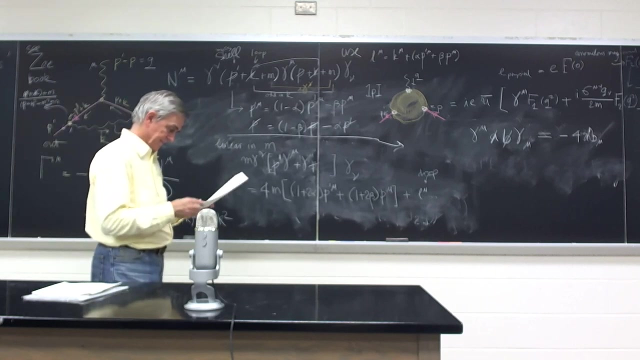 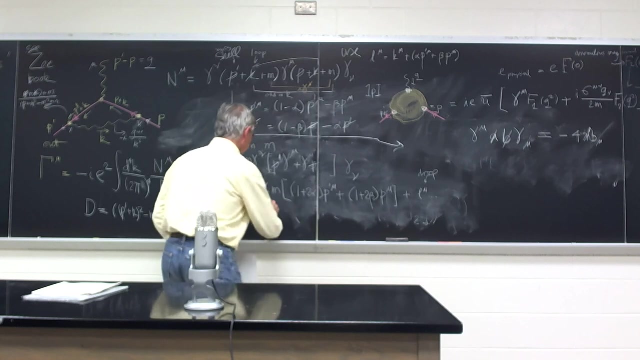 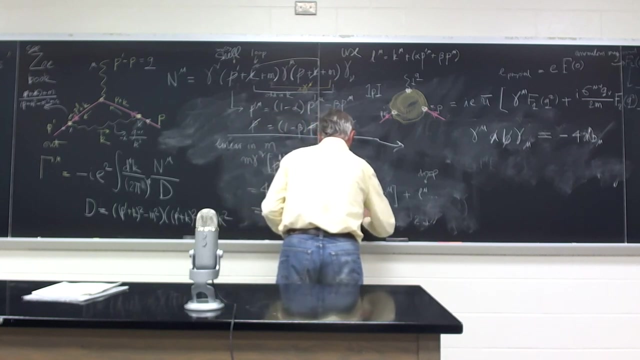 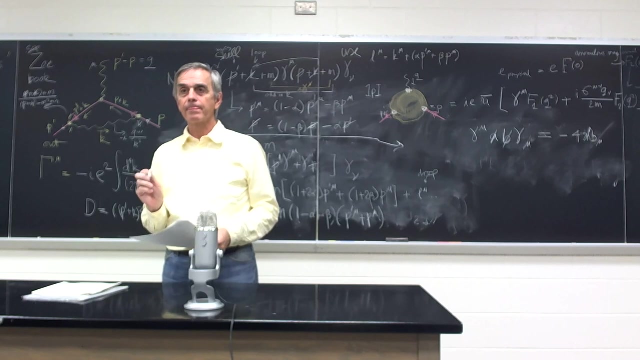 to achieve the origin. and what the identity does is when I replace: Let me just write it. I'm in deep waters right now. Let me just write it. I need to write and then go and discuss it. What did you ask? Why am I dropping L mu? 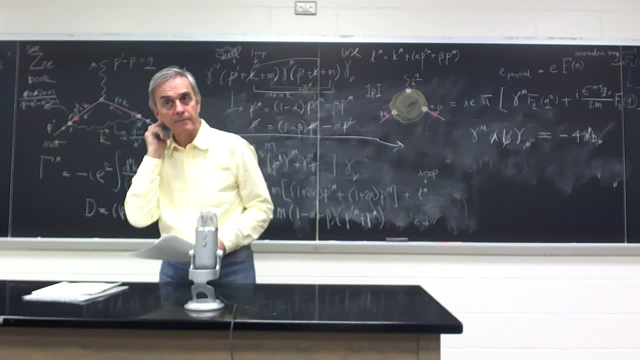 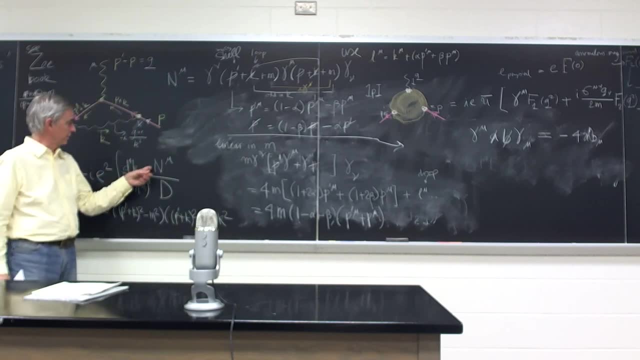 Why am I dropping which term L mu? Because if I have a term that's proportional to L mu, it's linear and integrated over all spaces. It's an odd function that's being integrated over all spaces. So you know anything that's proportional to K or L, to the first or third power. 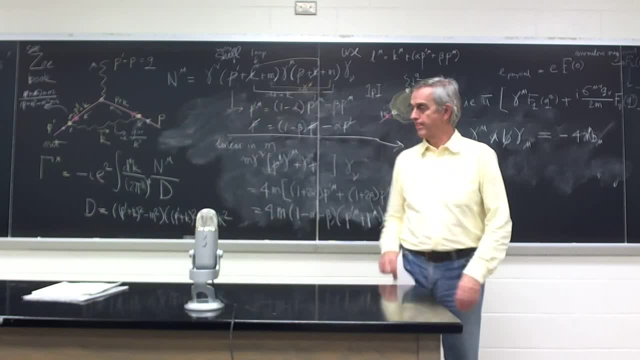 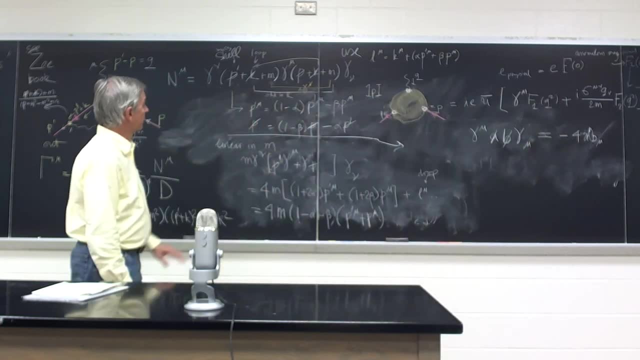 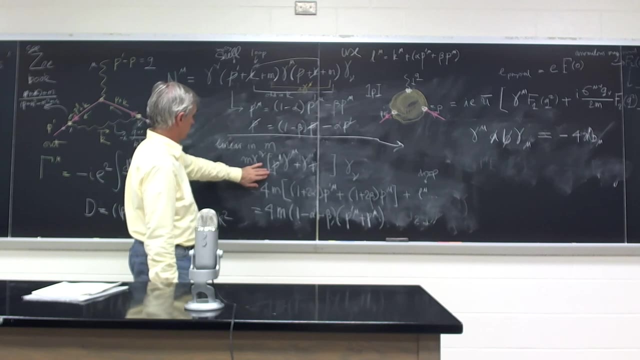 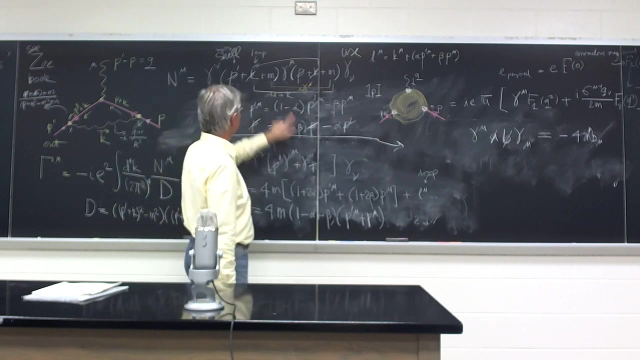 will drop out. I have to. So this is in the original integration. Oh Yeah, what I'm dropping is: There are also terms that look like P. right, This is also these terms: M times K. So every time I write this, there's also terms that have a K here. 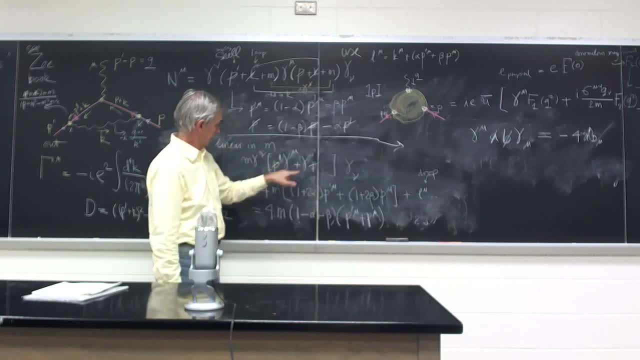 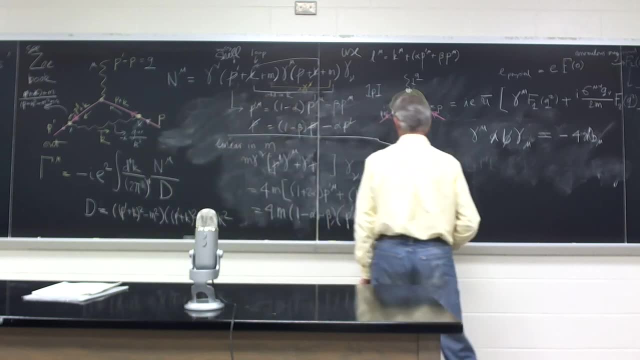 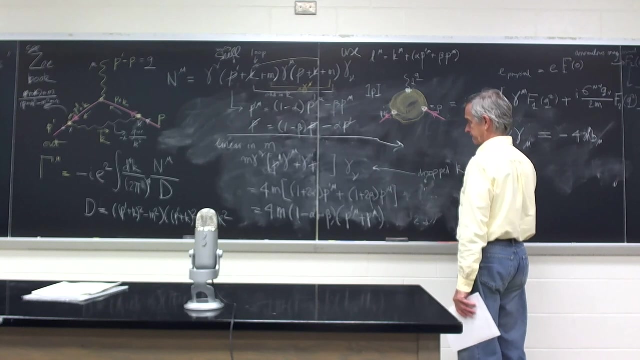 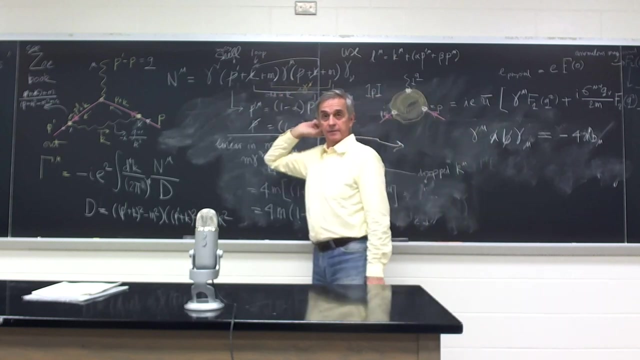 Or in change coordinates, it will give me a lambda, And that one is odd. So this is just odd. So maybe Let me say Before here, actually, Maybe it's easier to understand: Drop. You know, here I've dropped Terms proportional to K, It's a distance. 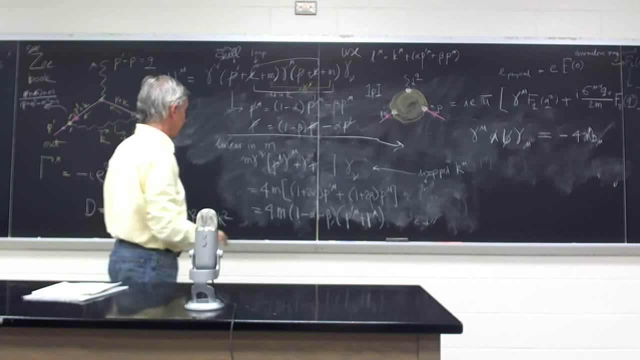 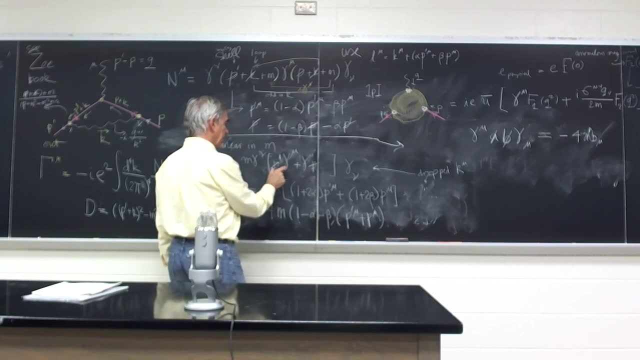 Now, one thing I can't remember is Why did I get a 2 here? So you know I'll pick up a 2 And I do an anti-commutator, Because I want to bring these guys together: P's and slashes, Mews. 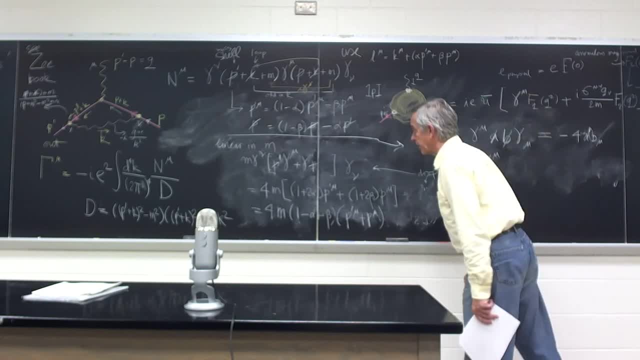 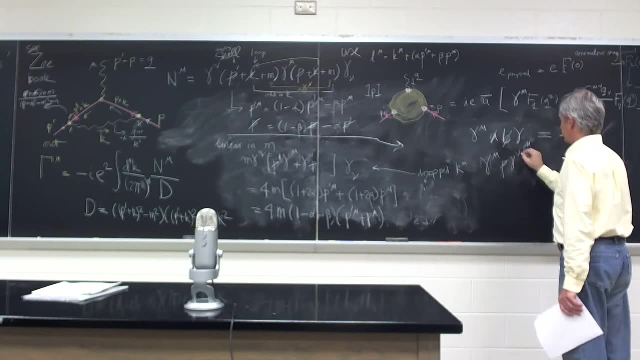 Let's look at all of these. So I have a P slash: Gamma Mews, Gamma. So that's That's first term. has this form Right? Alright? P Lambda, P lambda, Gamma Mews. Let me put it down here: Gamma Mews, Gamma, Gamma Lambda. 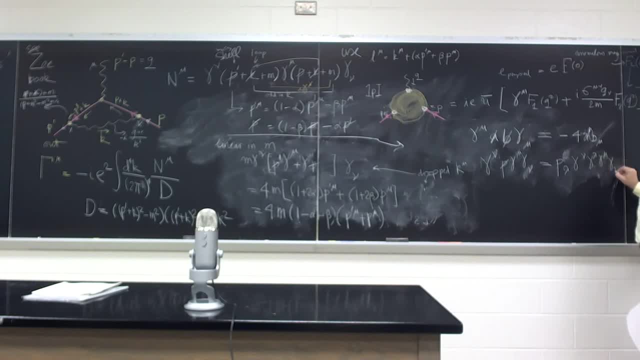 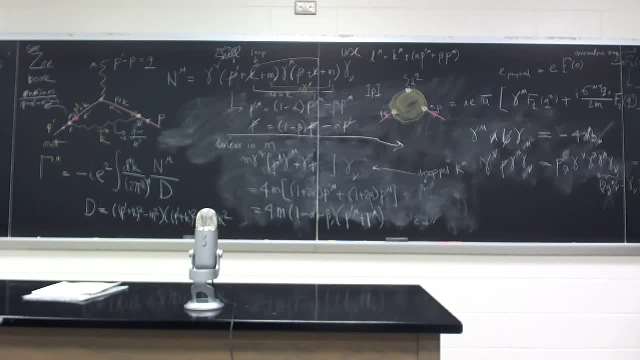 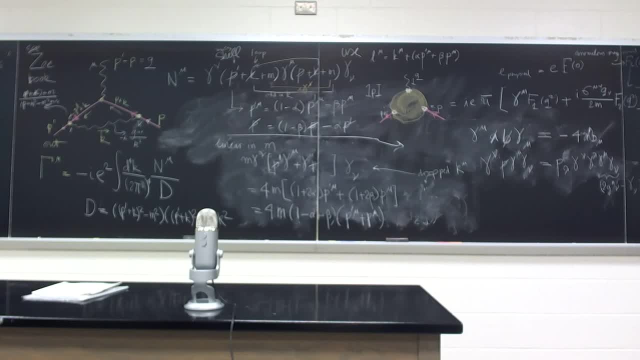 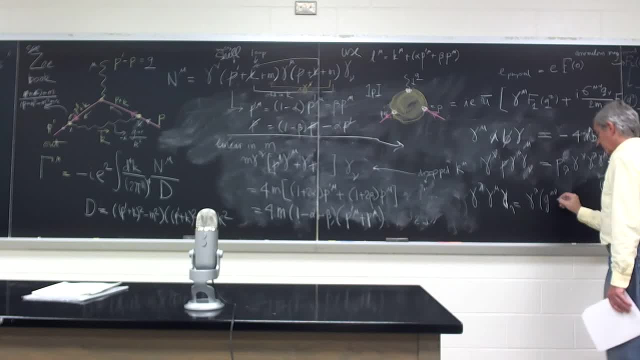 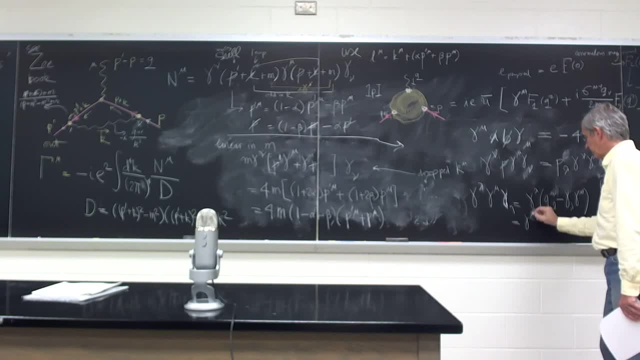 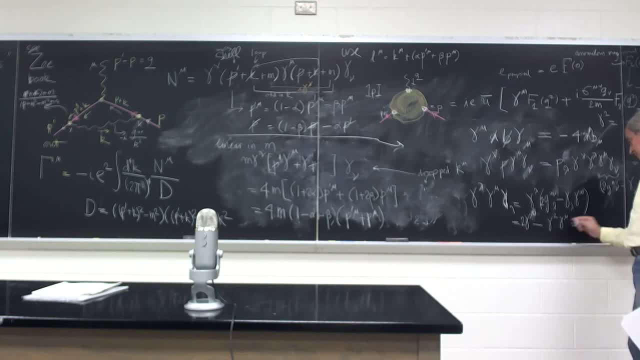 i mean, that was the first thing. that's how you introduce it, so i thought we introduced it to be one. uh, uh uh. so that's gamma mu looks to me wrong. but if this is one i subtract, am i wrong? hello, anybody there. i'm off the blood. it's embarrassing. 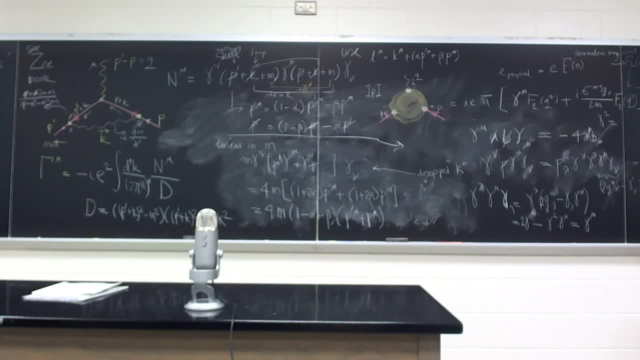 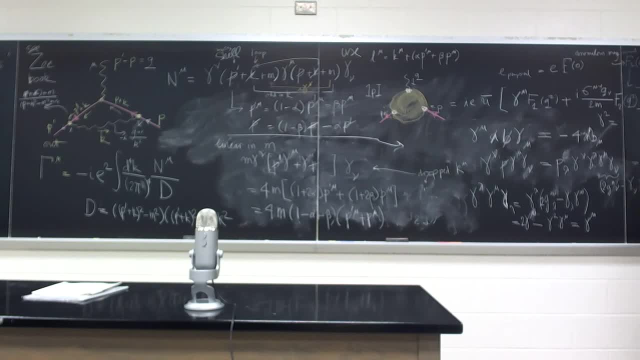 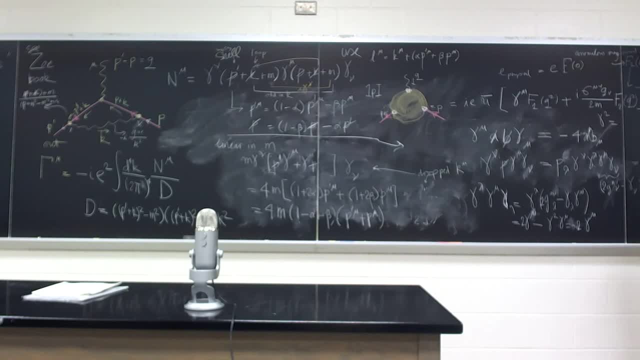 Anyway, so you do this stuff and you prove this identity, you stick it in there and so I think this 2 alpha came from. you know, this 2 bothers me a lot because there was 2 or 2 here and I hope it came from that identity. it dropped there, but there was. 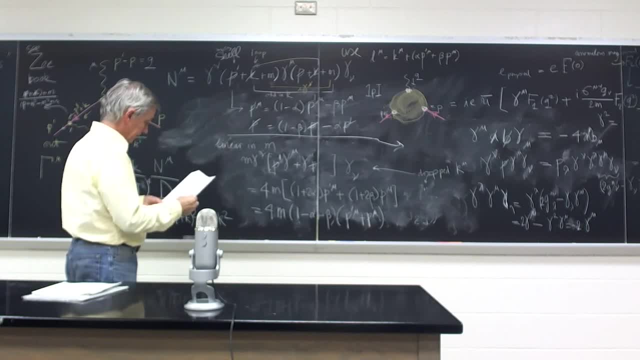 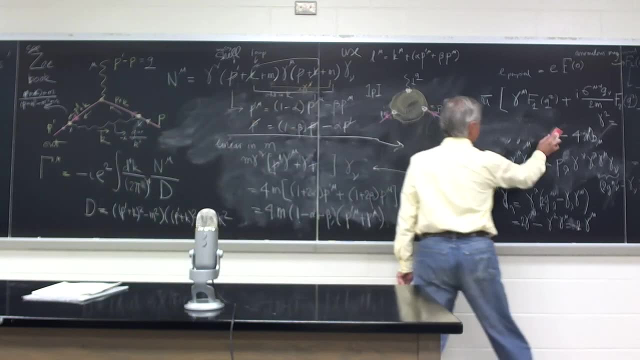 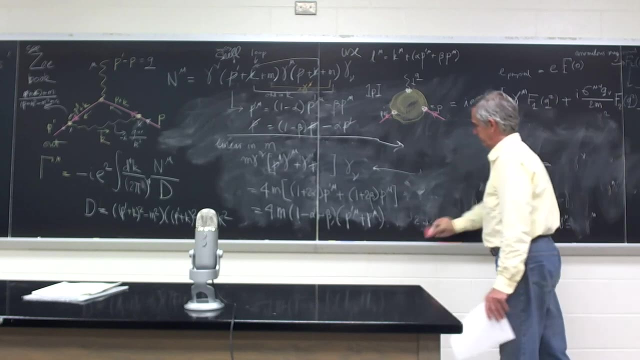 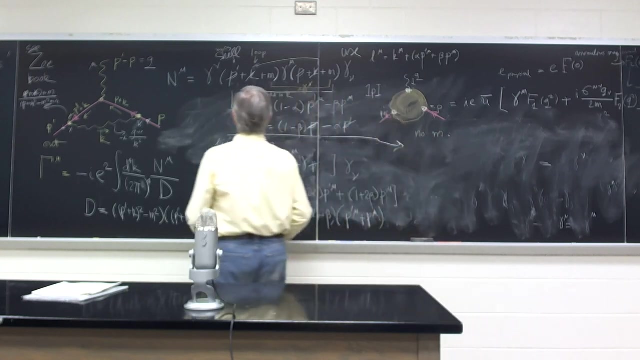 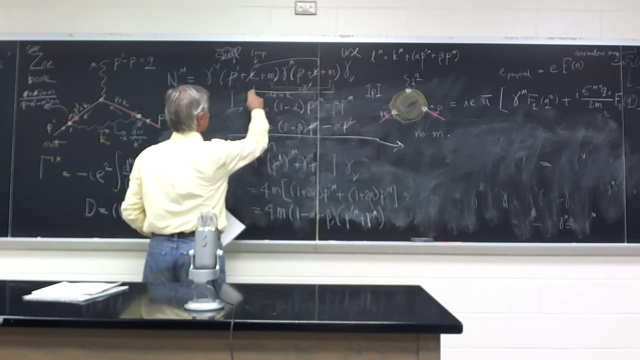 something here. So then there is finally a term that has no M in it. So that's a term where we are multiplying these parts together and we know that cross terms, where there is a K here and T there will vanish because they are odd by integration. 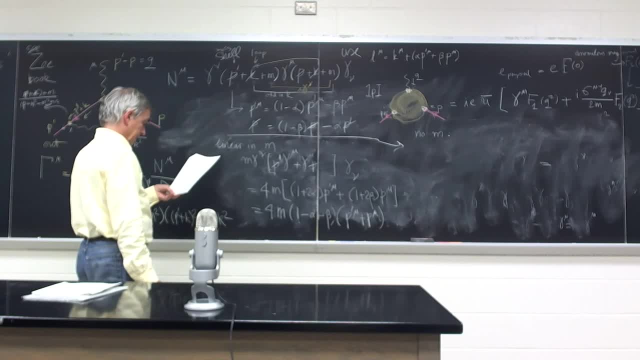 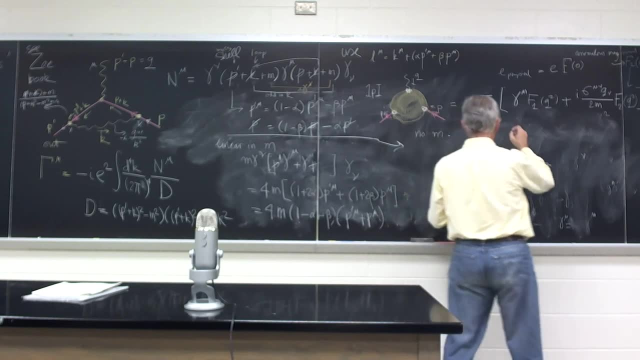 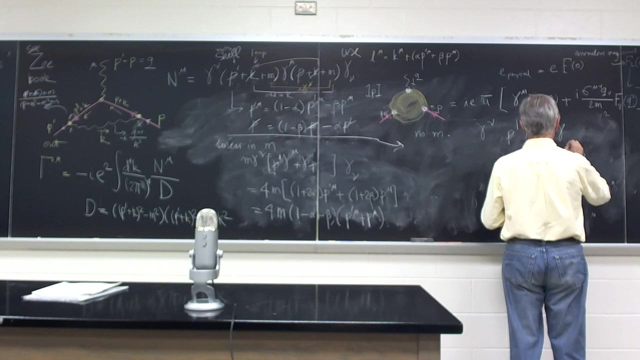 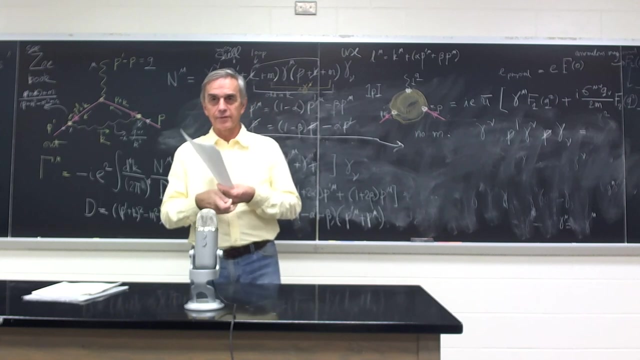 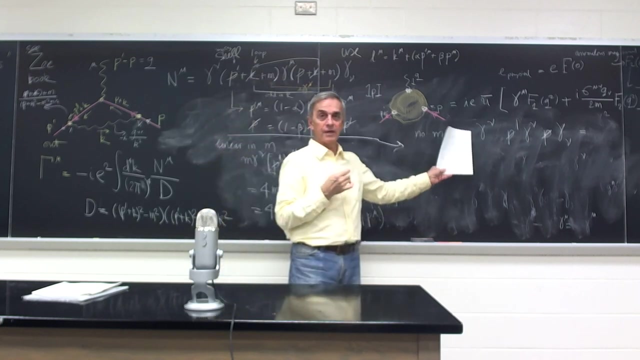 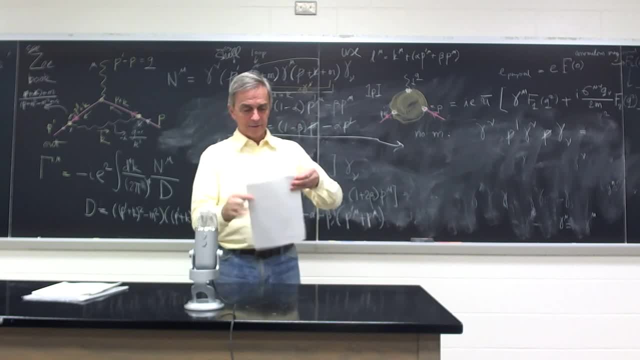 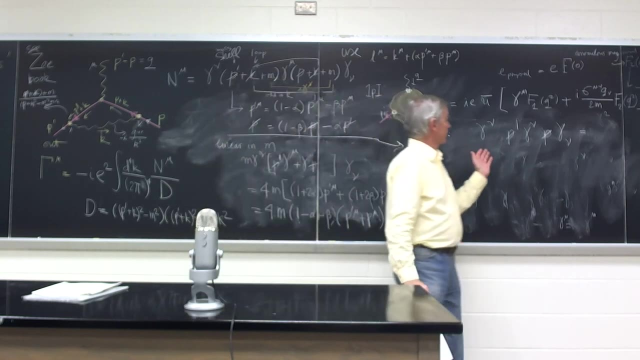 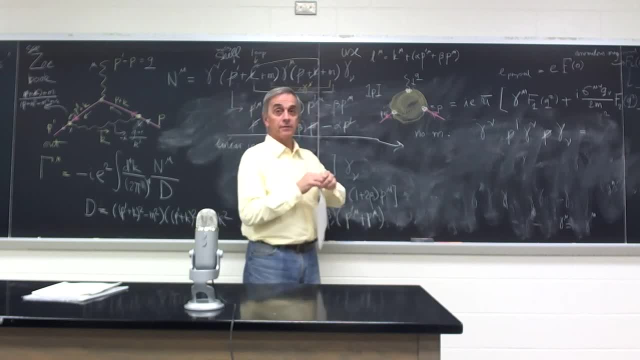 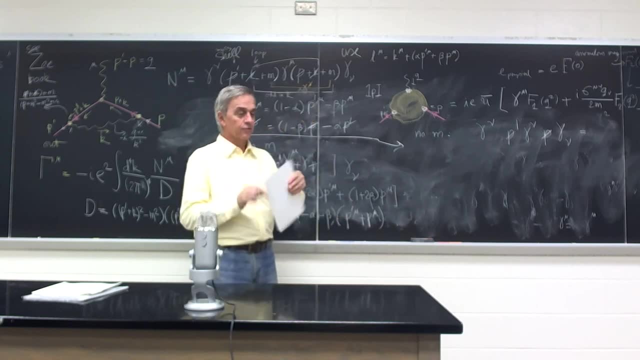 Brookhaven. I was in Cornell, but we had a synchrotron and at night they allowed me to edit my files. So I wrote an algebraic evaluation language in the editor. so whenever they checked what I was doing, I was just editing, I was running Tico editor, but actually I was doing very 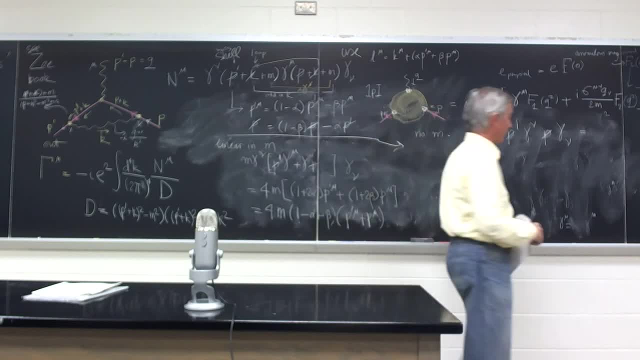 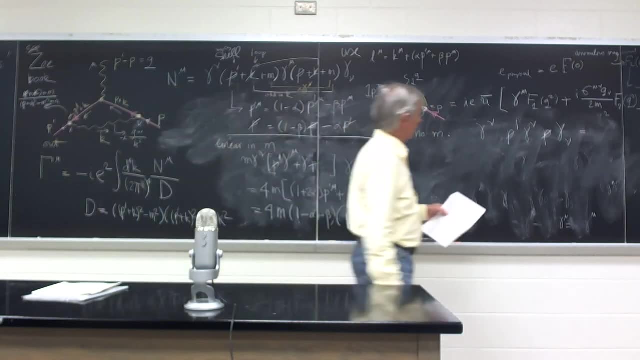 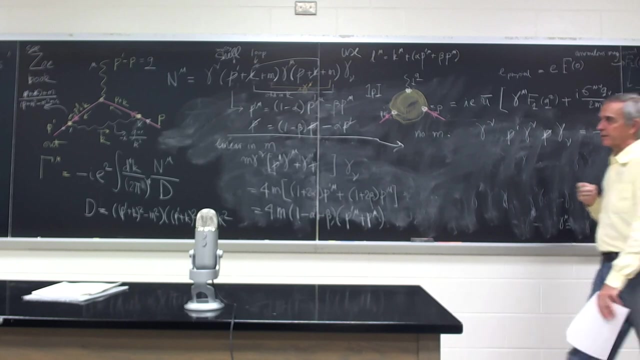 gruesome calculations, of which this is a trivial part, because you know, by the time you get to the three loops, you know these guys get endless and you have to evaluate them all. But here is the worst in this particular calculation. So you can move this through using anti-commutations and, by the way you know, this is where I 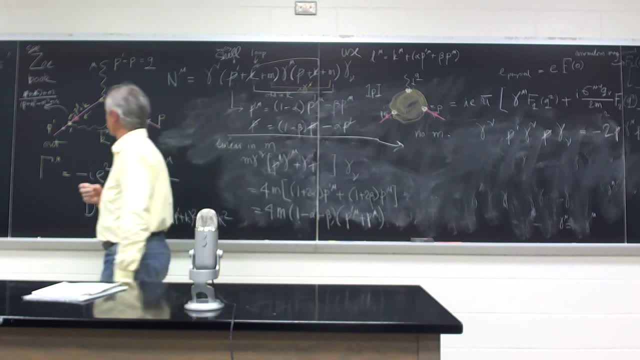 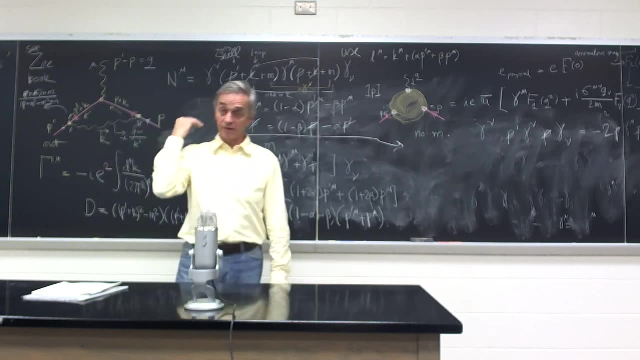 find the machine. it took them months to do this calculation because the Klein-Maschina formula was formulas simpler than this. but you're scattering off external thing. but it had lots of gamma matrices in it and they only knew that there were four by four matrices. 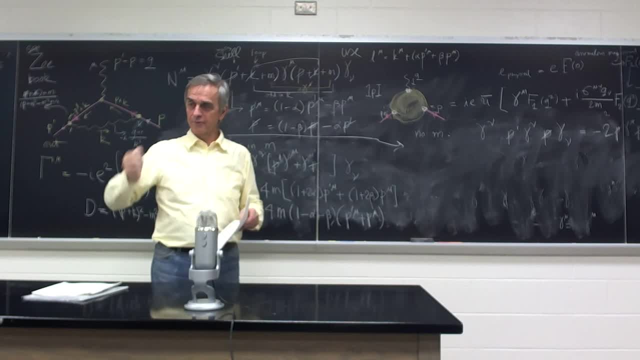 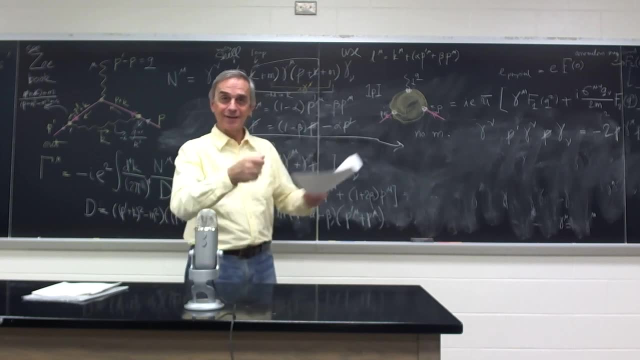 so they would multiply, every day, every morning they would multiply four by four matrices, and they had four of each, because it was sound, over there were Pauli matrices stuck in the way to the original. So the original, So the original. 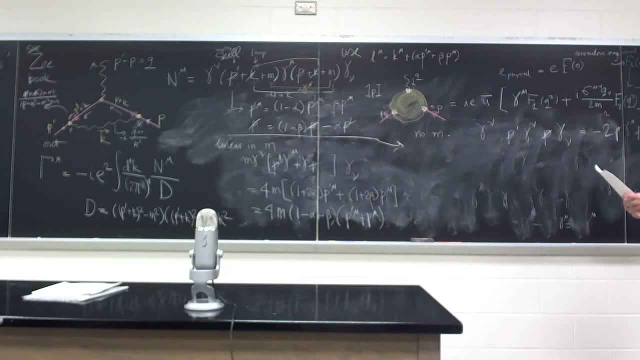 So the original calculation is just crazy, but you know, once you understand its algebra, it's very easy to optimize and the claim is that that's what this calculation is, And it's a little bit unfortunate. you notice that P and P prime have gotten interchanged. 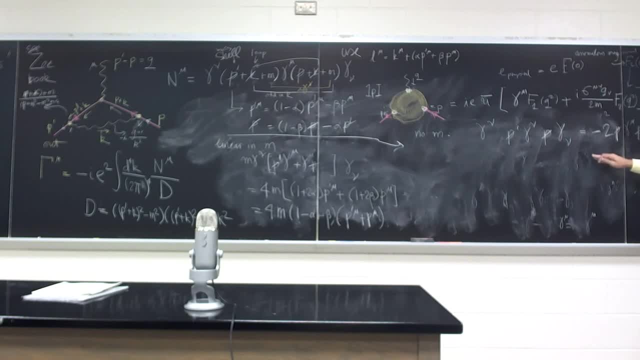 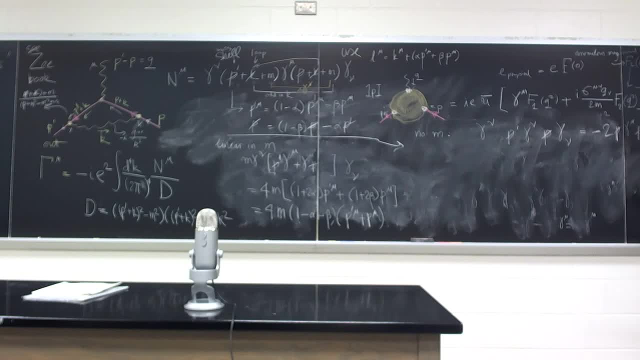 So it's called P prime, U bar of P prime. So this one which is gamma mu, which you can draw, What about the indices? You appear in mu and I can't see it. This one is in mu. 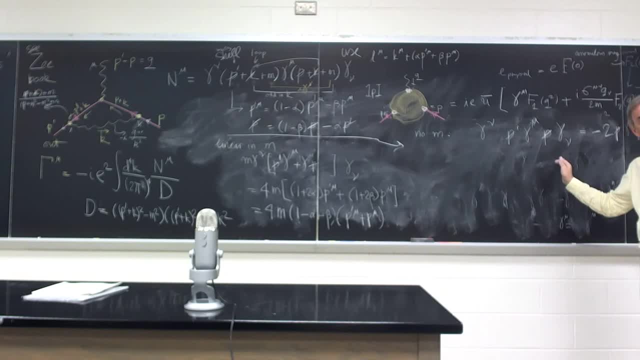 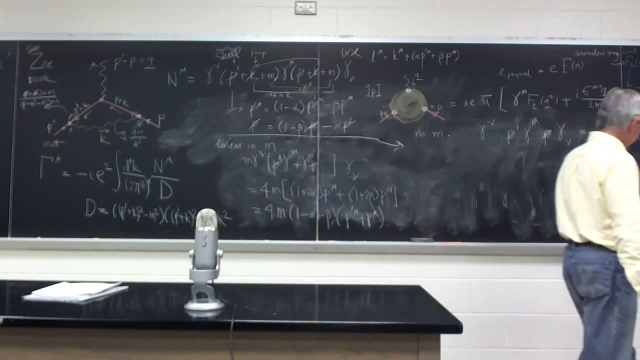 Again, you know, when I do these calculations I only draw pictures. So there is no confusion. But at this level it's not a question level. it's simple to do it within the system. So then you know you have to. 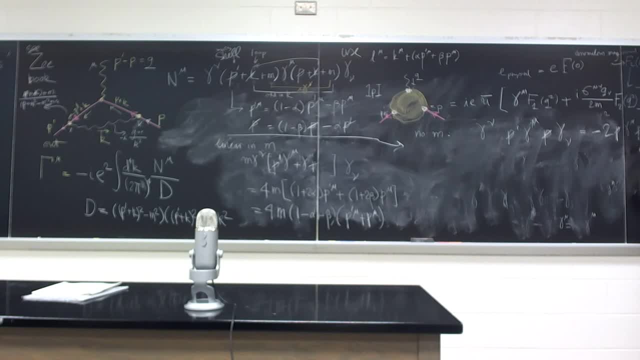 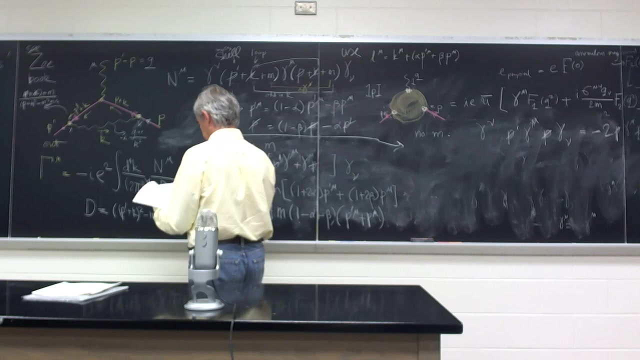 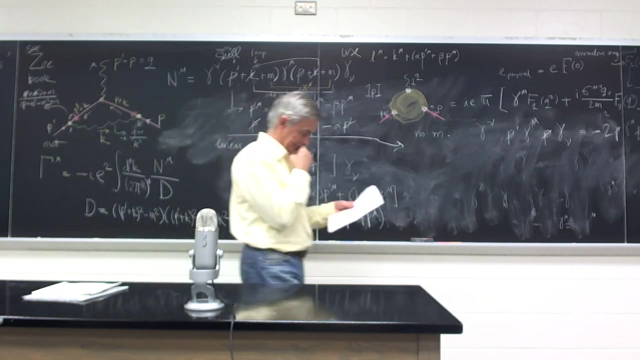 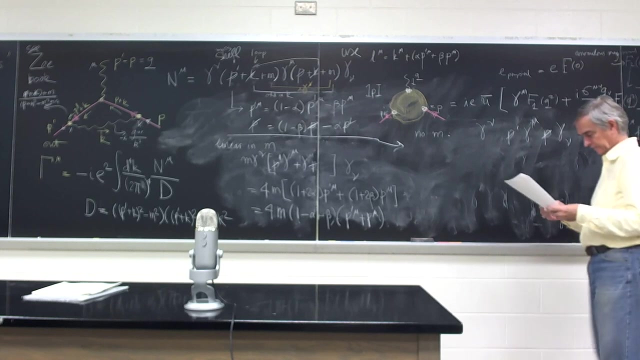 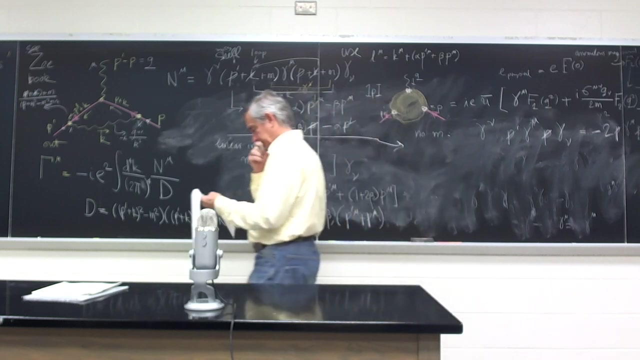 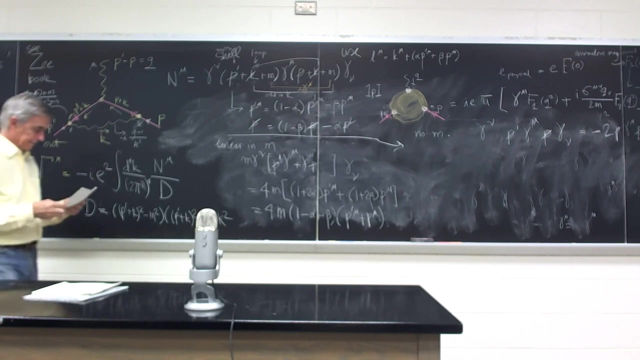 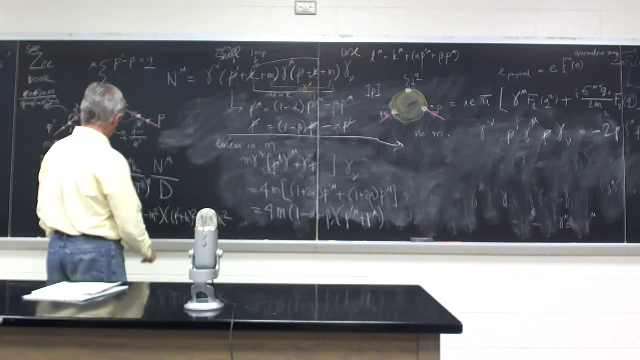 commute them back so you can use the mashup properly. And when this is all done, the claim is that I mean, I'm sorry, but the two problems, that I was scared through this madness and that after you have done that, after you have done all this stuff, 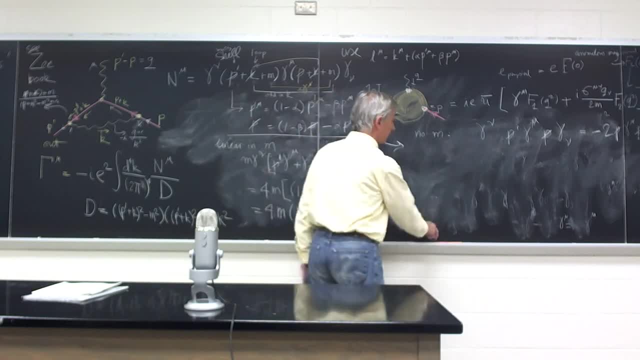 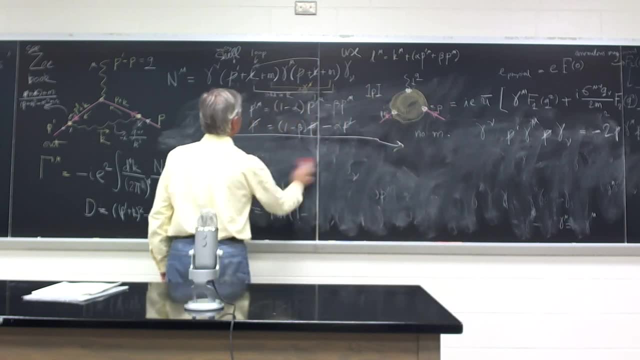 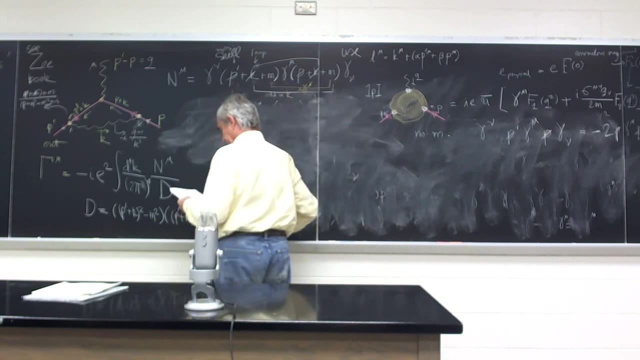 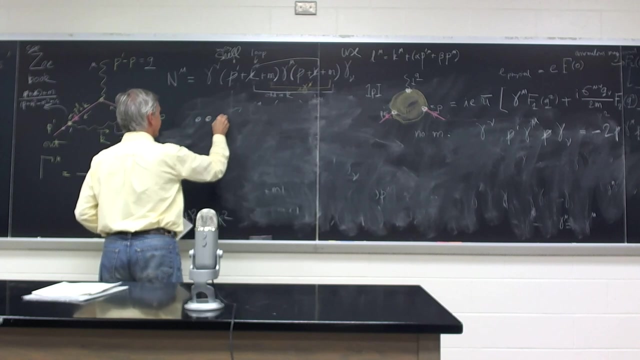 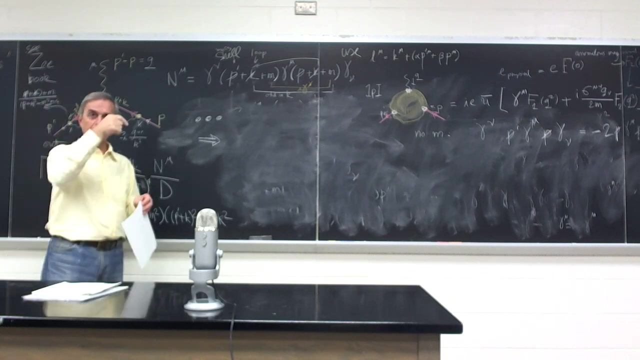 you finally have a part of the numerator that contributes to the magnetic moment. The next one is Dot dot, dot, And this is what you're allways doing, In high-re, presumably. there's a popular phrase that says blah, blah, blah. after some algebra we obtain blah, blah, blah. 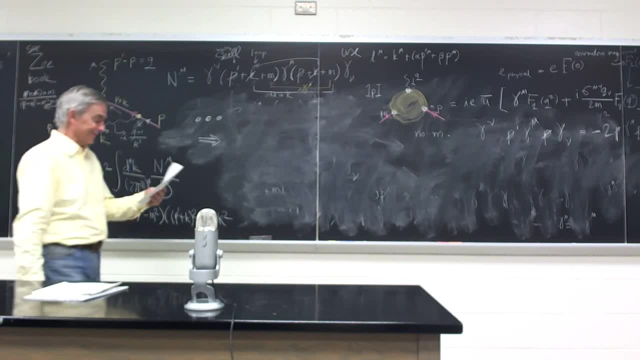 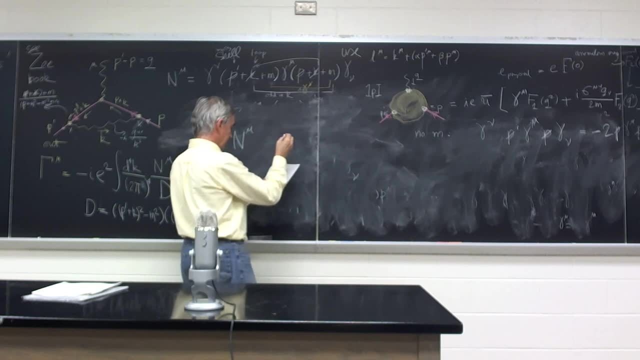 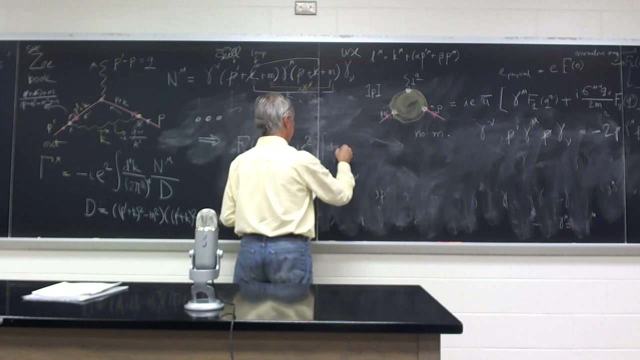 In high-re we obtain blah, blah, blah, And this after some algebra often turns out to be a month of algebra, but here it's only a few hours of algebra, which you can do yourself, And we get that formula for the magnetic anomaly. second form factor of zero, which is minus, i squared integral of g, alpha, d, beta. 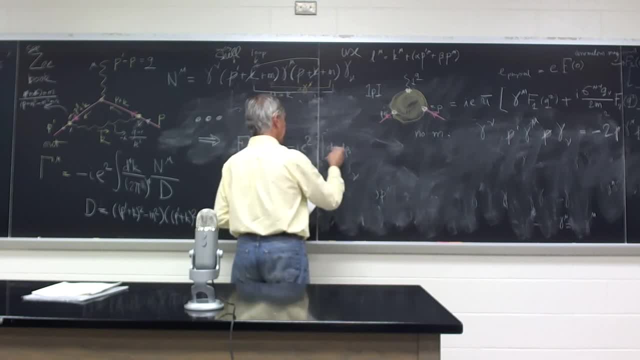 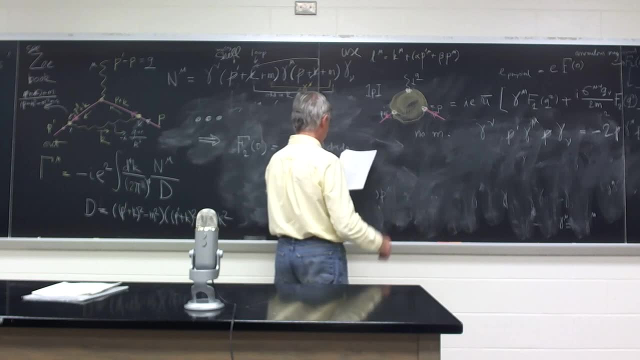 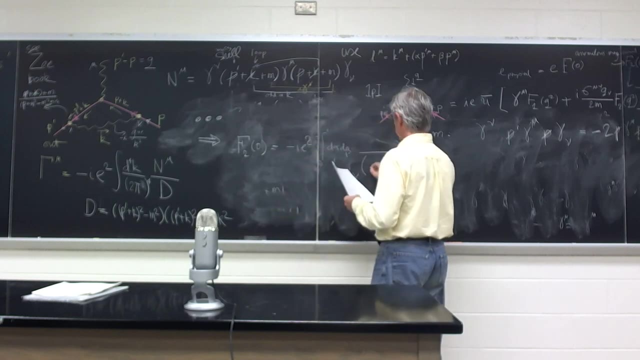 you know, from zero, So it's one, and then the sum of them has to be one or it's less than one, And we have a very simple numerator which is four momentum square. I still haven't integrated the momentum to this. 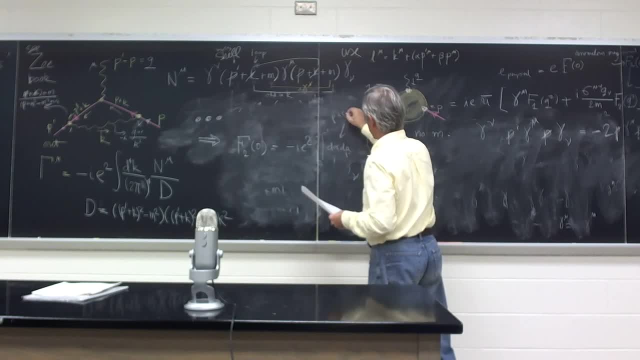 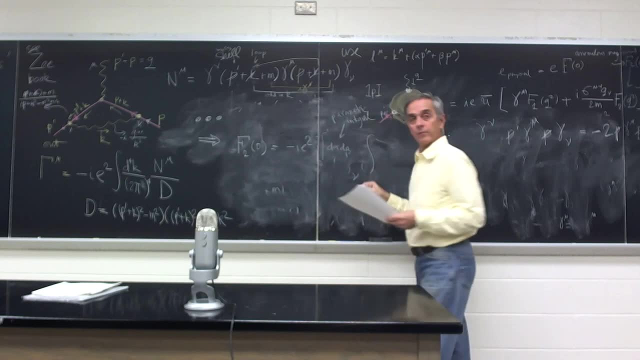 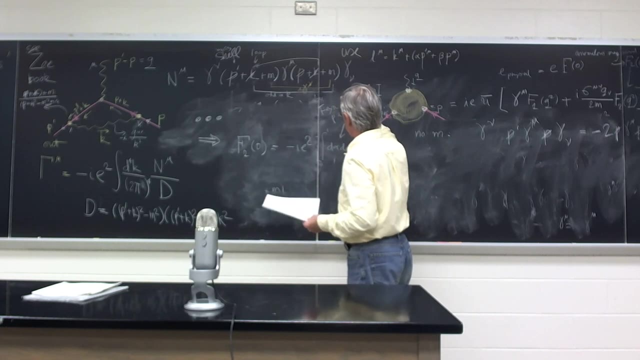 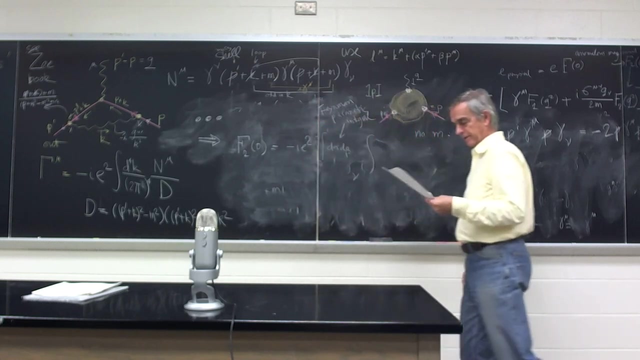 This is called parametric, It's a symmetric integral. What did you say? Yeah, so this one is called Feynman. I prefer Schwinger, but you know the Laplace transforms, which are the better thing. But if you listen to a bit and explain the Schwinger representation, it's more insightful. 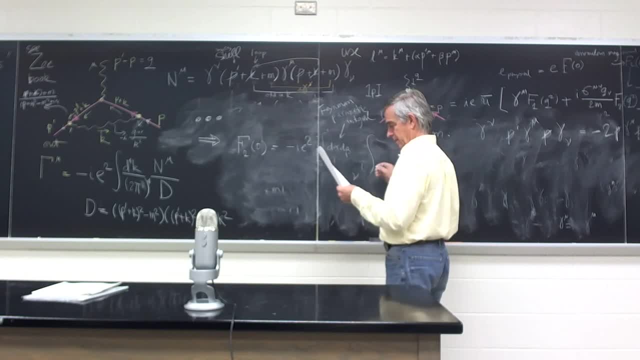 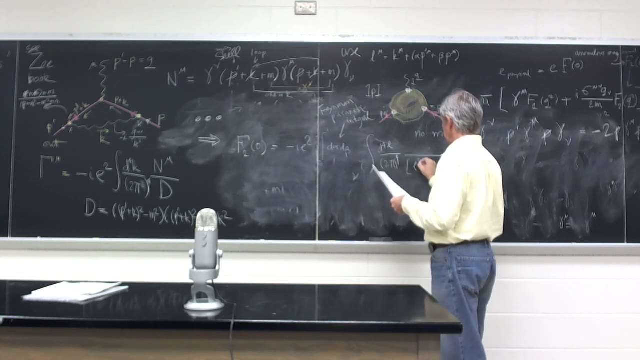 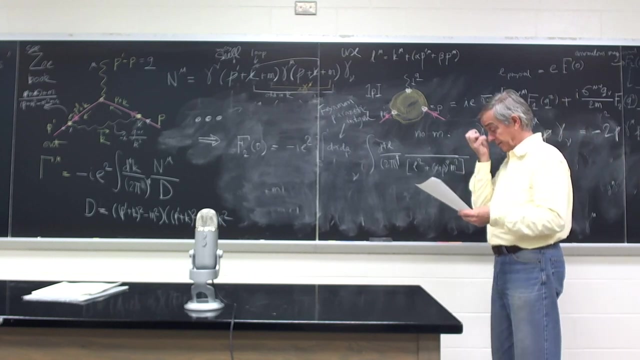 It puts some physics in there. The link is on the web page. So the numerator is just quadratic in the four momentum. And this integral is another reason Integrals are like this. There's another reason why, Okay Well, Wolfram decided to develop the language because he wanted to get rid of – the way 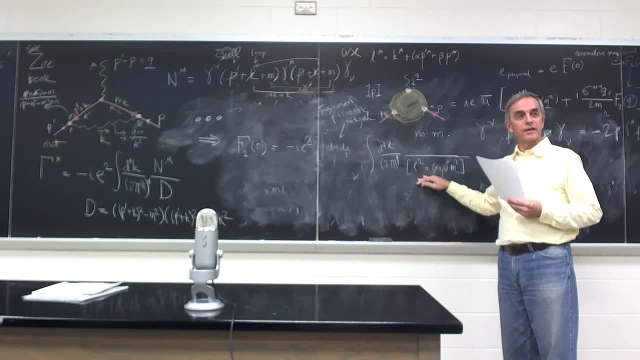 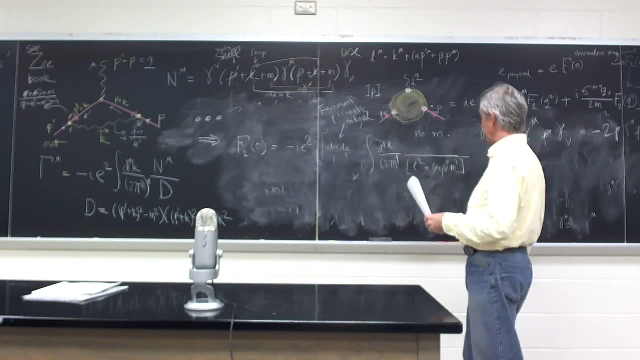 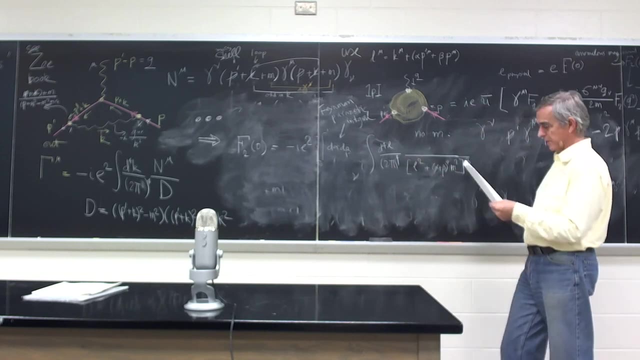 we do this. integral is we look up at Gratstein and Riesling tables in the old days. But he wanted to compute it to do the lookup. So that's where Mathematica, originally Maxima, came from. So to the cube. So that was an amazing simplification downstairs. 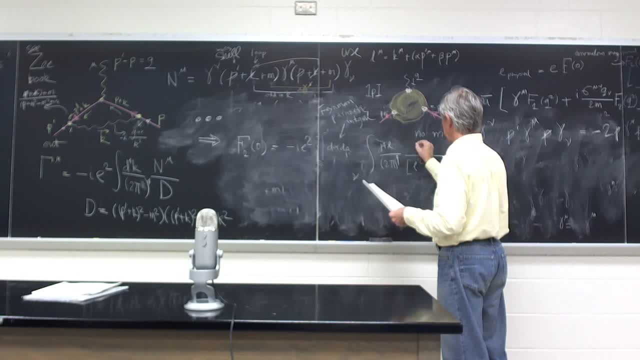 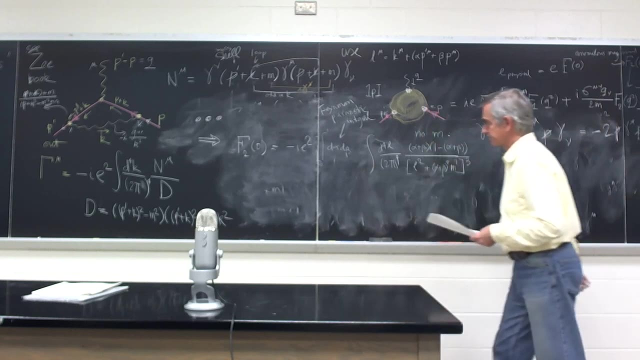 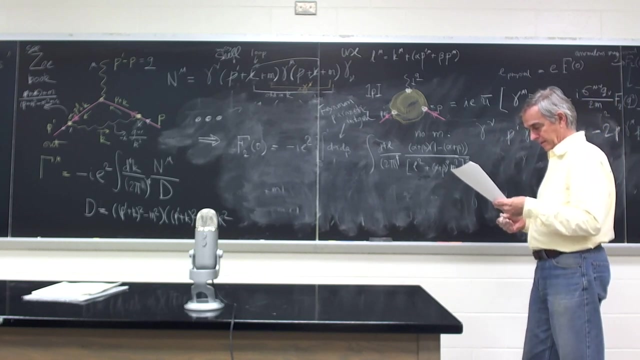 And upstairs turns out also pretty amazing. You can get alpha plus beta, R minus alpha plus beta And that's the integral for the form factor. after you do all the algebra, Now the momentum thing, you sort of know how to do because this looks like the radius. 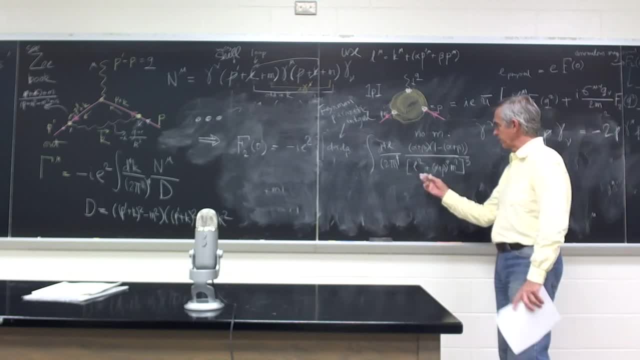 It's not the radius, It's the integral, It's the integral, It's the integral And it's not the radius of something. So integral is the volume of some sphere because it's radially invariant. So it becomes a one-dimensional integral in the – this radius and multiplied by 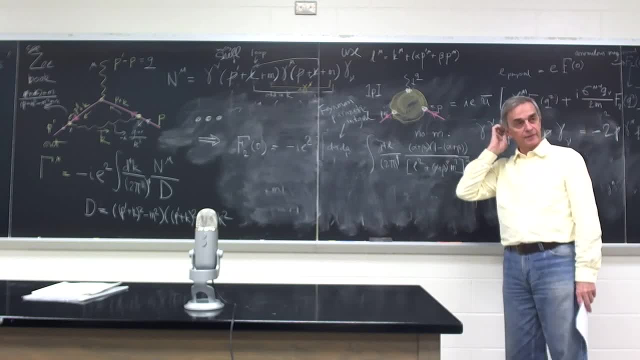 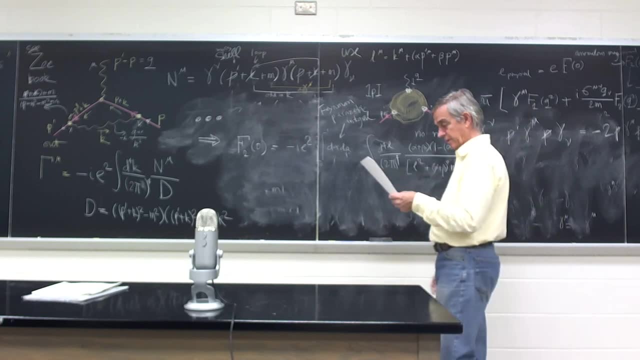 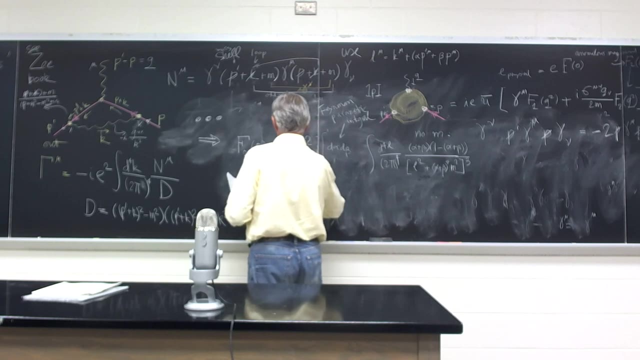 you know some combination of pi's that give you the volume of a sphere and gamma functions which don't look like anything much, So that once you do that integral it turns out that integral here looks very special If you know how to do this integral for every Feynman diagram. 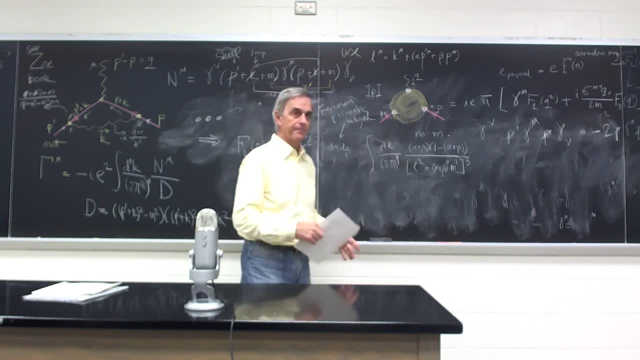 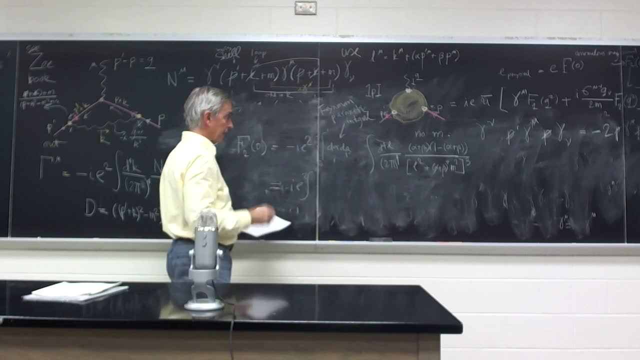 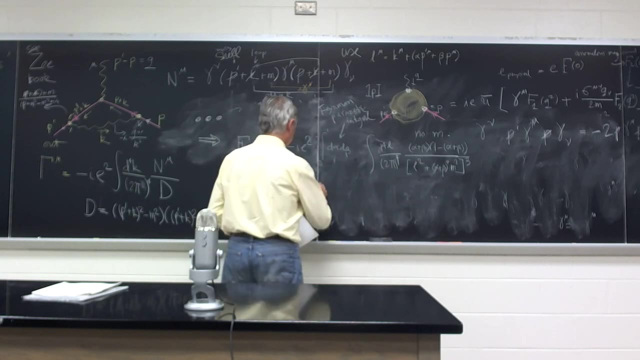 you know how to rewrite every Feynman diagram in parametric form, So there's a beautiful theory of how to do it. You know graph theory of the same kind that's used in electrical engineering, actually, And computer science. Then you end up with this two-dimensional integral. 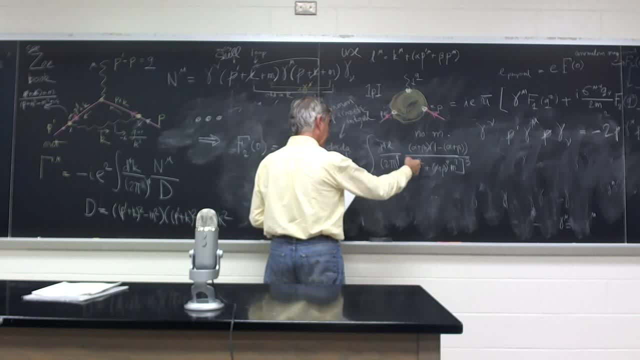 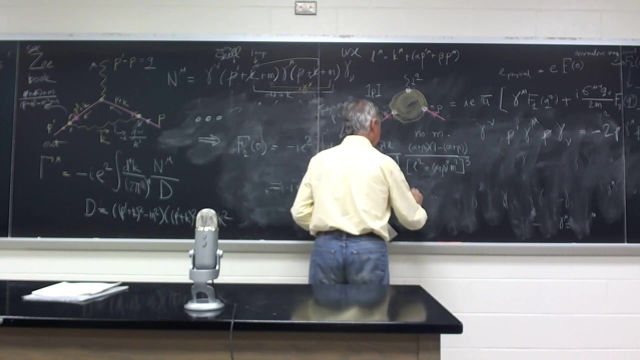 And this thing here gives you minus i integrating this. So there's a two i squared alpha plus Okay Times, the numerator that you already have And you know that this is a cube square and square One minus alpha is this: 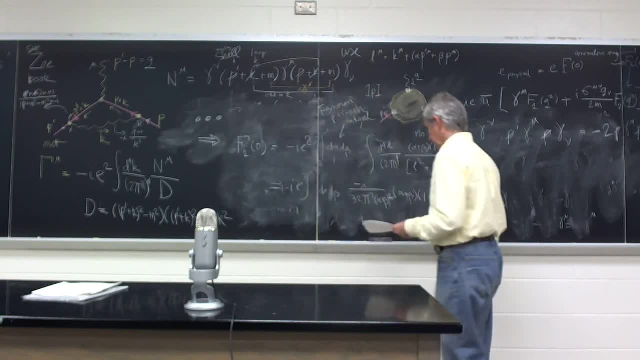 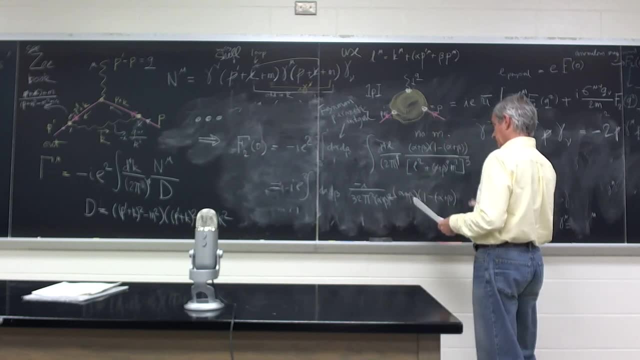 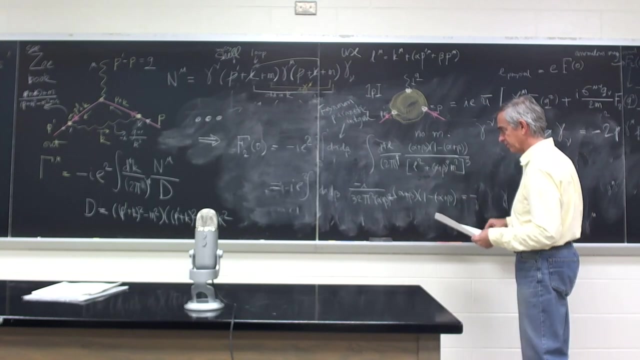 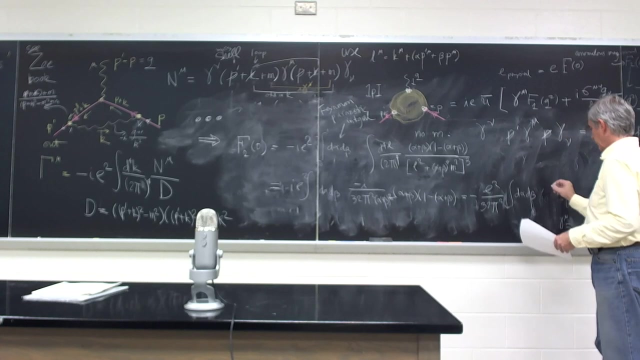 And then there's a consolation And you get minus on these two. i's Except. it's a very important sign, and I'm not sure why it's not plus or minus, But let's say it's, And this is the integral. 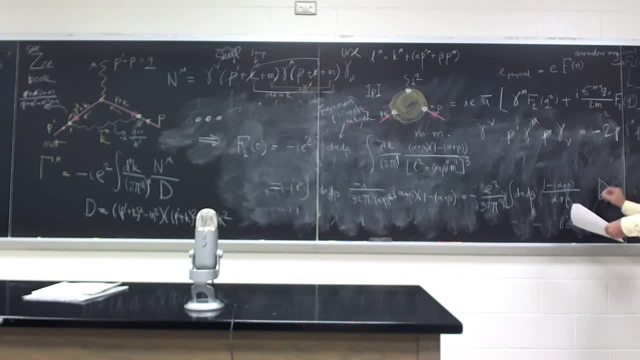 Let's say it was a. So that's it, And you'll see a zero. And then you know this is integrated in alpha beta planes. It's integrated over a triangle. So this is 1, zero. This is alpha beta theta. 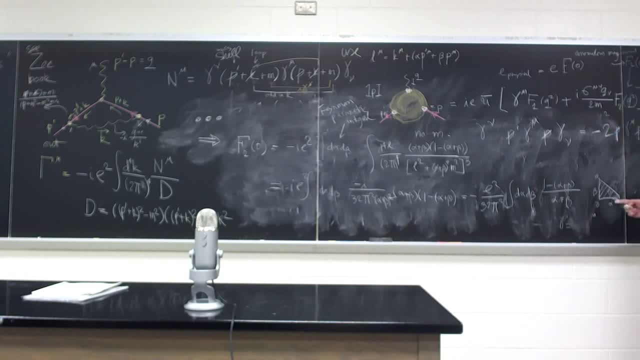 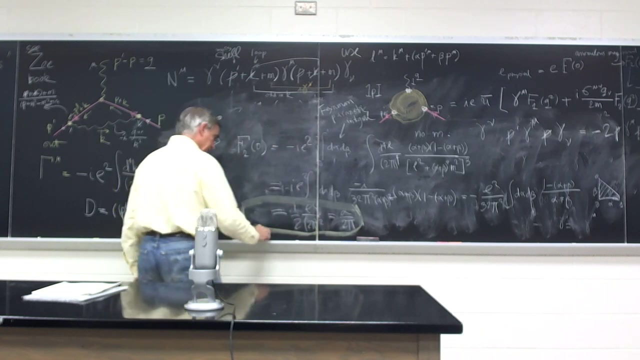 So if you first integrate these- that's the integral in alpha- you allow us to take any value, but then beta is limited to the vertical part And this becomes one each square. And this is the Schrodinger correction. It was reported as half a page of physical review, basically stating that's the answer. 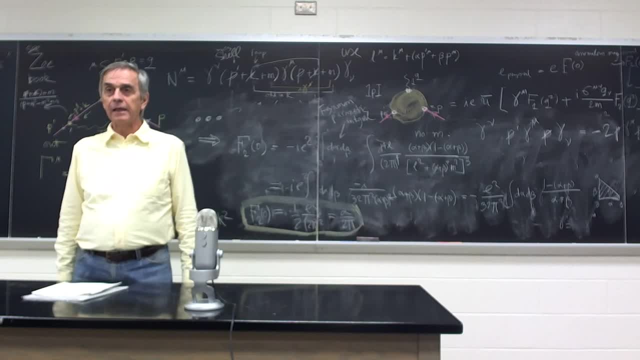 And you will, you know, get all the signs right in the exercise. But that outlines the calculation. You have to do some gamma mu gymnastics. You have to throw everything that doesn't contribute to sigma mu into this new term in your calculations. 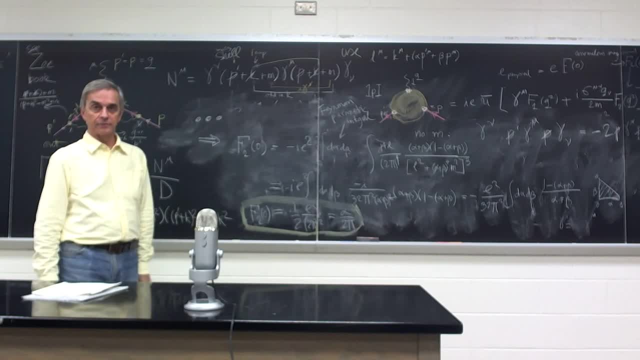 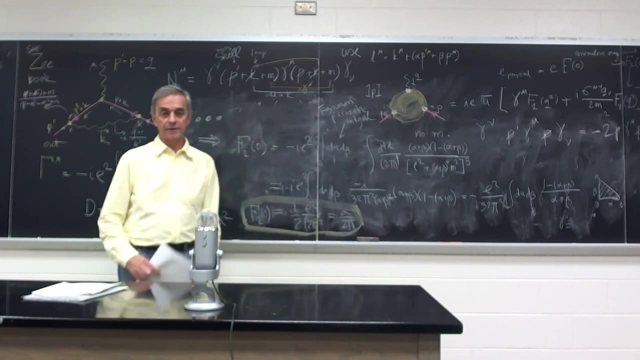 You know you go to parametric representation. As far as I know, this is the best way of doing this integral. I don't know of better alternatives. And the result is very simple, because you know this combination is called alpha, fine structure constant. 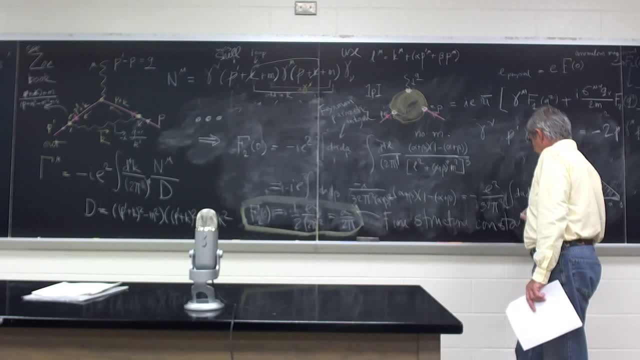 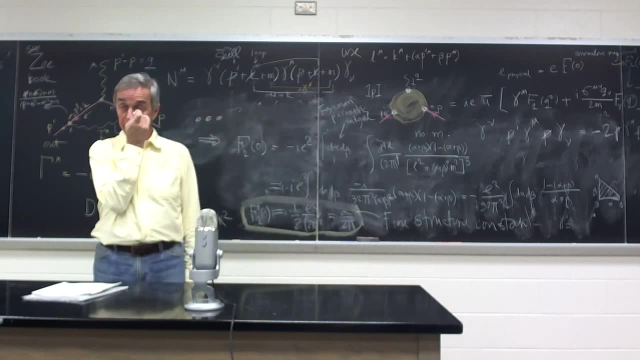 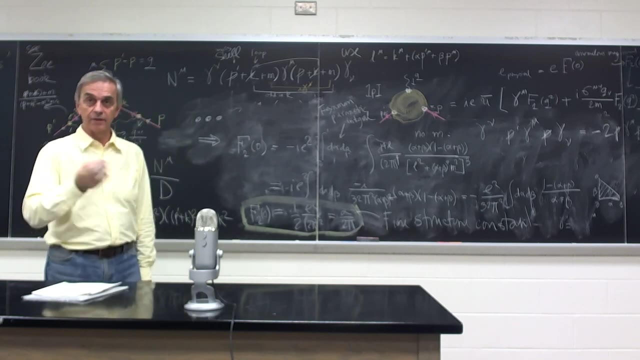 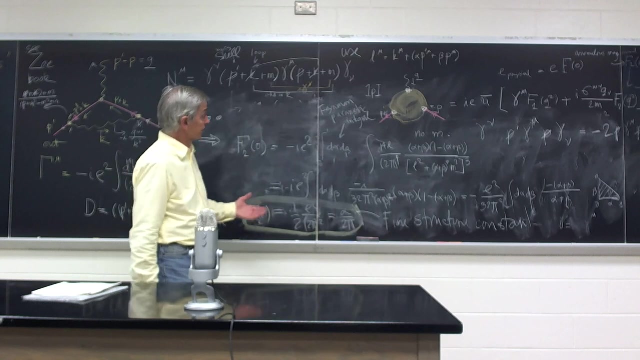 Then Schrodinger was very pleased because this explained the current experimental measurement in 1948.. So that was the first trial for real quantum field theory And it's a perturbation. So then you should be computing also terms that look like that. 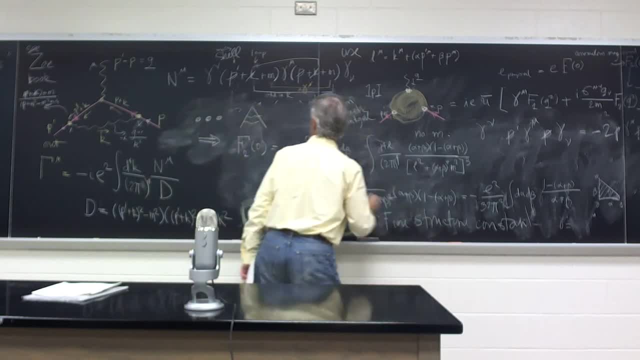 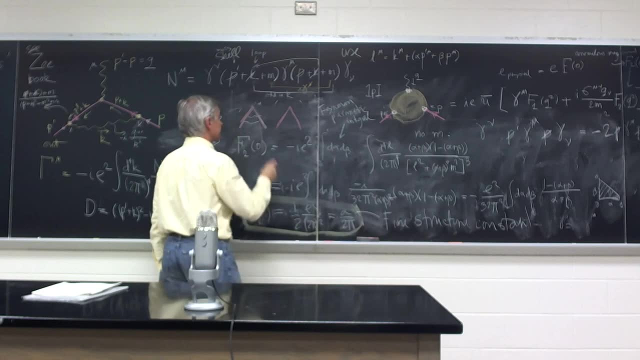 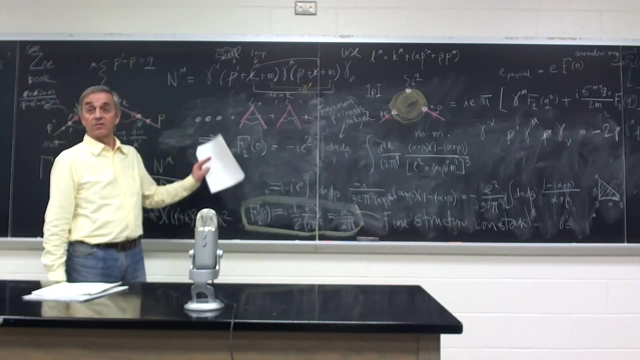 In order. there's a bunch of diagrams- Not very many, It looks like that- And the first calculation was actually wrong. So you know, first people computed it, made some errors, So it had to be fixed. You never read Schrodinger's. 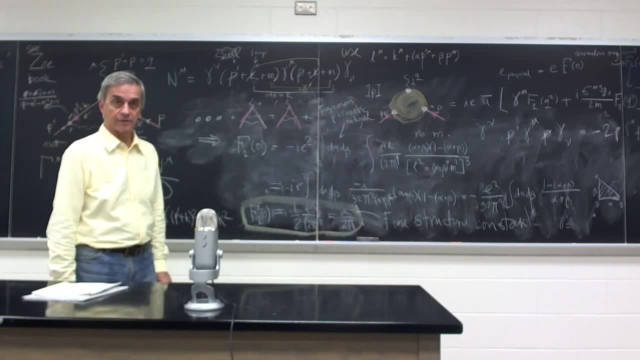 Schrodinger has written two books called Fields and Sources, And in the second book he actually does it analytically. It's totally amazing. He does a two-loop. you know this calculation that they screwed up for you in the first loop. he does analytically there. 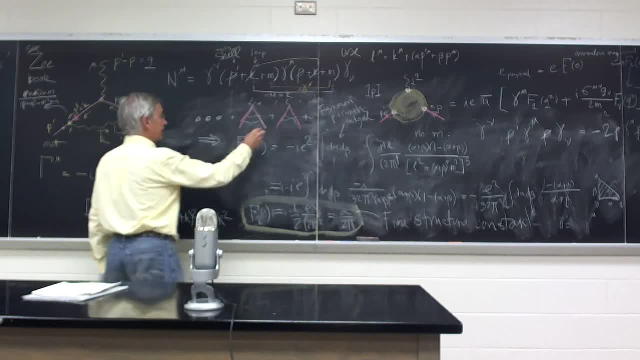 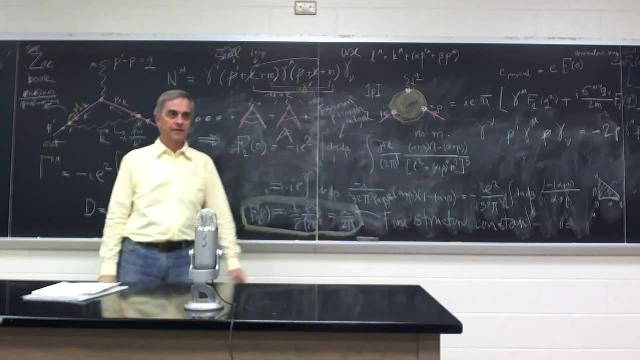 And today, by the time you get to three of these guys, it gets really complicated. So you know, there are 712 basic diagrams. No, that's nothing. That's beginning of the story, Because each one of them is hundreds of terms, et cetera. 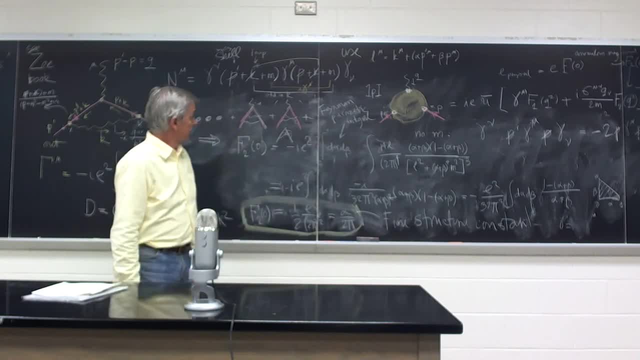 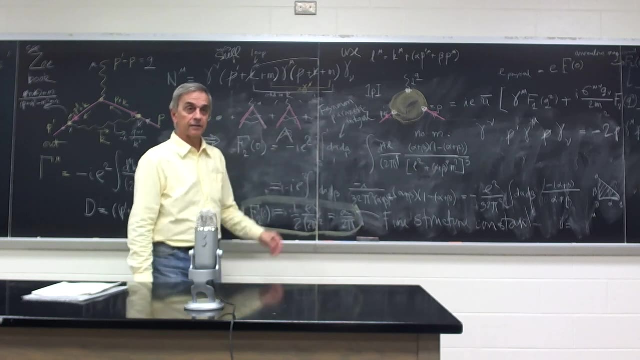 So you're working these few thousand diagrams. People have pushed it now They have completed. the amazing advisor of mine And this collaborator has completed four-loop correction. That took, you know, maybe a decade to do. Maybe I'm not being fair. 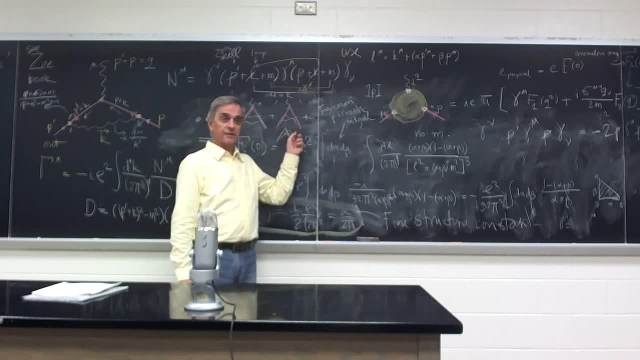 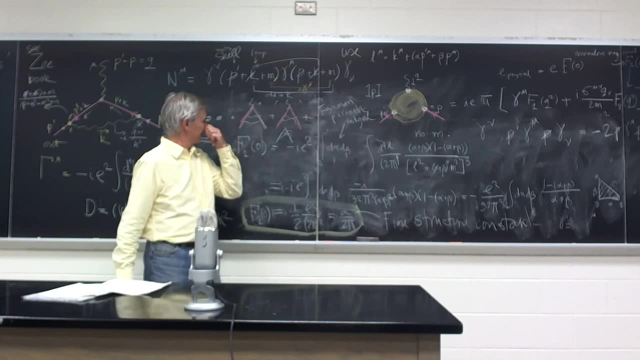 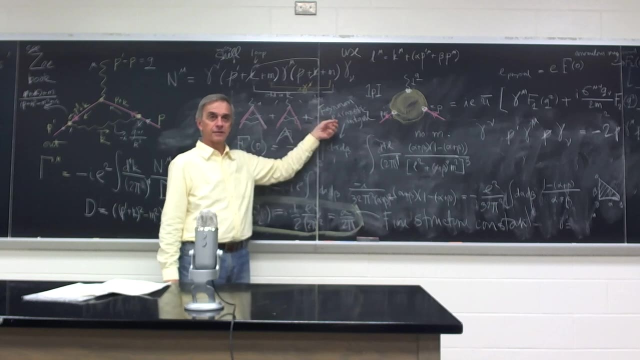 And much of the fifth order is also five loops. So five loops is computed, Not all of it, but much of it. And what happened to us? you know, while I was doing my calculation the experiment came in. It was three orders of magnitude better than the result we had by that time. 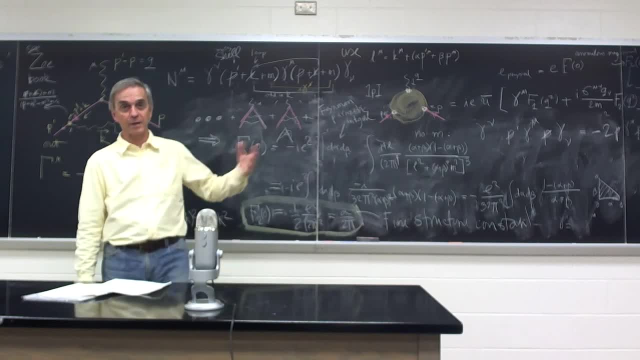 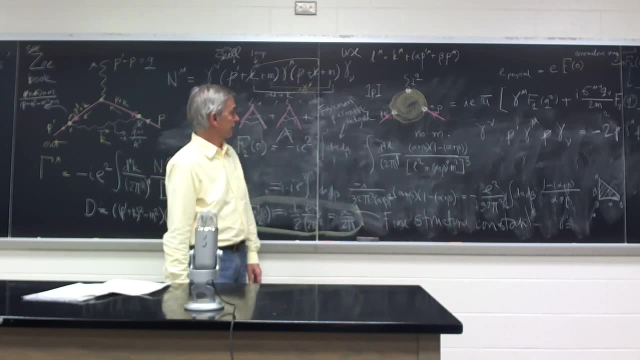 So theorists had to compute these corrections because experiments are so amazing. So I think it's one of the best, you know, finest things that's measured in nature. They select a magnetic moment, You know. one possibility is that, if you believe in quantum electrodynamics- 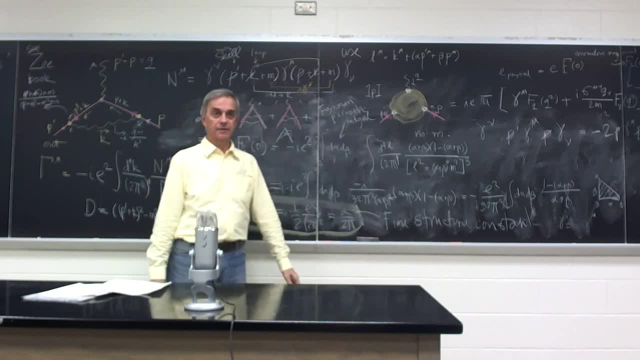 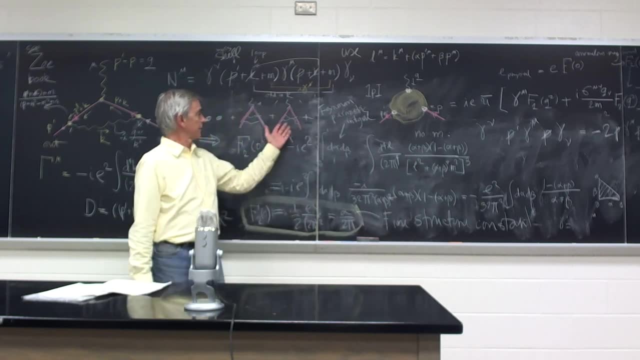 you might use it as a standard for alpha for charge, And that's not obvious, Because by the time you get to this higher order corrections, you start completing this polarization of photon into hadrons. So it turns out the way that higher order corrections are computed. 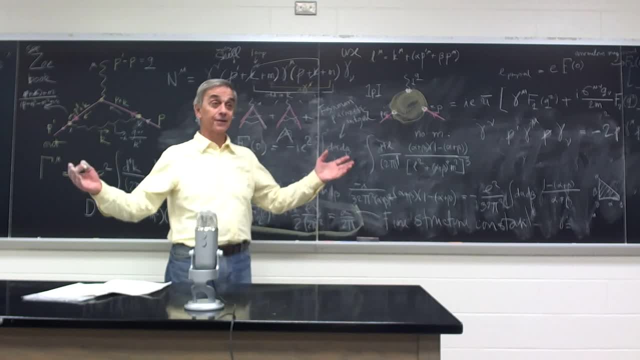 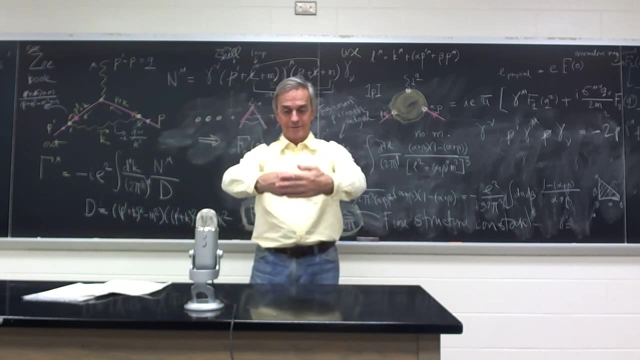 is that there's contribution that's measured by a lack, you know. So you measure at very high energy, You measure photon-photon collisions And that goes by dispersion relations into calculation of magnetic moments. So you know this totally crazy thing, you know.